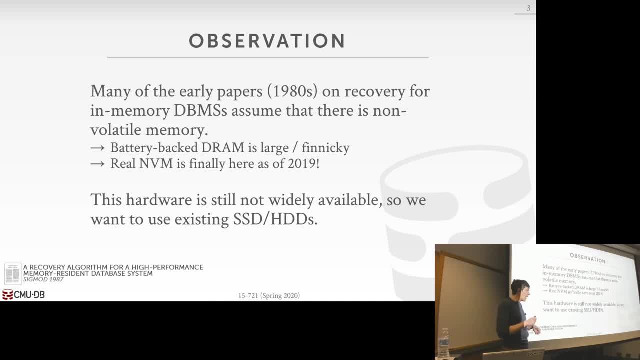 The paper I had you guys read was not in an in-memory database and I'll explain why I signed it. The there's actually not a lot, not many papers about about in-memory database log recovery When you look back at the early ones from the 1980s. 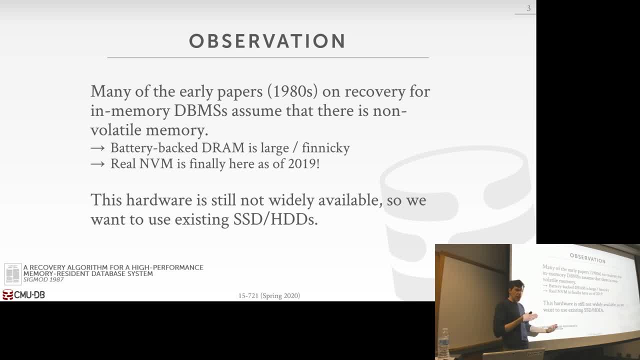 they all make this big assumption that the log or the database itself will be backed by what is called non-volatile memory or or persistent memory. Back in the 1980s this just meant battery backed up DRAM. So you had a little battery on the motherboard that could be triggered any time you. 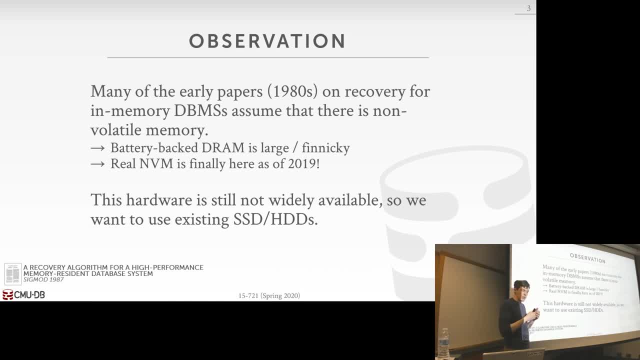 recognized that the power was gonna go down and you used the battery to actually graciously shut down the memory, read it out, the disk, And so when you came back, all your contents of DRAM were still there. So battery backed up DRAM has been around for a long time. It's not widely used because it takes. 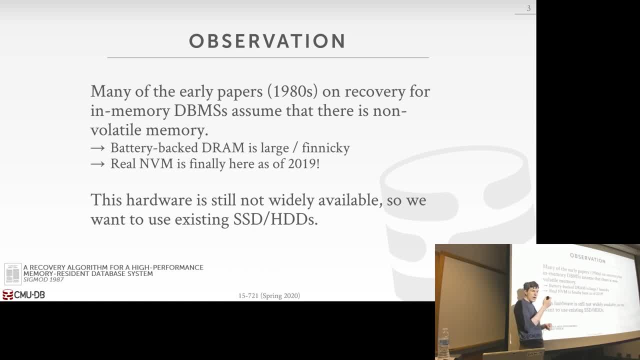 up space on the motherboard, right They? they're great, until you try to use them and they don't work right, Because you have to make sure the battery is always functioning correctly So you don't see that too often in the wild. You certainly can't go to Amazon and get an AWS instance that has 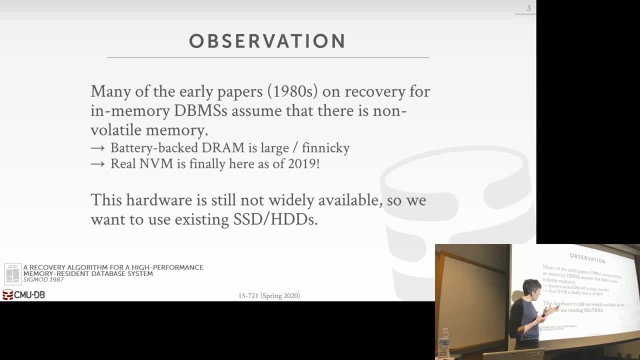 has this. So the other kind of persistent memory, though instead of being battery backed up DRAM, is to use what is called true non-volatile memory or true persistent memory. And so, for years and years and years, every time I taught this class, I would say, Oh, no, real non-volatile memory. 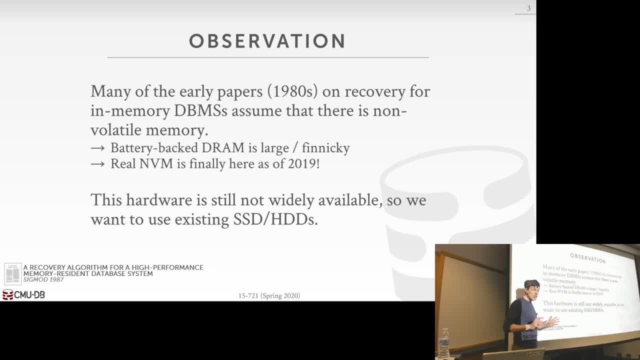 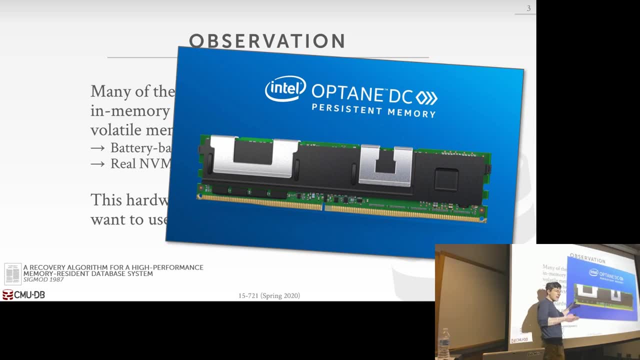 is coming out 1 year from now. 1 year from now. And finally, last year Intel stepped up and released true non-volatile memory called the Optane. Uh, and again the idea is that it can just goes into a dim slot like you would with DRAM, But this has magic inside of it that says: uh, you know if I 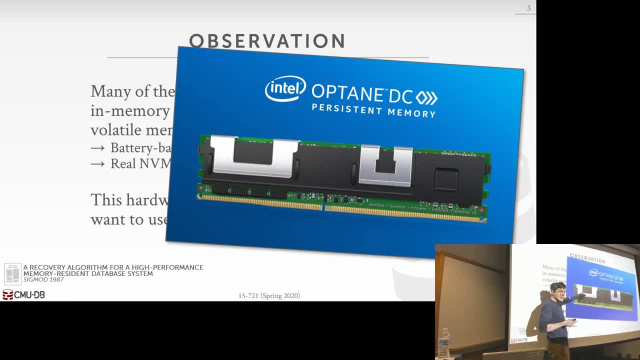 if I lose power, I I still retain everything. It's gonna be slightly slower than DRAM, but it's gonna be way faster than'thathet Dag DRAM, but it's gonna be way faster than aze, than SSDs. So we're not going to talk about NVM stuff or persistent memory right now. 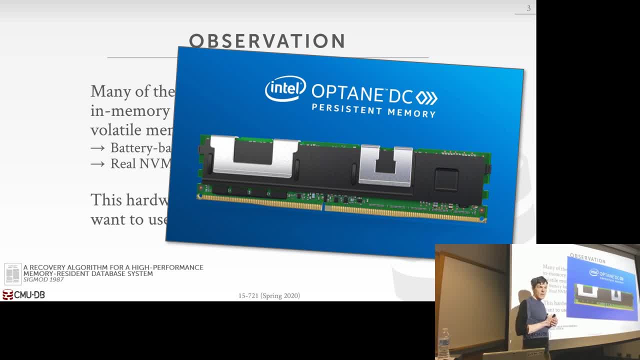 We'll cover this at the end of the semester. Yes, The question is, is it really expensive? What's that? What'd you say? Oh, yes and no, It's not like. it's not like outlandish, It's like maybe a couple thousand for like 128 gigs or something like that. 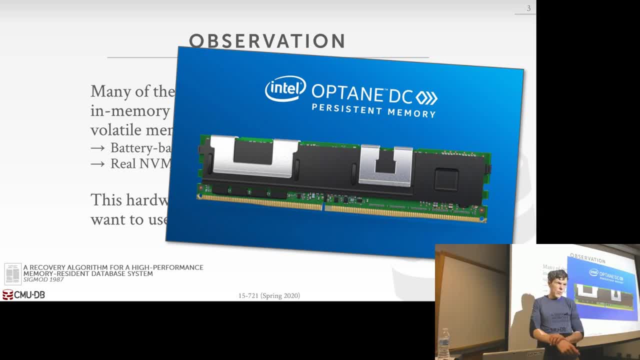 I don't know the exact prices. I don't think Intel publishes them. You can maybe only get it from OEM. But yes, it's more expensive than DRAM, more expensive than SSDs, but, like it, has certain properties that you can't get out of an SSD, 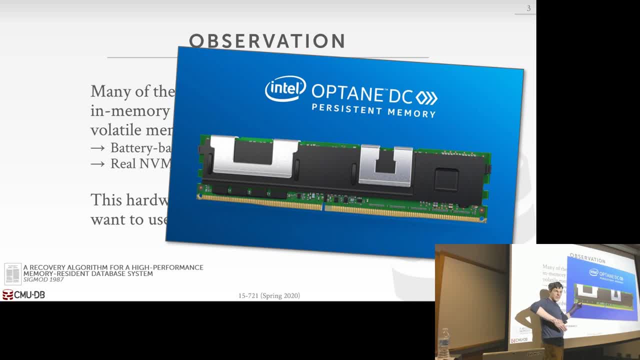 You can also get it in a form factor that goes down on the PCI Express. So it is that looks like a flash drive, even though it's a special. basically, it's not NAND flash, it's not DRAM, it's a special storage medium called phase change memory. 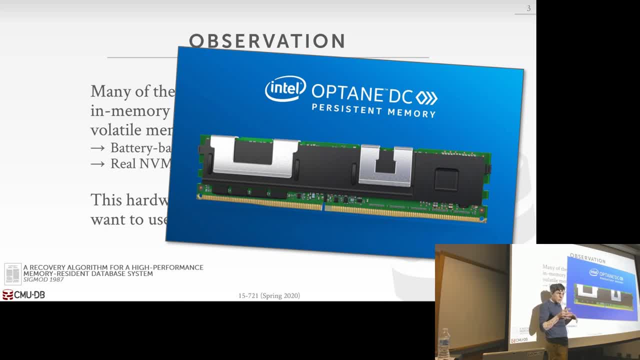 You can get it in other form factors and that one. those prices are close to what SSDs are, But for the DIMM stuff it's more pricey Again. we'll cover this later in the semester. The point I'm just to make is like: 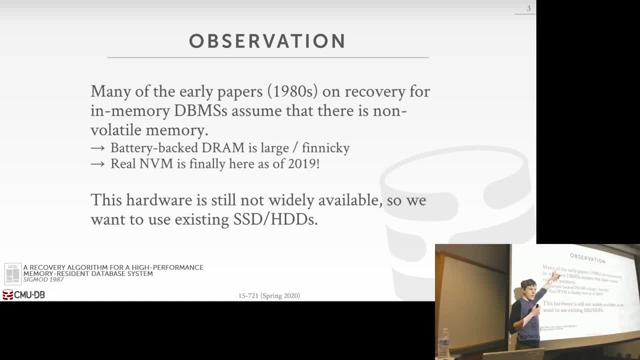 if you go read the early papers on logging protocols for memory databases, they all assume this, but back then they didn't really have it, So we still have to design our protocols using, you know, relying on SSDs or spinning disk hard drives. 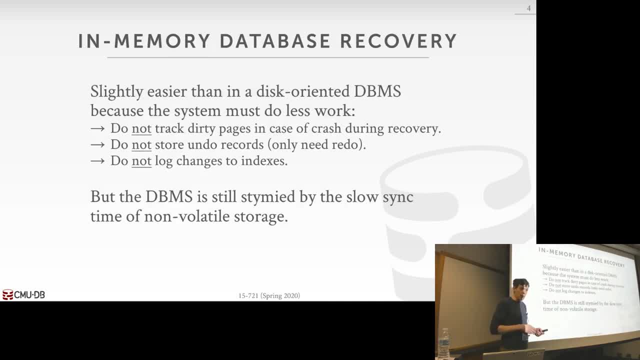 So the good thing, though, for us in an memory database is that our recovery protocol is going to be slightly easier than what we have to do in a disk oriented system, And this is just due to the fact that, since the primary storage location of the database is in memory, when we crash or there's a failure. 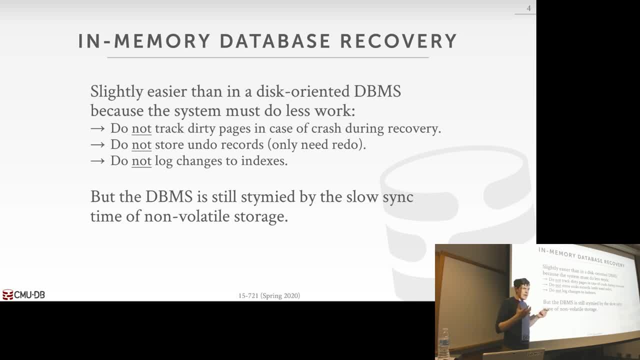 that memory is wiped. So when we come back, all we need to do is just load in the last checkpoint and replay the log from disk, and we don't have to worry about any dirty pages from transactions that may be lingering around on disk that we have to reverse. 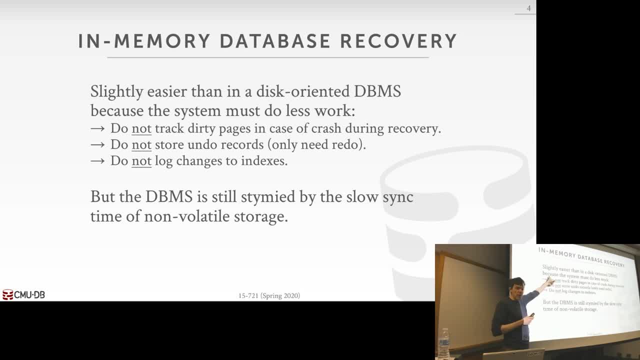 as we would in a disk oriented system. So we don't have to track dirty pages right as we run, Like if a transaction makes some changes and then it doesn't commit and we crash, well, all those memory pages get wiped. 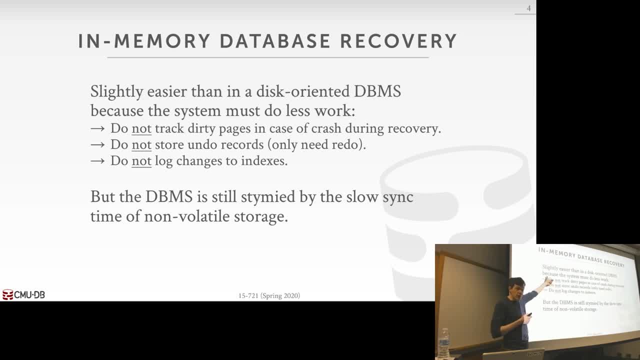 So that's fine. So this means now we don't have to store any undo records to reverse these things, because there's nothing to reverse. The only thing we need to write out the disk is just redo information. The other big difference is going to be that we're not going to log any changes. 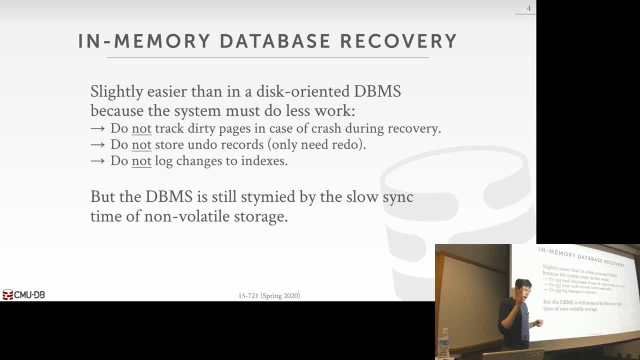 that we make to indexes. So in a disk based system, as I update my table and that causes updates to the indexes, I'm also going to create log records that record the changes to the index, But in memory. So in a disk based system, as I update my table. 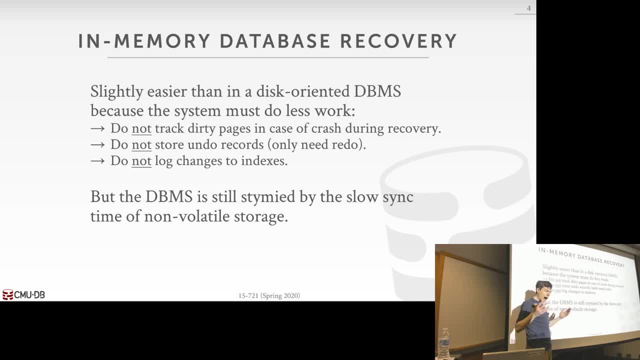 and that causes updates to the indexes. I'm also going to create log records that record the changes to the index, But in memory database I don't do any of that, And so when I crash I have to load the database back in from the checkpoint file. anyway. 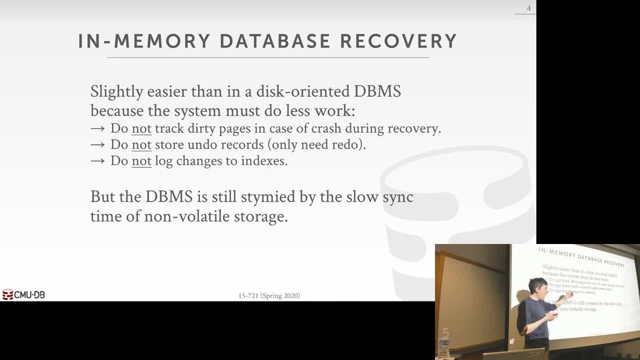 So the disk is way more expensive than doing the computation. So I'm just going to rebuild the indexes on the fly as I load the checkpoint in, And in a disk based system you don't do that. So we still have to deal with the fact that disk is going to be slow. 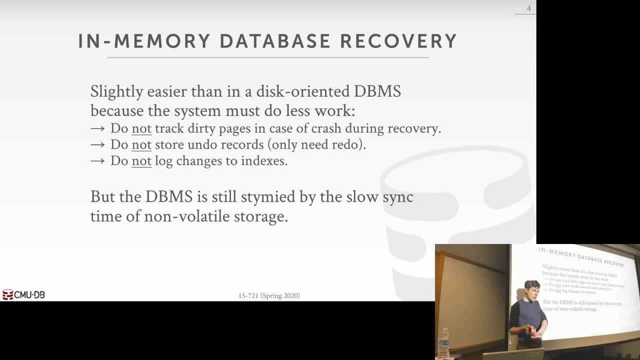 And so we still want to take advantage of all the optimizations we would do in a disk ordering system, like group commit, batching things, doing speculative lock releases, things like that. All of those optimizations are still going to apply for us here, even though we're in memory. 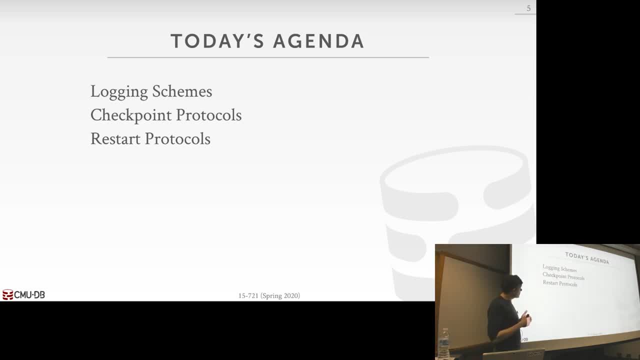 So today I'm going to talk first about different types of logging schemes And again, the paper I had you guys read was for a disk-ordering system, but it's relying on multiversioning. So I think that's really interesting and we'll see how that works. 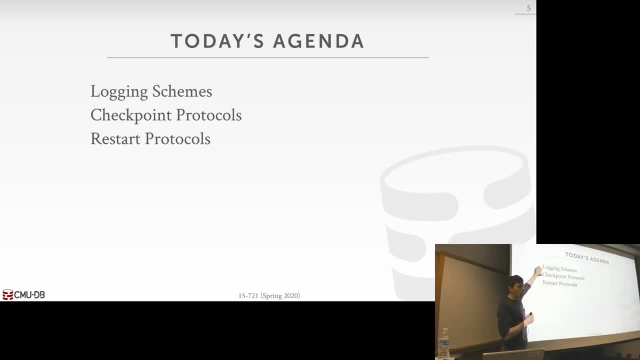 And then we'll talk about checkpoint protocols, And these two here are what you need to guarantee your database will. Actually, this is all you really need to guarantee your database is durable. This is a way to speed things up after a crash, and this is a way to speed things up. 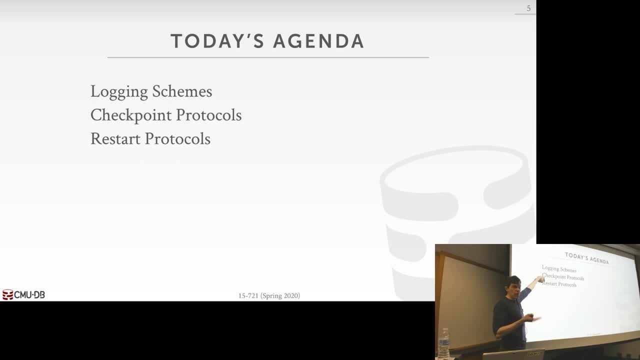 if you're going to do a restart and you know that it's going to be scheduled at a certain time, So this one you absolutely have to have. This one is an optimization to make this go faster and this is an optimization to avoid having to do all of this. 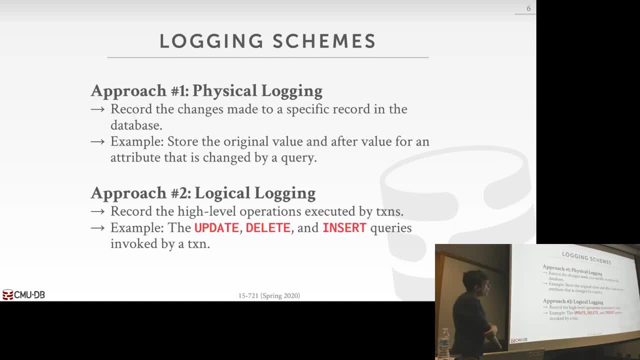 OK, All right. So at a high level, there's two types of logging schemes. There's physical logging and logical logging. Physical logging is like taking a diff, as you would in Git. The idea is that we're going to record the changes. 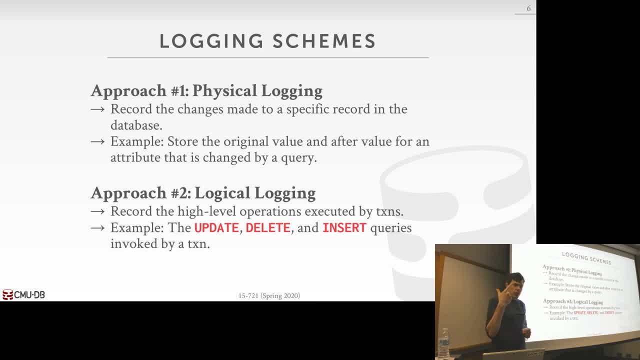 that we're making to a record at the byte level, If you think, also in MVCC, if you're using a Delta store. I'm just recording. here's the column that I modified and here's the new value. All right, 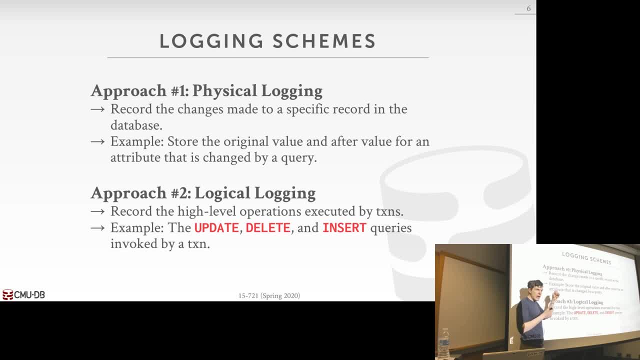 So then, after a crash, we're essentially just going to replay these log records and reapply the changes to the columns. The other approach is to do logical logging, and this is where, instead of storing again the low-level bytes, we're modifying within a tuple. 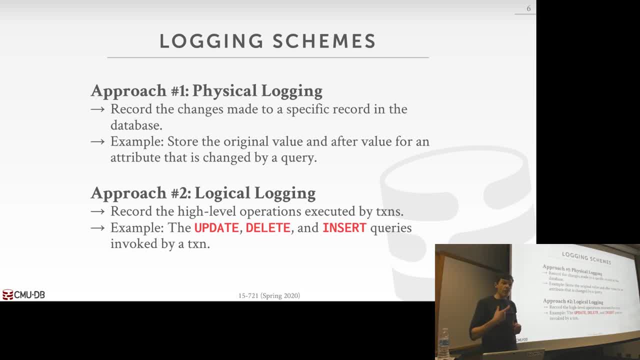 we're just going to store the high-level operation that the application invoked or requested on the database to make that change. So it would be like recording the actual SQL statements that they would send us: the insert, update, delete queries. So the idea here is: if I have a database, 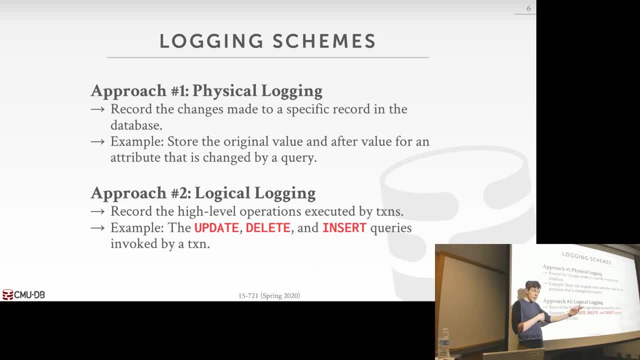 but the table has 1,000 tuples. make it big, make it a billion tuples. If I'm doing physical logging with one query that needs to update all one billion tuples, then I need one billion log records that correspond to every single tuple that I've modified. 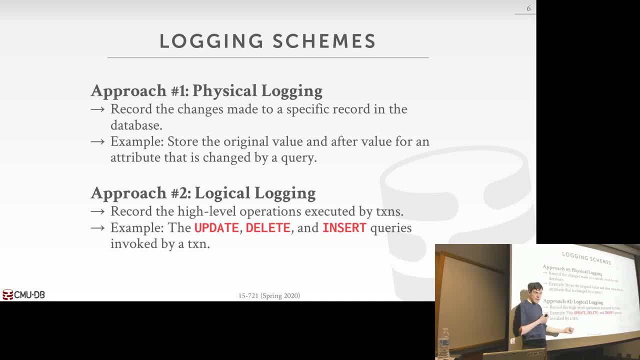 But if I'm doing logical logging then I only need to record that single update statement and that's enough for my system and I have to restart to replay that update and put me back in the correct state. So logical logging is going to be much smaller log files. 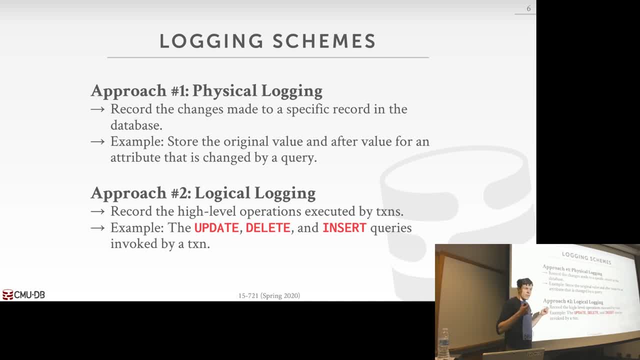 and potentially much faster to commit at runtime. but the recovery processes could potentially be more expensive because there's no magic I can do to make this update go faster during recovery. So if I have to update a billion tuples and it takes an hour the first time I run it, 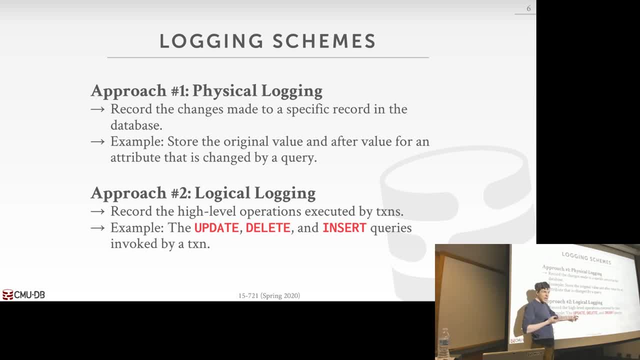 after I crash and restart and replay this update query, it might take an hour again, So it might delay the amount of time it takes for me for my database to come back online. So for this reason, most systems are going to choose physical logging. 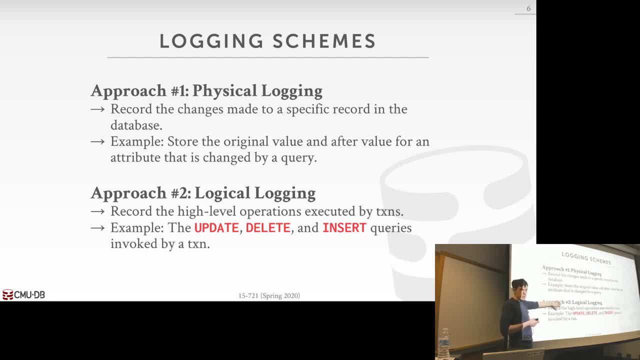 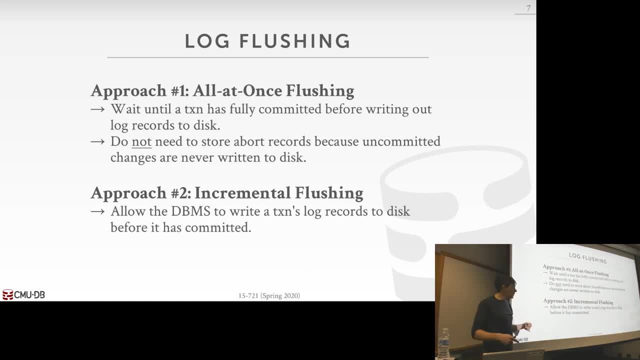 and this is only used in certain specialized systems. Okay, Now the question is: when do we actually flush the log records that a transaction generates? So the first approach is to do all at once, meaning as a transaction runs and they're making changes. 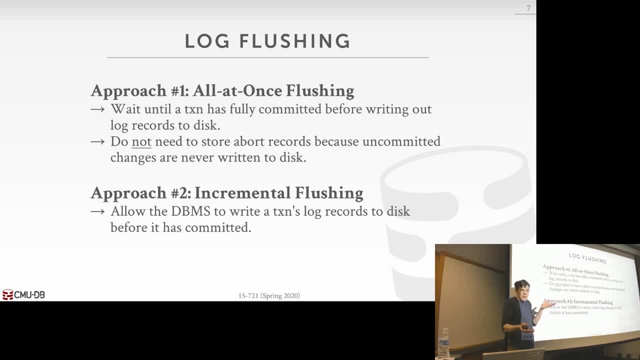 they're executing queries that update the database. it doesn't matter whether it's physical. it doesn't matter whether it's physical. it doesn't matter whether it's physical logging or logical logging. I'm just going to record in memory in this log buffer for my transaction. 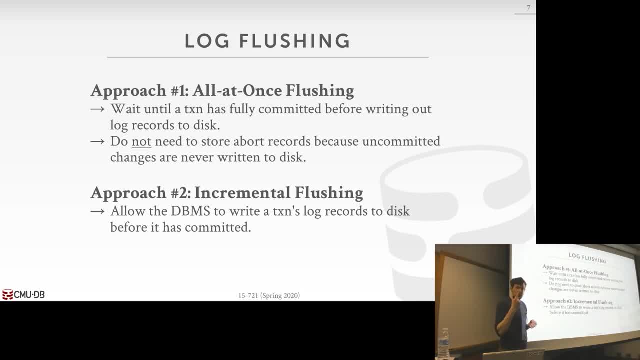 here's all the log records. And only when the transaction says go ahead and commit, we pass our validation. then we hand off those log records to our logger thread who then flushes it out the disk. Of course we have to wait until all those log records are written to disk. 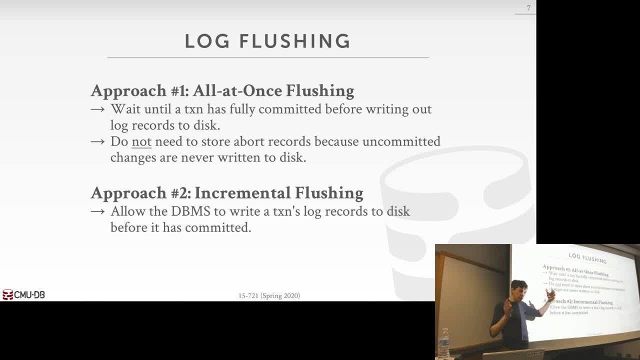 before we can tell the outside world that our transaction committed. So it could be, if I update a billion tuples and I update a billion log records, I have to wait for those one billion log records to get written to disk. The other approach is to do incremental flushing. 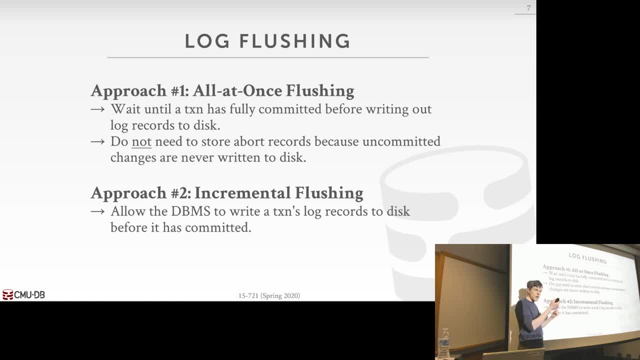 And this is as transactions run and they're accumulating these log records. when their local log buffer gets full, they can hand that off to some writer thread who can then start writing that off the disk and then they get a new log buffer to start filling up with new log records. 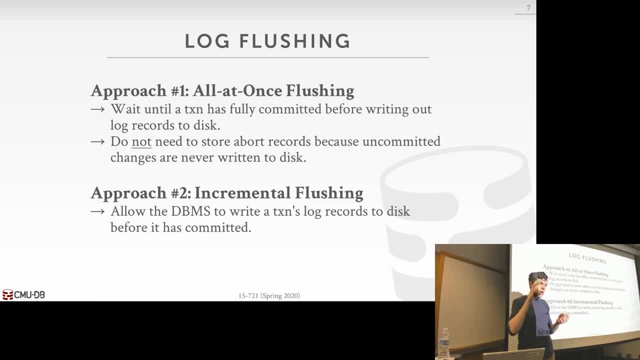 So that means that if there's a crash now in the log there may be log records from transactions that did not commit yet. Right, Because we're allowing things to get written out before everything is finished. So in this approach, here for the all at once. 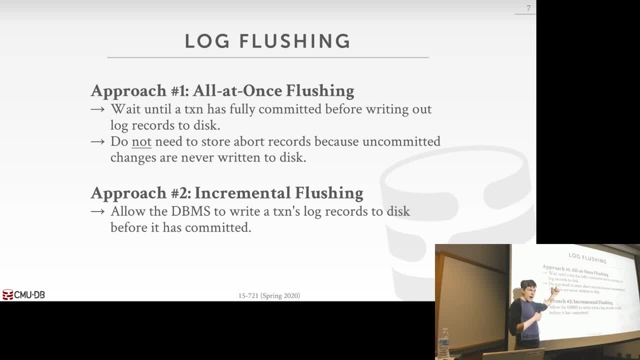 this makes recovery easier because I know if I crash and come back I'm almost never going to see log records from transactions that did not commit. I may see a transaction did commit and they start writing out all their log records but we crash before we write the rest of it and the commit message. 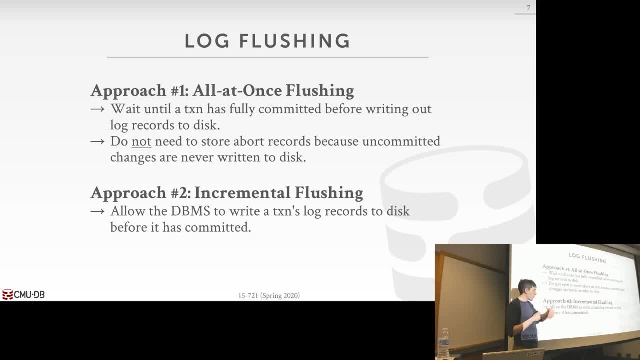 In that case I certainly have to undo it, But most of the times I'll have all the log records. In the case of incremental flushing I have to do some extra work to go figure out. here's a bunch of transactions that haven't finished. 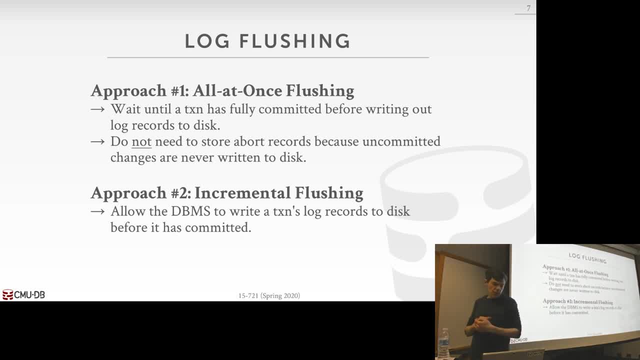 let me go ahead and make sure I don't reapply their changes. So this is not that big of a deal because again, we don't write out any dirty pages. we're reloading from the checkpoint anyway. it's just we have to do some extra processing in the log. 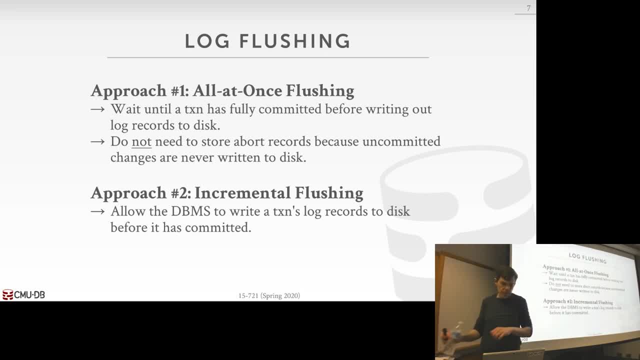 to make sure we skip things that shouldn't have committed. Yes, So the first thing: if a transaction is, let's say, inserting 10 billion tuples, and it inserted them and, sorry, it changed the log, it changed them and then it did something and those 5 billion things, 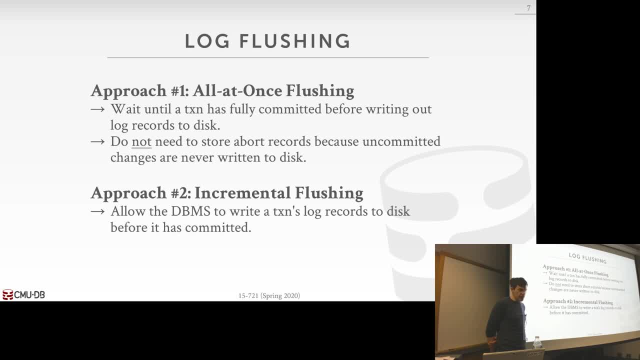 got stored and the last 5 billion things did not get stored Correct, And then it crashed also. Yes, So now how do you undo these last 5 billion things? Again, there's nothing to undo, No, but it updated things. 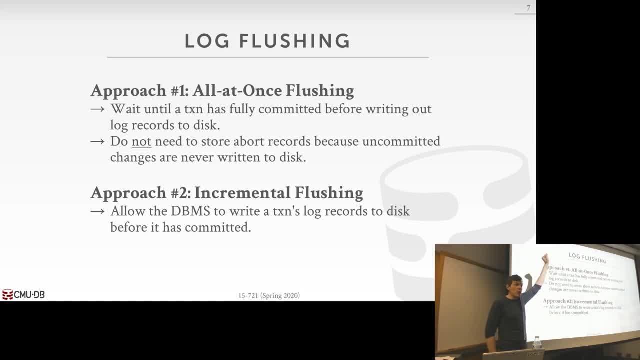 But updated what? Updated in-memory pages? We crash. that memory is gone. So when we come back online we're loading the checkpoint. there's no dirty pages, Right? It's just in this case here. we'll talk about replication in the next class. 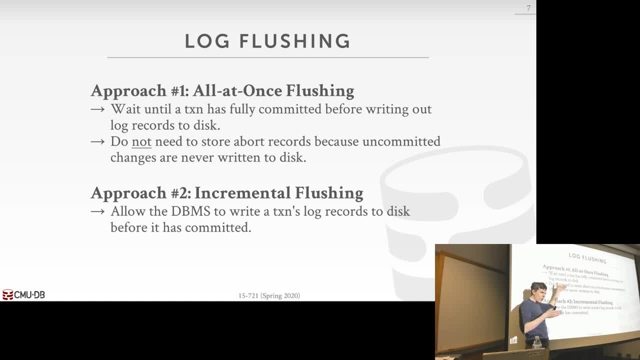 but it's sort of like: when do I send the outside world to a replica? hey, here's all my updates from my transaction. In this case also too, if I update 10 billion tuples, I have to have a log buffer that can handle 10 billion tuples. 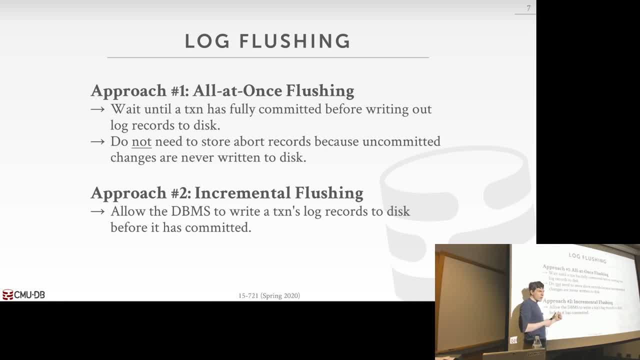 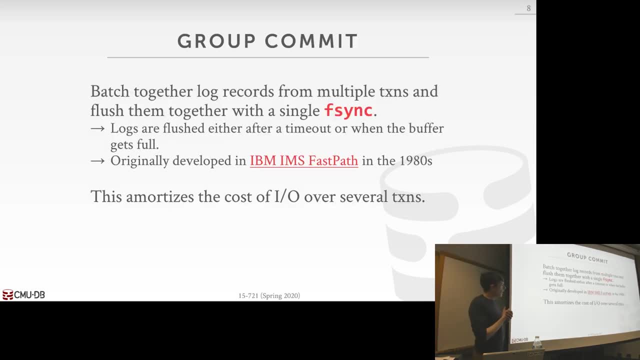 and I may run out of memory. So for this reason, most systems are going to do this approach, But there are some advantages to doing this. All right, these are the standard techniques we talked about before in the introduction. So the first thing we're going to do is we're going to do a group commit. 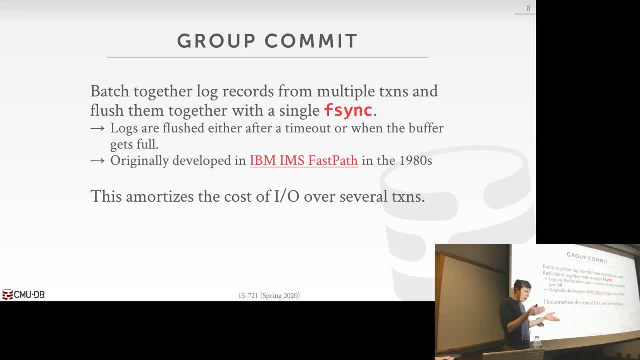 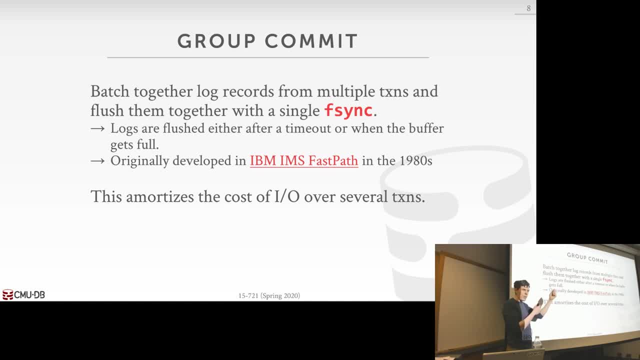 with log records from different transactions and that we can then flush them out whenever that log buffer is full and then have another log buffer start getting filled up by other transactions. And the idea here is we want to amortize the fsync cost across multiple transactions. 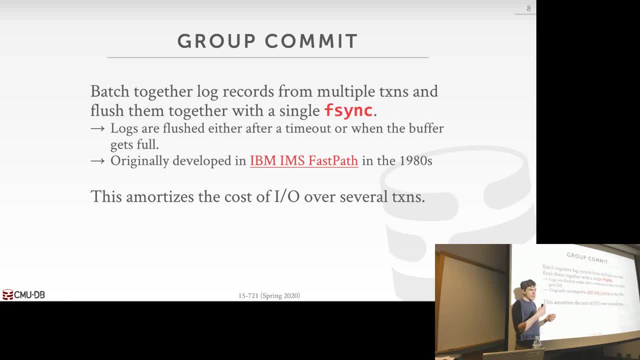 So if you're the first guy getting added to this queue, then, yes, you wait the longest because you have to wait for the log buffer to get full, And then you have to wait for the log buffer to get full, And then you have to wait for the log buffer to get full. 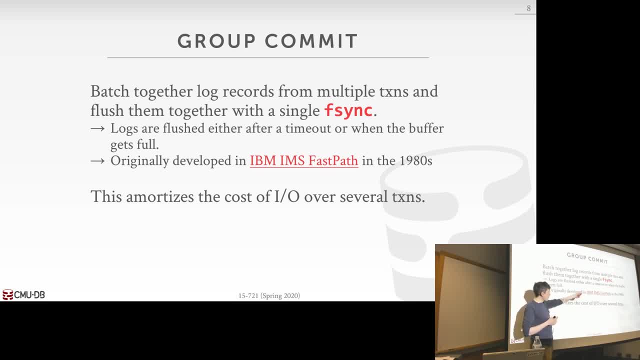 And then you have to wait for the log buffer to get full. So this is basically running with a dedicated fsync call. So this is a really old technique. As I said, it's used in pretty much every system today. It was originally developed for this thing called FastPath. 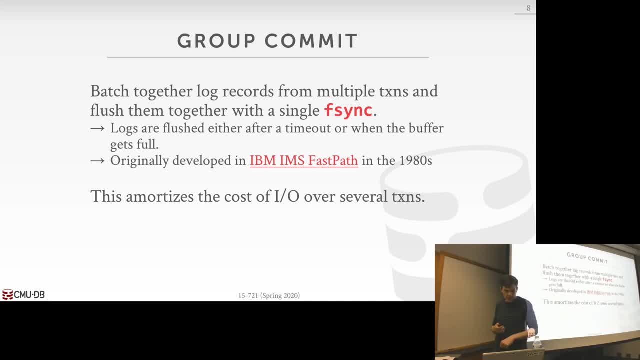 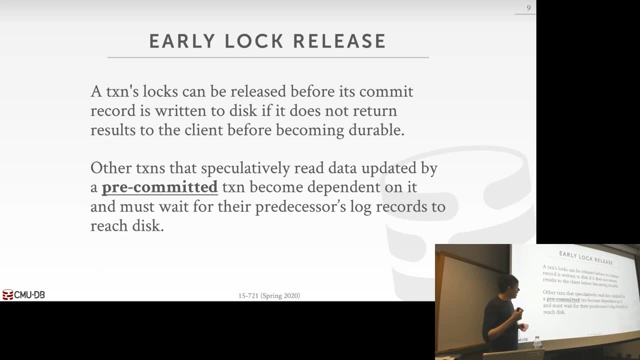 which was a specialized in-memory engine for IBM's IMS from the early 1980s. But, like I said, everyone pretty much does this today. The other thing we can do now, which is related to the speculative lock release or speculative reads, 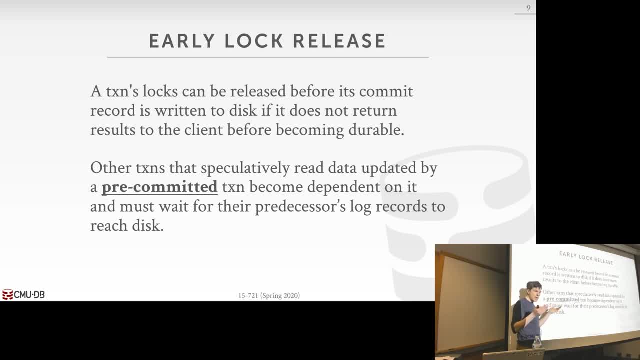 which goes ahead and commits. we don't have to wait for the updates to become durable on disk before we release all our locks. We can let other transactions start modifying the tuples that we've modified, assuming those log records will get written out of disk. 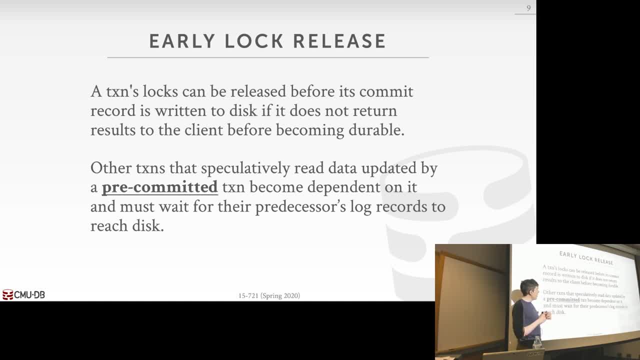 Or they read things that we modified before the log records get flushed to disk And we have to sort of keep track of that. We did these speculative reads. even though the transaction is logically committed physically, it hasn't gotten rid of the disk yet. 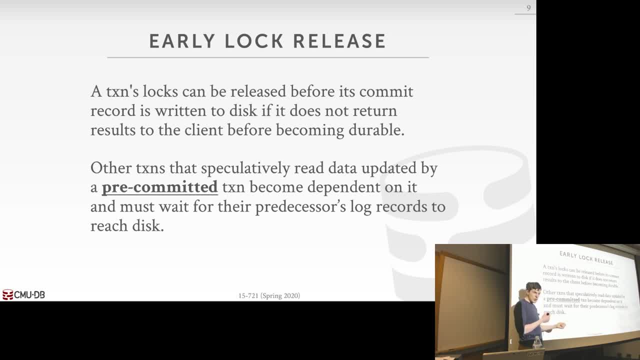 So we know that if any transaction reads something that we wrote, they have to get stalled until we actually flush the disk. So that means that my read-only transaction that it reads an update from your transaction, but your transaction hasn't been written to disk yet. 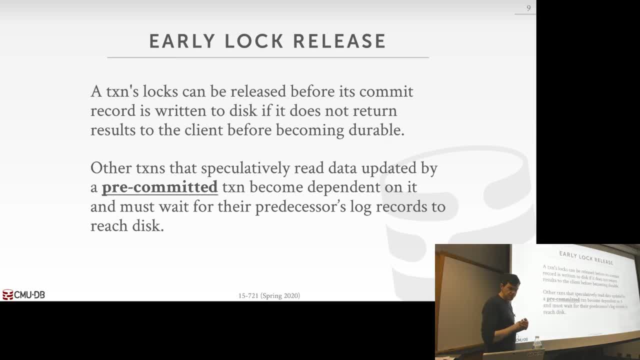 I have to wait for you to get flushed before I can get committed Again. this is a standard technique And on MVCC we would know this information because we maintain the state map that says this transaction's log records have not been flushed yet. 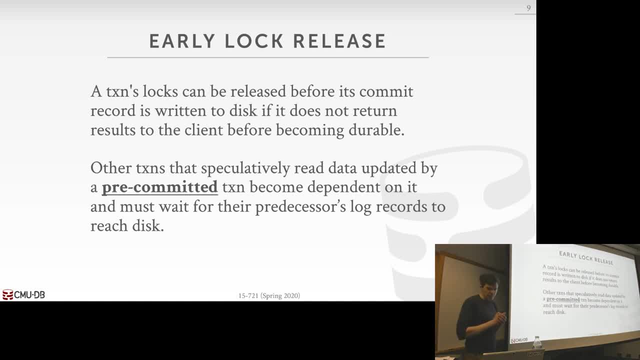 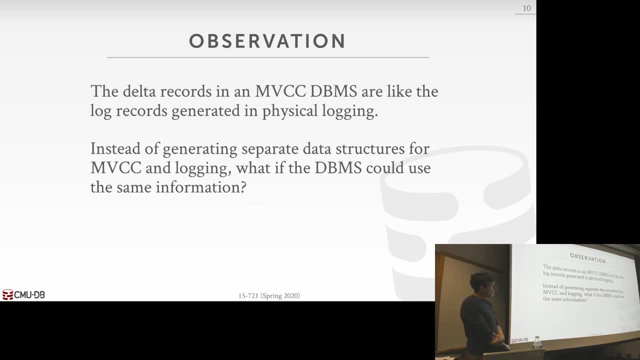 so therefore, you can't commit right away if you read something from them. Okay, So I sort of alluded to this a little bit now in the last couple of slides, where if we have a multiversion system, then the delta records we're going to generate for MVCC. 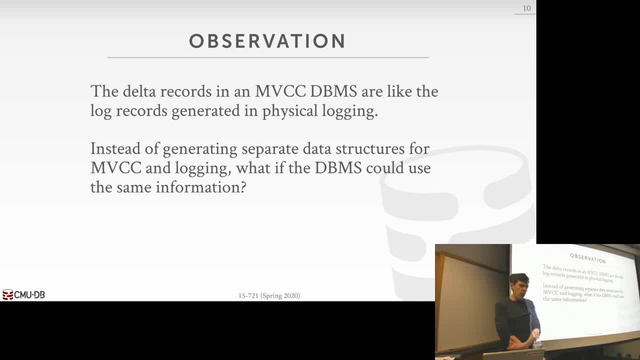 are more or less the same thing we're going to generate in our log. It's not exactly the same because, depending on if we're doing oldest to newest or newest to oldest, we could be generating redo records or undo records for our tuples we're modifying. 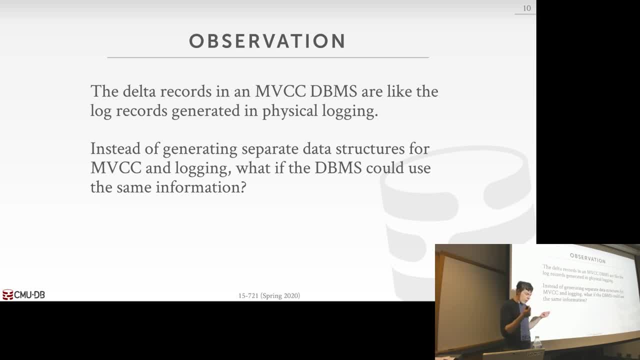 whereas the database log file wants to have redo records, at least for an in-memory database. So the idea is that what if we can combine all the metadata we're generating for MVCC with all the metadata we're generating with the log file? 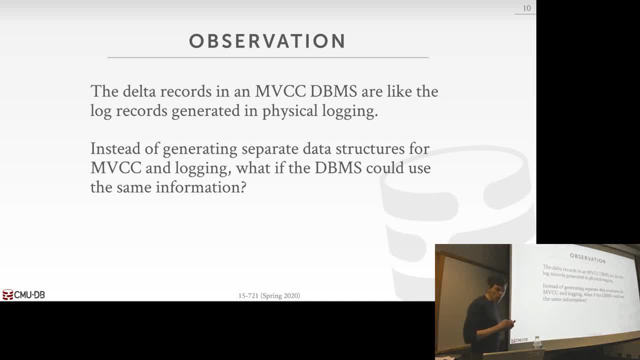 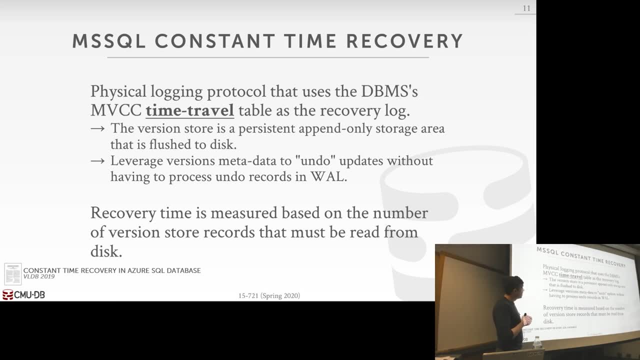 and that way we're not duplicating this effort. So that was the paper I had you guys read for today. It came out just this year, or last year, in VOD 2019.. So, as I said, it's not an in-memory system, but it's a multiversion system. 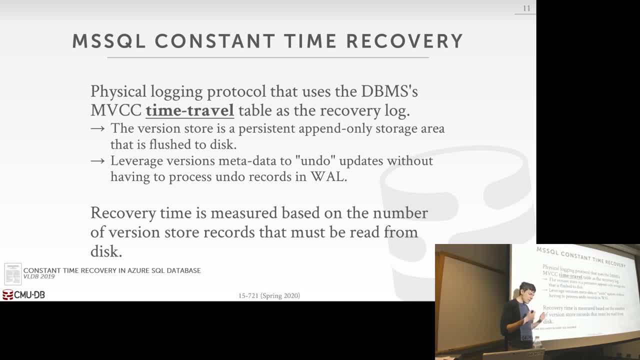 and I think it's a good description of how you can piggyback off of the MVCC metadata you're generating to make logging work better. So this protocol is going to be a physical logging protocol that's going to rely on the database system's time travel table. 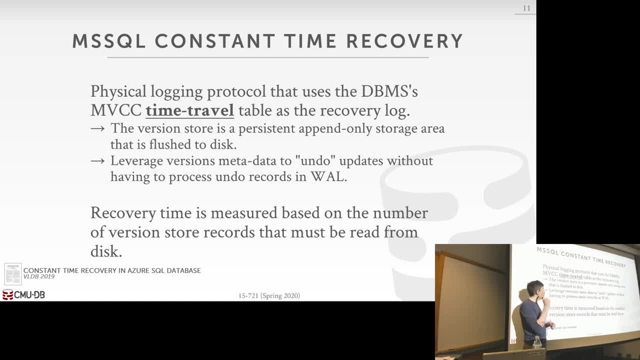 which they call the version store, the tempdb. So we're going to rely on that time travel table to act almost as a recovery log. So what'll happen is we'll start writing out the changes we make to this version store to a log file, but they're only going to contain essentially. 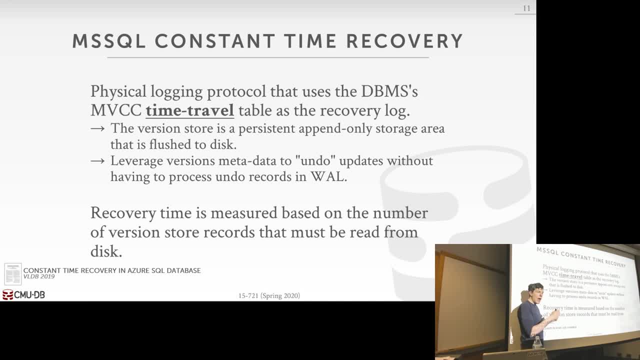 the redo records of the versions we've generated And then, when we crash and come back, all we need to do now is just suck in this version store into disk or, sorry, alpha disk- into memory, and we don't need to undo anything right away. 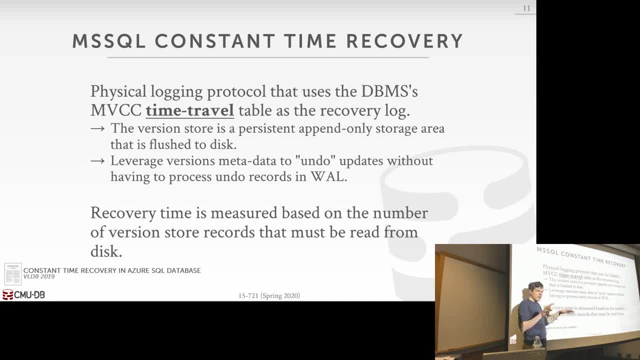 We just bring those pages back in, then the database is now at the state it was at the moment of the crash, And then we just need to do some background extra work to do this logical revert, to make sure that we don't read things we don't persist versions. 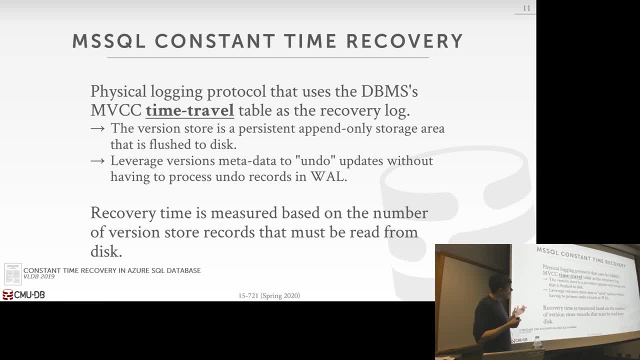 from transactions that did not commit at the crash. So the problem they were trying to solve- that they mentioned in the paper- is that they had certain customers running on Azure in the cloud or SQL Server in the cloud, where they would have these really long. 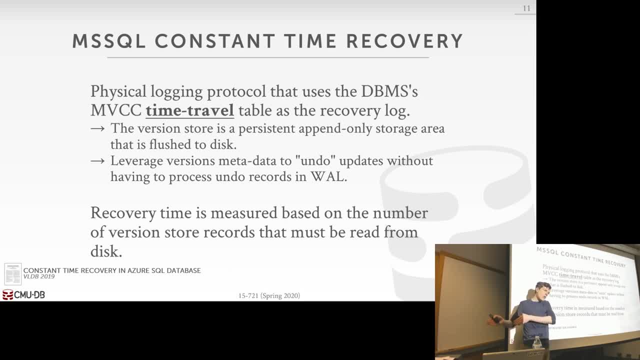 transactions that when there was a crash. now you need to undo all the changes. So this 10 billion table update we just mentioned- Like if I crash before I finish updating all those tuples when I come back now. I've got to spend a long time undoing everything. 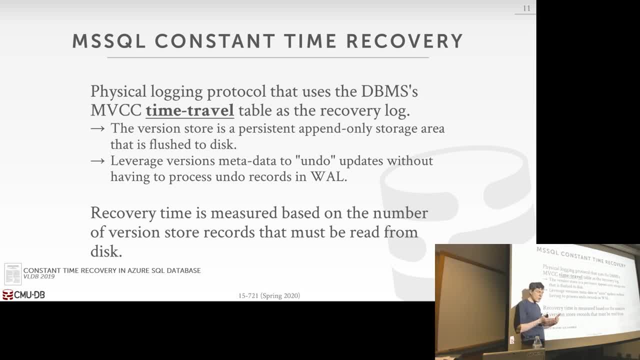 So what they wanted to do is have what they call constant time recovery, which was saying that the time it's going to take for me to restore the database back to the correct state is only contingent on the size of the log file, because I just need to be able to read that in the redo phase. 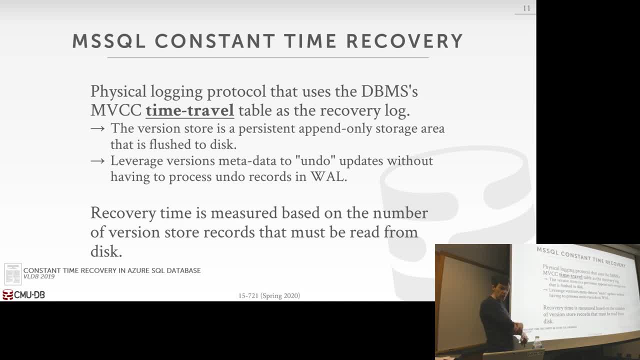 And I don't have to worry about how much time I'm going to spend going in the reverse direction to undo things. Does that make sense? So let's go through some examples and then we'll see how it works. So again, there's a lot of things that we can do. 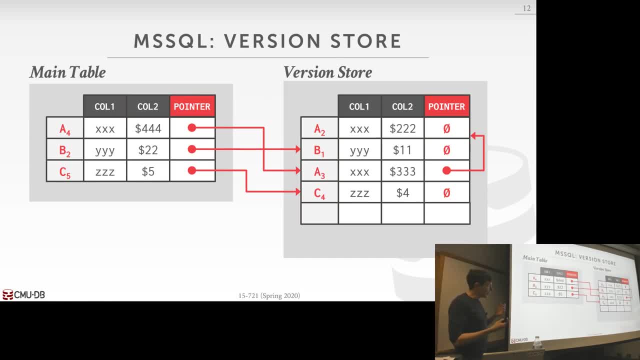 This is with SQL Server. Azure SQL is the name of the cloud version of it. But, as I said, for this feature they're putting out in the on-premise version, which includes the Linux one. So they're doing time travel version storage, but they just call it a version store. 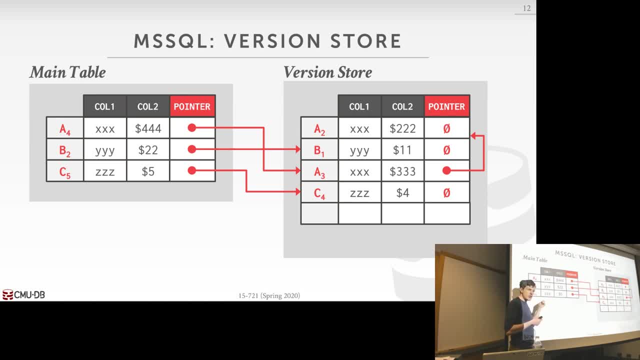 And so the idea here is that you have the main table and this has the latest version, and they're doing newest to oldest, So this version has a pointer now to another tuple. that's the next oldest tuple, and then there's a version chain. 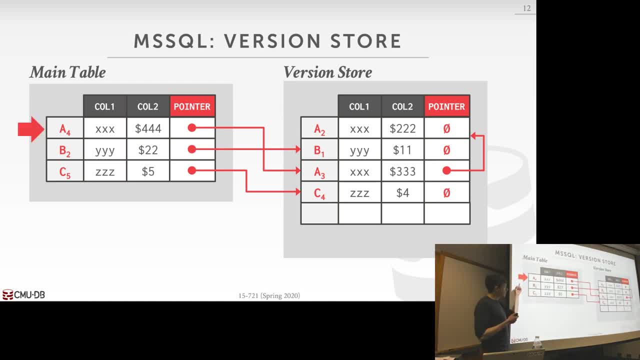 allowed to go back in time to find previous versions. So now, if a transaction comes along and wants to update this tuple here, we first make a copy of the current version into our version store, update the pointer to connect the chain and then we can overwrite the old version with our new one here. 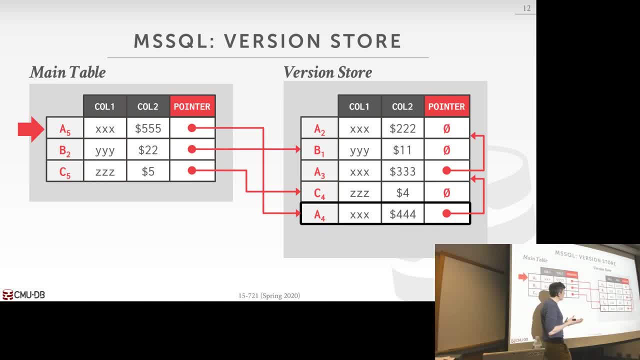 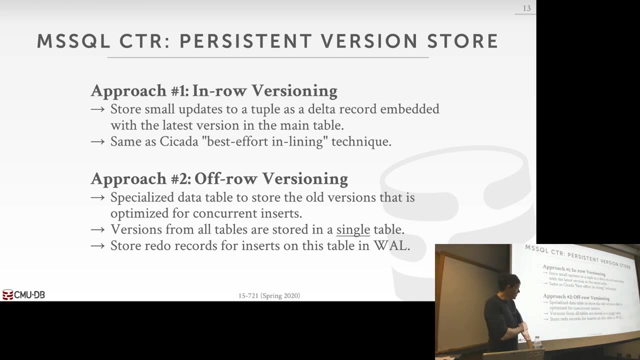 Right. So the idea here is that they want to leverage this thing, which is basically redo information, all right, to then allow them to restore the state of the database just by loading this thing back in. So there's going to be two variants of how they're going to do this. persistent version store. 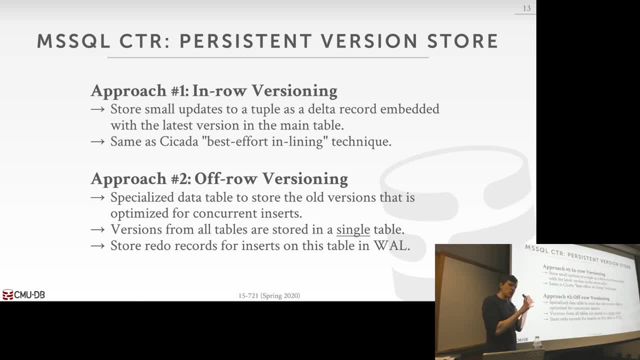 So the first one is that they're going to do in-row versioning. where this is actually, you're not going to use the version store. This is going to look like that Cicada inlining, where, instead of making a whole copy of the tuple and putting it into the version store, 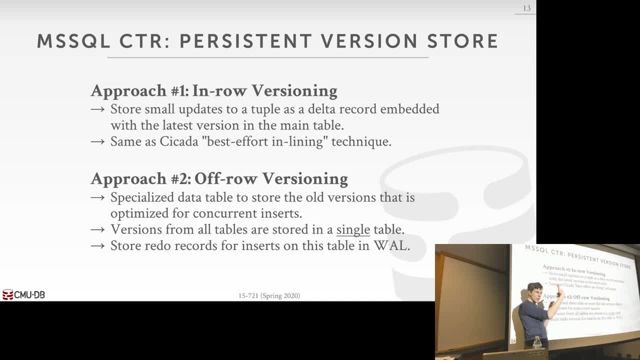 they're going to pack it in the special field inside the tuple of just the delta record of what was modified And then that gets written out to the write ahead log just as it would any other tuple update, And that's enough information to be able to recreate the database state. 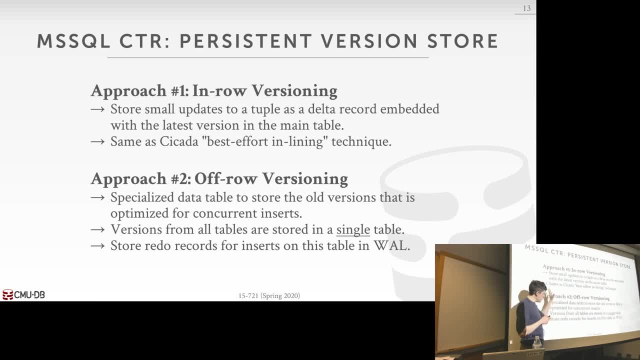 I'll show this in the next slide. And then for the off-row versioning, which is actually using the time travel table. instead of having a time travel table for every single logical table in your database, they're going to have one giant time travel table for every single table. 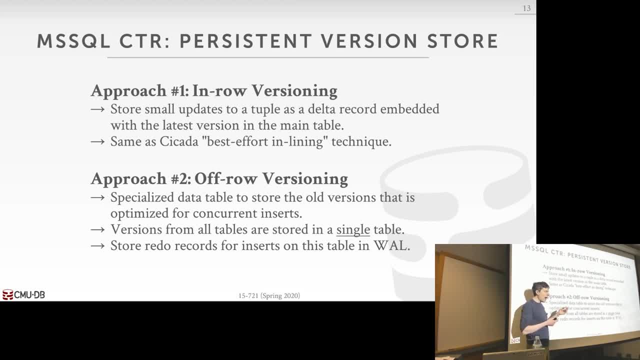 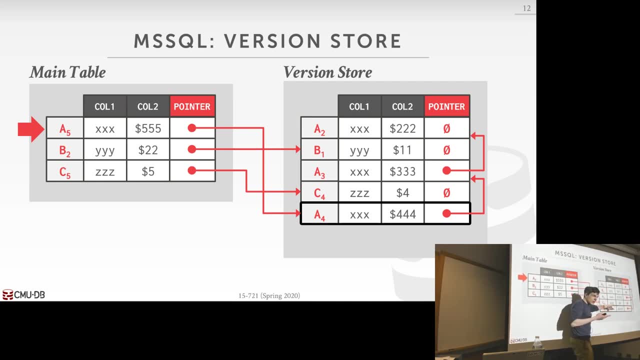 This is way different. I've never seen this used before, And so the way it works is that the in here, instead of having discrete columns or attributes that represent the columns in the table, they're just going to have one column and then just store a blob or a byte string of the serialized data for that tuple. 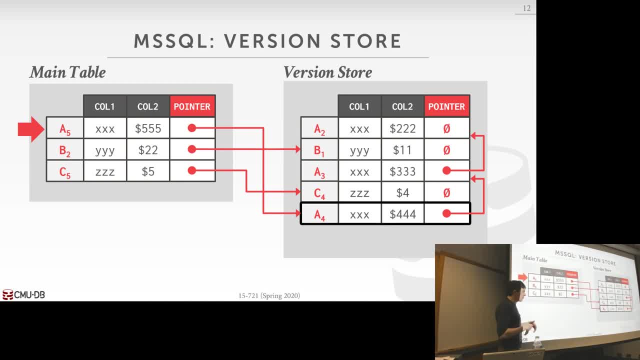 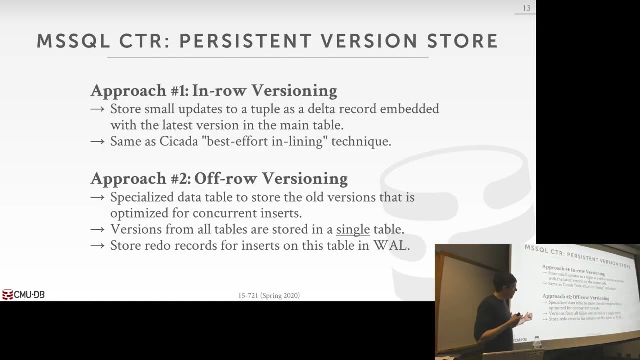 And that way you can store any tables tuples inside there, Because there's no, we're not doing any processing on looking at the actual columns in this. We're just almost using it as an in-memory log that then gets flushed. So they're also going to modify the data table data structure itself so that you can do fast concurrent inserts. 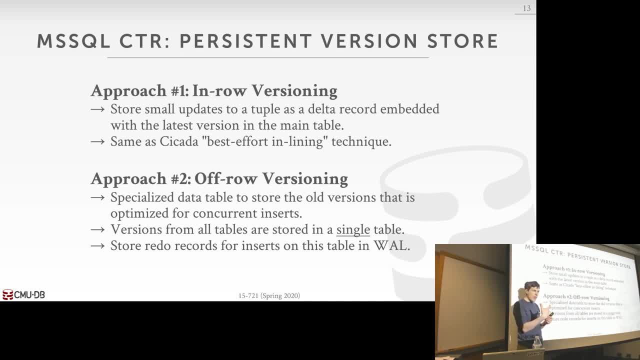 So that means that they're going to partition the database in memory so that, or sorry, the table in memory, so that different threads write to different regions of the table, And then this allows you to you sort of write them out very quickly to the write ahead log. 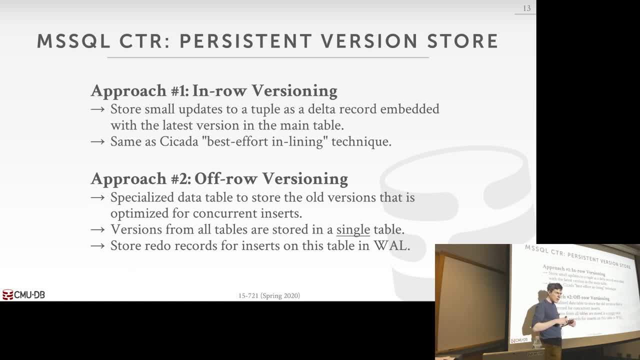 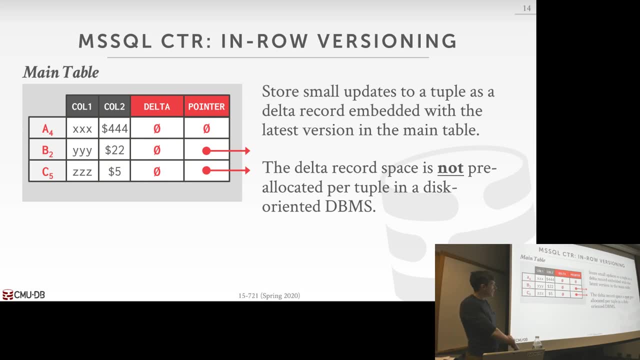 And you never can allow it to go back and update any other tuple, right? It's only append only, And now you do sequential writes out to the log, which is efficient. So this is the in-row versioning. This is the same thing we talked about with Cicada. 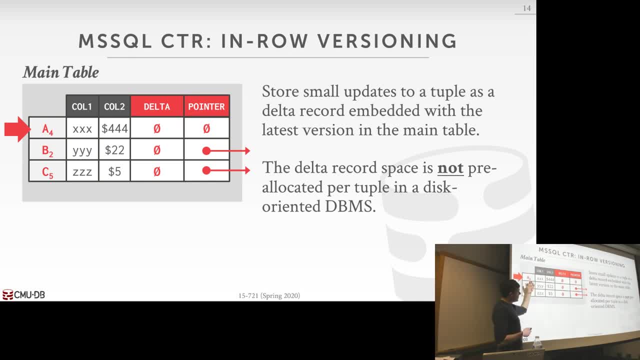 Basically they, when I do an update of this tuple, instead of making this copy of this old version and putting it into the time travel table, those embed a delta record inside of here And then that just gets written out to a write ahead log, just as you normally would. 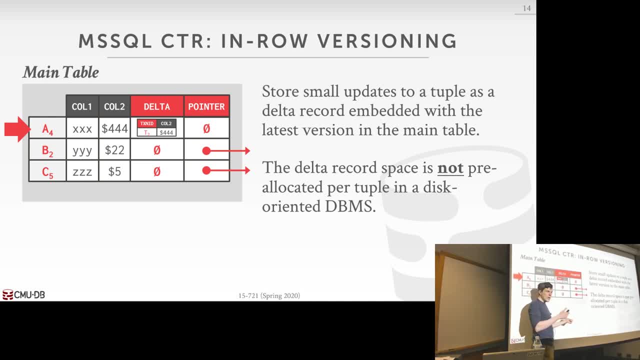 So an important distinction here about why they can do this and why we can't do this very easily in an in-memory database system is that in a disk-oriented database the tuples can be very, very length. In an in-memory database we said we had, the primary location of a tuple has to be fixed length. 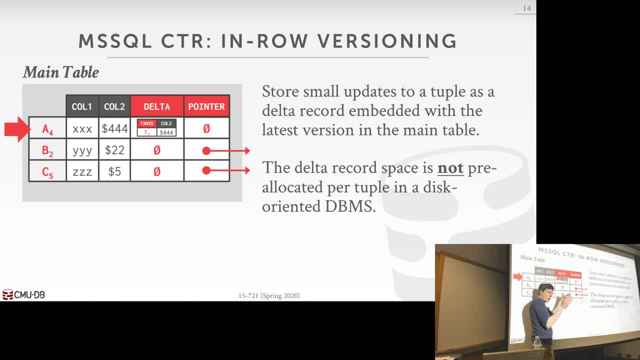 So we either have to allocate this delta space for every single tuple- it can only be a certain size- if we're in-memory, But in a disk-based database I can leave this thing empty- And then, if I decide to use it, when I insert the new tuple. 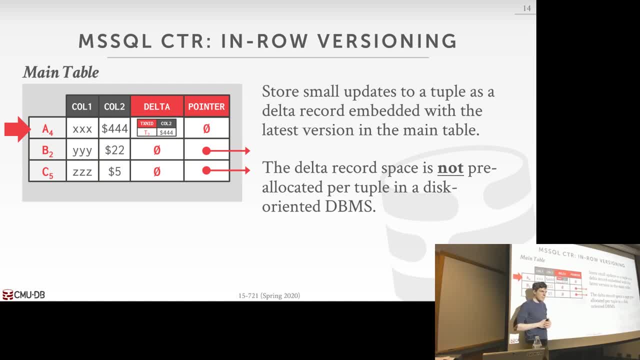 then I just grab a new slot in my page and can write everything out, Right? So that's one important distinction between what they're doing and how you do this in an in-memory database. Okay, So let's see how they're going to do recovery. 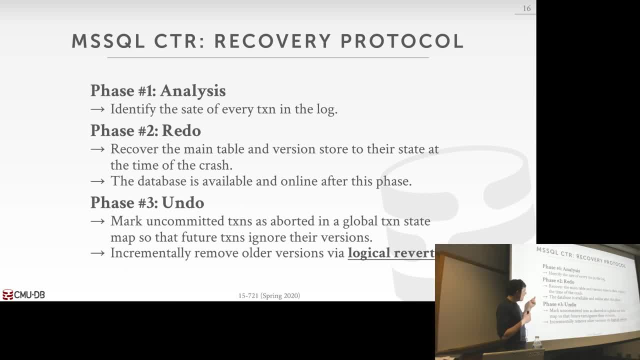 So this almost looks like standard ARIES, except that under ARIES the database is not available until you complete the undo phase. In their world it's immediately available after the redo phase, Because all they're doing is they're loading back in that version store. 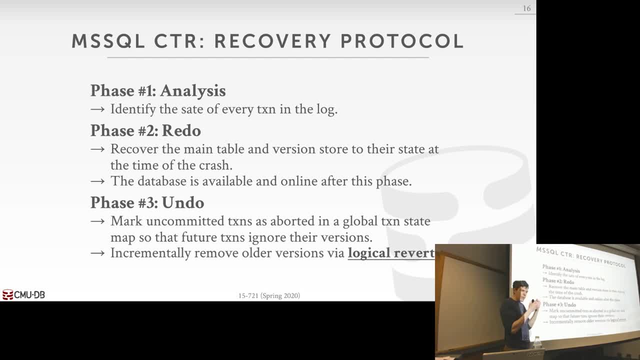 and then all the old versions that are around are now available And then we just piggyback off all that same version detection or identification that we do under MVCC To identify which tuples are actually visible to our transaction. So analysis phase again, we just scan through the log up to the last checkpoint. 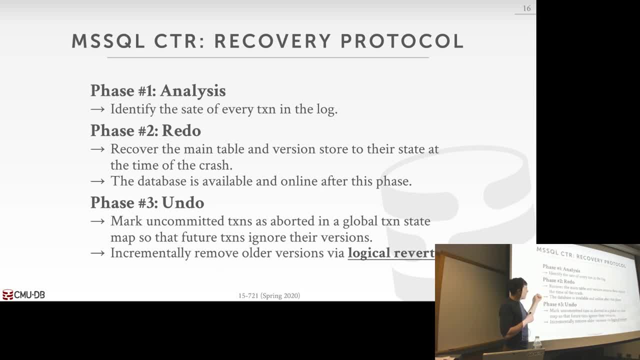 to figure out what transactions are running And then in the redo phase we're going to replay the write-ahead log to put us back in the correct state for the main table in the version store. But, as I said, the version store is only going to contain versions. 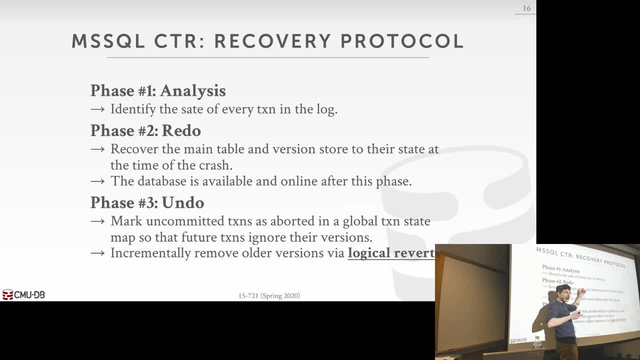 from transactions that did not commit as well as in the main table. But because we're MVCC, we know what the timestamps were for those versions And then when we come back online and start running regular transactions, we would know to skip over things that were uncommitted. 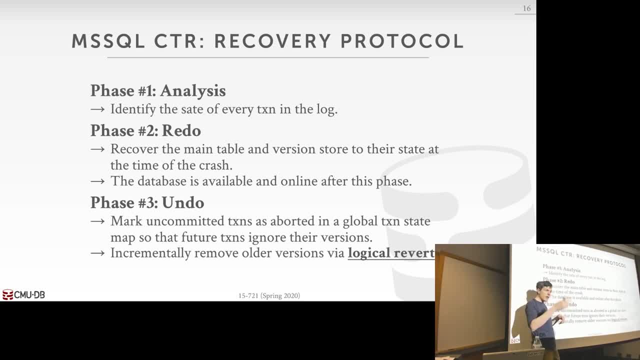 Because we're going to maintain this global state map that says here's all the transactions that are around and here's what their status is. Then in the undo phase, we select transactions to start execute And when they find things that are aborted, they can go ahead. 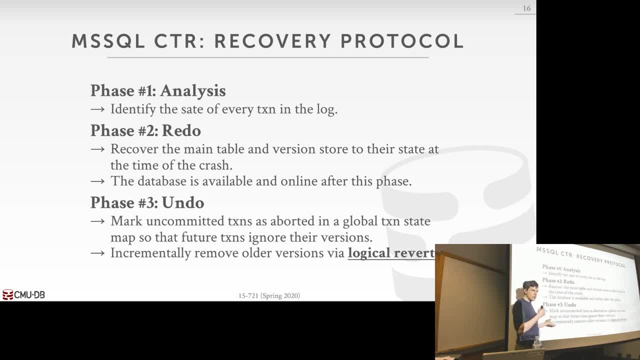 either clean them up or there would be a separate background process to clean them up asynchronously, And they refer to this thing as a logical revert. But from a logical revert perspective it's a logical revert. For my purpose it just sounds like garbage collection. 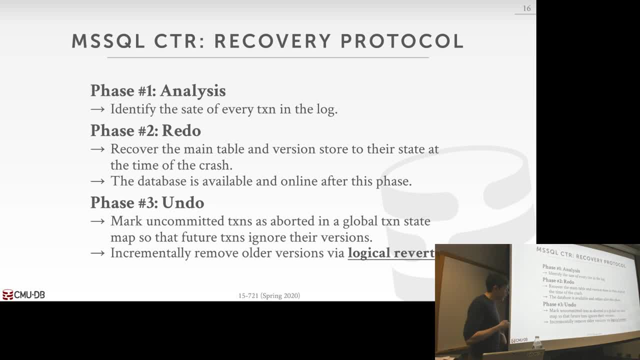 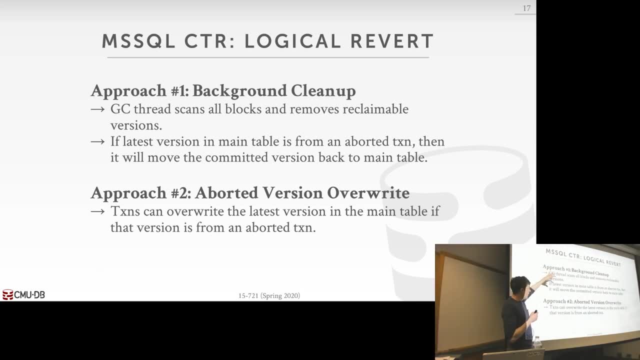 Although the fact that transactions can do something slightly different when they find aborted versions is not exactly garbage collection. So this is already what it says. So you have separate threads. they're going to scan through the blocks, find all the reclaimed old versions. 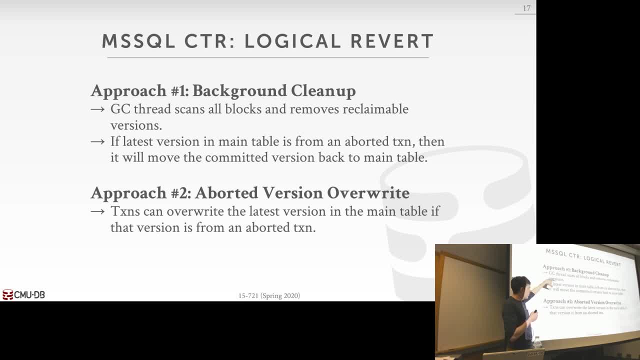 And then if you recognize that the latest version of a tuple is in the version store, then you just move it back into the main table Again. that's the same thing we would see in regular GC that we've already talked about. The only one optimization they do. 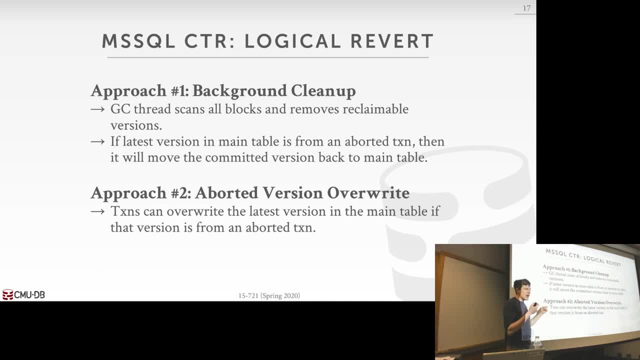 that's slightly different is if a transaction recognizes that. oh, in the main table I see the current version. the master version of the tuple is from an aborted transaction. then instead of copying that out and making a new version in the time travel. 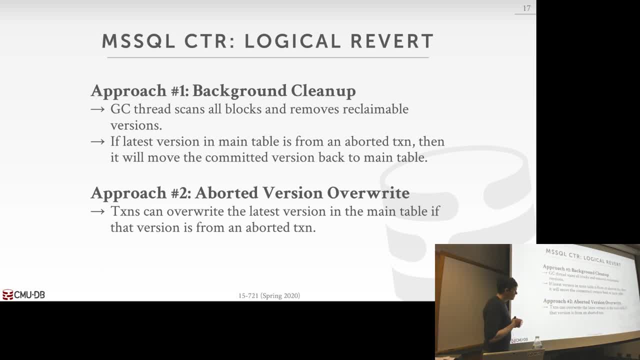 they just completely overwrite it, right. So, again, like I said, I think this is interesting because this is, although it's a disk-based system, it's showing you how you can use the MVCC metadata to do a different type of logging scheme. 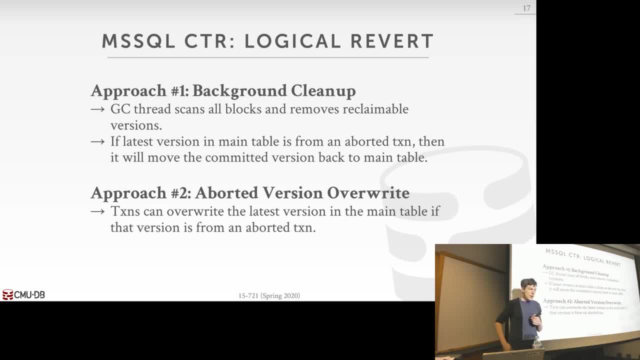 And essentially get better performance. Any questions about this? There's this other bit about the syslog where they would store changes for non-version data structures like page tables and people street layouts. That again, we can ignore all of that in memory system because we're not going to maintain that information. 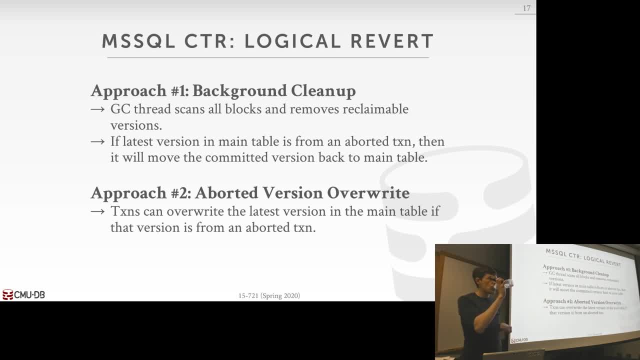 Yes, Are they paying extra cost when they are reading from the data storage and that thing is serialized so they can like. Yeah, so he's correct. like, does this mean at runtime? if I need to go read an old version, I have to go to the version store and everything is just serialized as a blob. 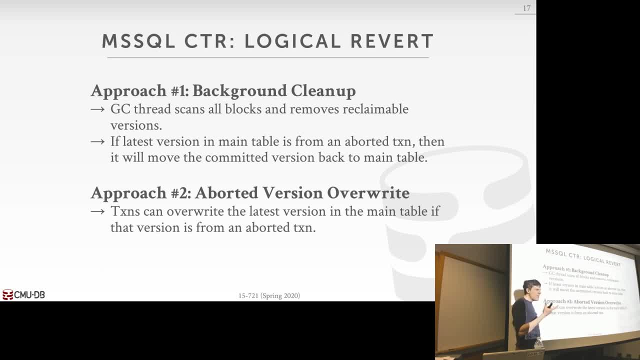 do I pay a penalty for having to read that? Yes, but I think they measure it. it's kind of small. Same thing with the delta record. if I have the in-row delta record, I have to replay it and they pay a computational cost for that. 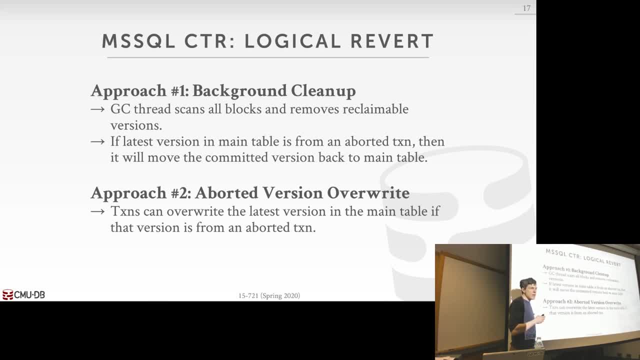 If it is in-row, then you don't have much penalty, right? This is what they say, that Yeah, but it's not, as It's not as free as like going reading and having everything there. I agree with you. yes. 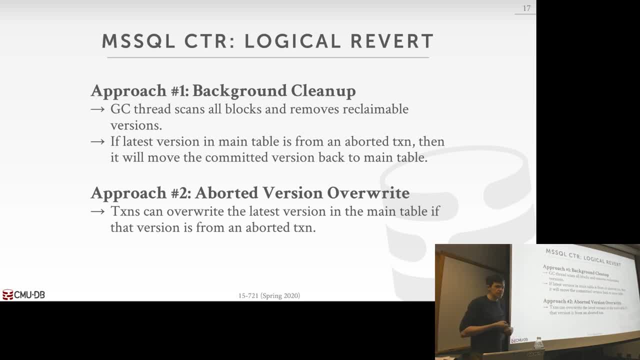 Yeah, and that's why we use DeltaStore in our own system. Most transactions- I don't remember if they say this in the paper- most transactions don't update all columns. That's right. the DeltaStore is The in-row version is usually going to be enough. 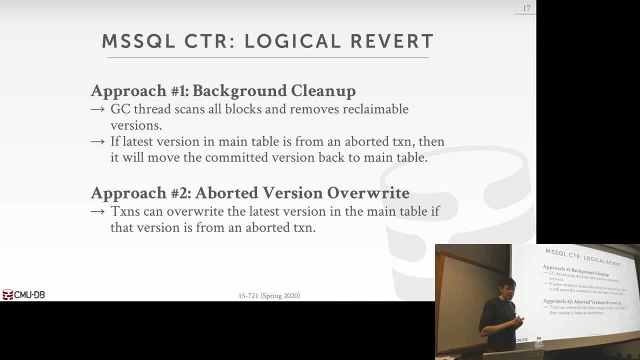 So this idea of what they're doing is not new. This is actually very similar to how Postgres was originally designed back in like 1986.. Like in Postgres, there's a paper called The Design of Postgres, and Sternbaker talks about how. 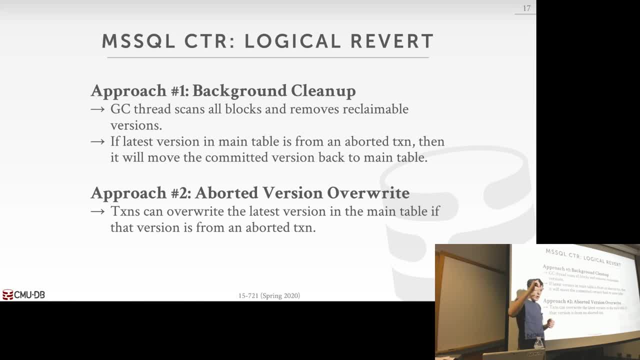 oh well, the log is not really a log file, it's a log table and everything's getting appended to that and that gets flushed out. So at a high level this is very similar, And they claim. the difference here is that this paper is about taking a system. 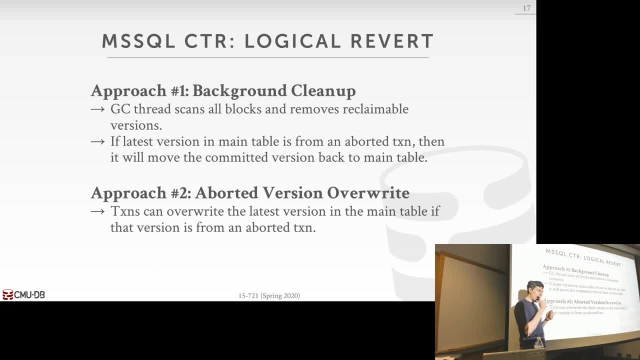 that was not designed to be multiversion in this way, and adding this after the fact, whereas Postgres was designed from the very beginning to be like this. And again, Postgres is an MVCC system. okay, All right. so again, this is a protocol that takes advantage of the fact that we're multiversioned. 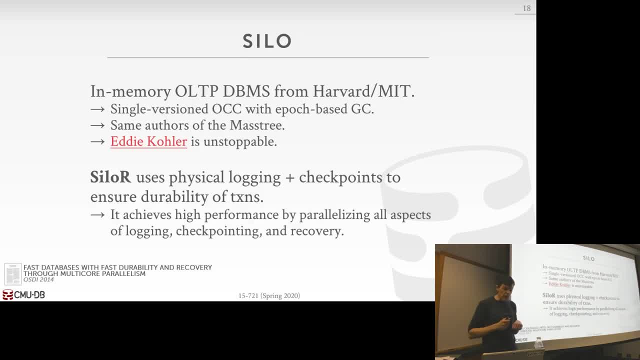 So now let's look at another logging protocol, that is, for in-memory databases. that's more about how you could architect the system to be aware of how the CPUs actually work and how they operate. So Silo is a memory OTP embedded database engine that was developed out of Harvard by Eddie Kohler. 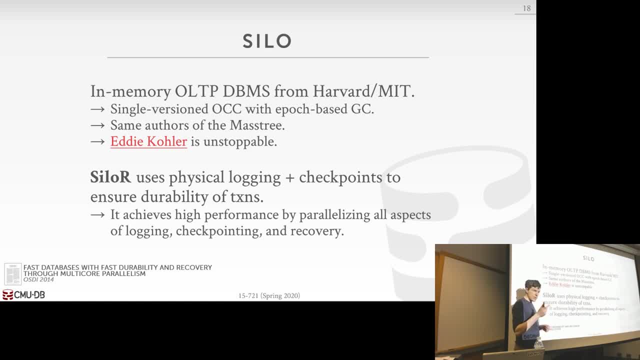 So it's not going to be multiversion, it's going to be a single-version system that uses OCC, and they're going to use an epoch-based garbage collection protocol to keep track of when you actually commit transactions and flush things out the disk. 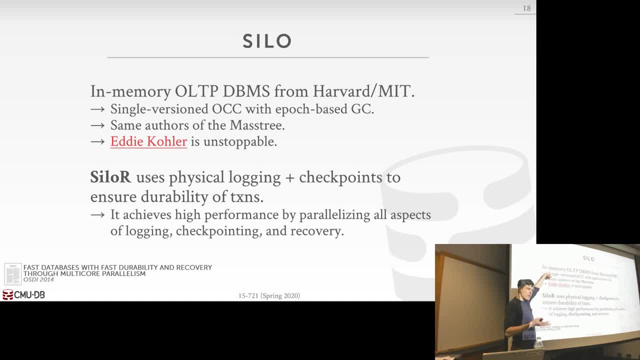 So this is Silo is the same people that developed the Mastree. They wrote Mastree first and then they built Silo around it. So the paper- This paper here- proposes a physical logging technique called Silo-R that is going to try to parallelize as much as possible all the logging checkpoint. 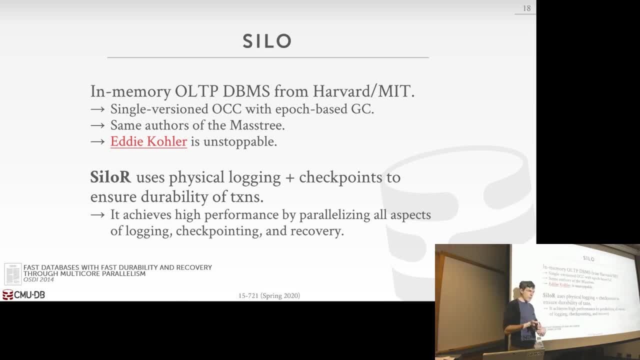 and recovery processes so that we get the best performance, And the way they're going to do this is that they're going to disaggregate the log across multiple files which could be stored on multiple disks and allow them to be read in parallel at the same time. 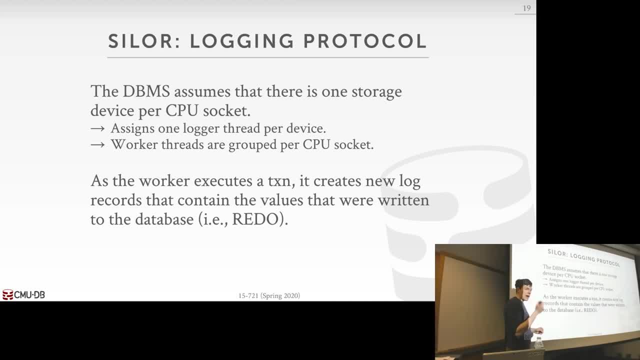 So the way this works is that for every single CPU socket in my system I'm going to have a dedicated logger thread and a dedicated log file, Right, And the idea here is that we want to localize all the memory writes we have to do to our local socket. 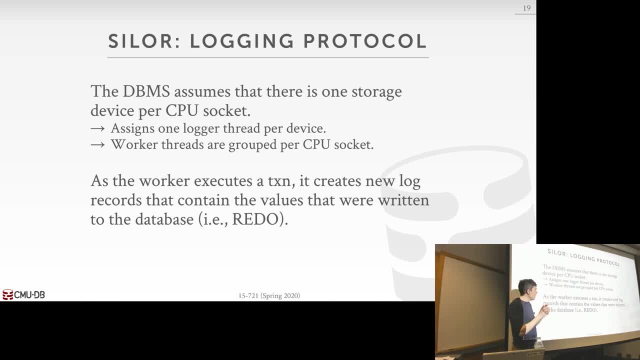 so we're never going over shared memory to another socket over the interconnect And then that way that log thread can be just pumping data out as fast as possible to the log file. So now, as transactions run, they're going to get a log buffer from their local logger thread. 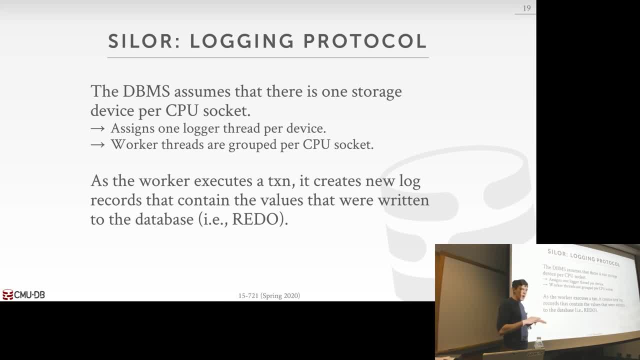 and then write out. just redo information Because they're in memory. we don't have to do any undo. And in this case, here they are. to make it simple, assume that all the logs- I assume that all the log records for a transaction- will be written out. 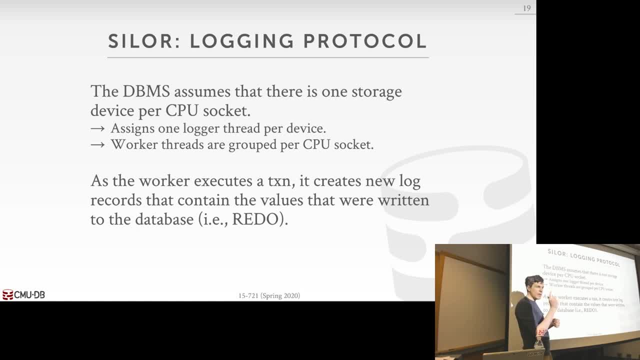 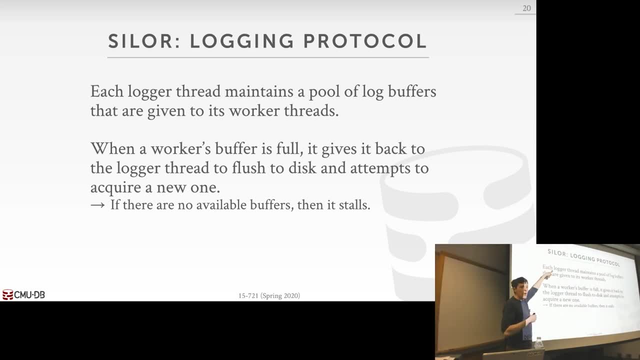 Actually in this case here you can do incremental, But in most cases it could be done all at once. All right, so again, I've already said some of this. So every logger thread is going to have a pool of log buffers. We hand them out to our local worker threads that are on the same socket as us. When my buffer gets full, I hand it back to my logger thread. The logger thread can then start writing out the disk, which means you can do incremental flushes. 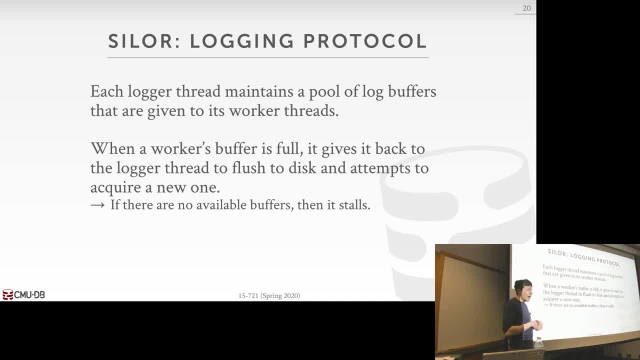 And then the worker thread tries to get a new log buffer. If there's no more log buffers available, then the worker thread has to stall until the logger thread comes back and says: you know, I flushed out enough, here's a new log thread or log buffer. 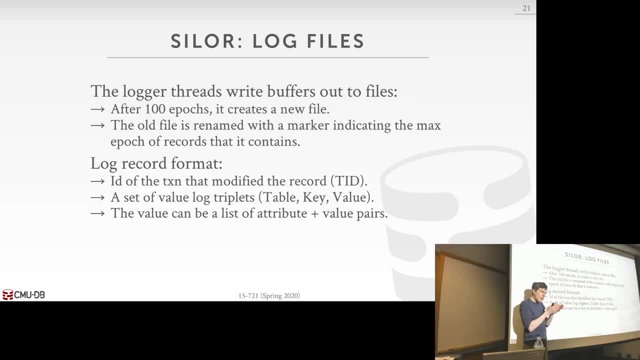 So now, what is going to happen, though, is that, because now our log file is broken up across multiple files on different disks, it may be the case our transaction might modify data that's managed by different CPU sockets, and therefore the log records for that transaction. 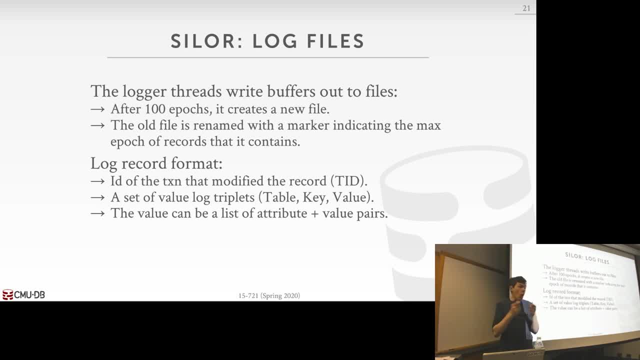 might be broken up across different disks, So I need a way to coordinate all of them so that I don't have you know, if I touch two log files, my transaction commits: the first log file gets flushed, but the second one doesn't. 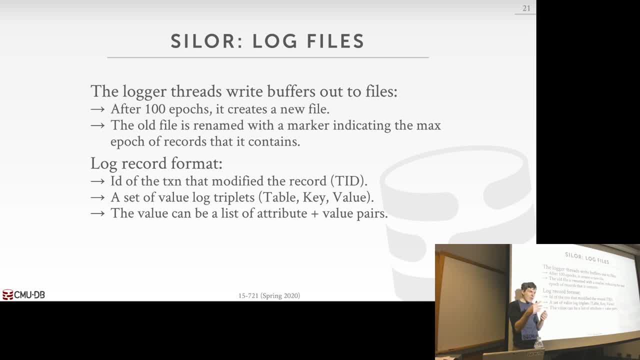 and then I tell the outside world that I crashed and I come back and now that you know, half the updates from the other log file never made it to disk. So you need a way to coordinate all of them so that you know that all the updates for a transaction have been safely flushed. 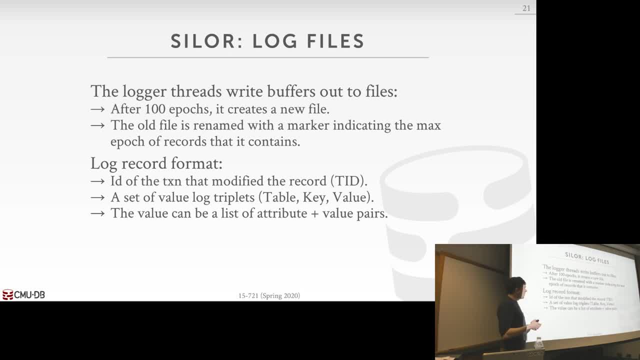 So this is what the epoch is going to do for us. So what's going to happen is, every so often, all the log this epoch will get incremented, and that forces every log thread to write out the current contents of the log buffer, and then we record what was the epoch. 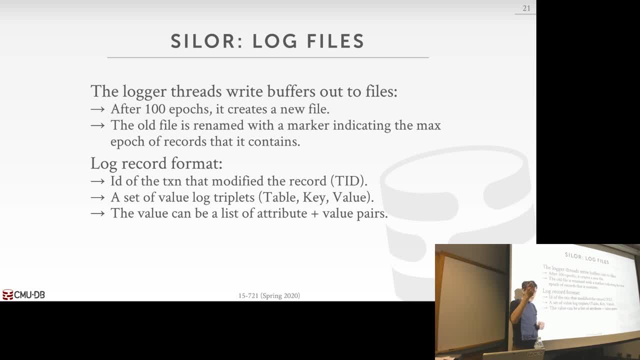 that everyone wrote at, and now we know that any transaction that has been committed and flushed to disk prior to that epoch is now durable and we can tell the outside world that we've committed. They're going to use this epoch and other ways of the system. 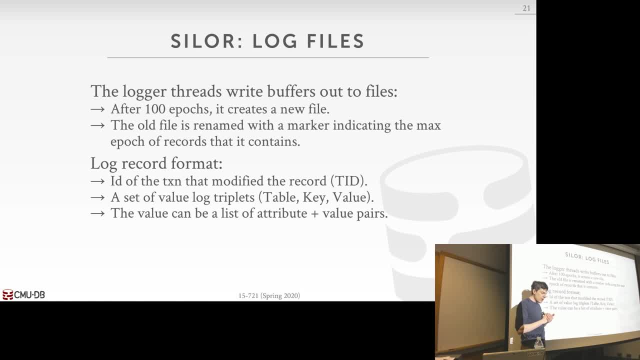 to minimize again coordination across different CPU sockets. but for our purposes here we can just focus on how we do it for logging. So our log records contain the ID of the transaction that modified a given tuple and silos are going to do serializable isolation. 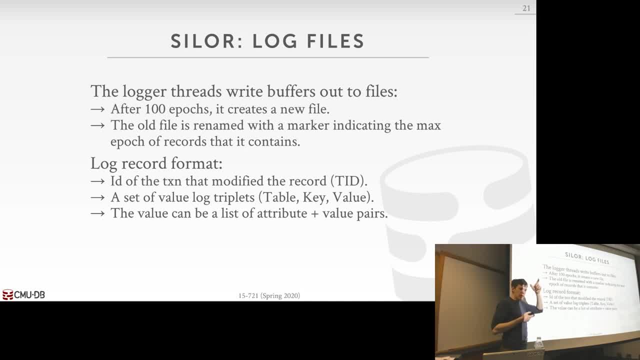 or serializable scheduling. so that means that the transaction ID will be enough to guarantee the correct ordering of the updates to the database. So if we just replay the log in the order of the transaction IDs, then that will put us back into the correct state. 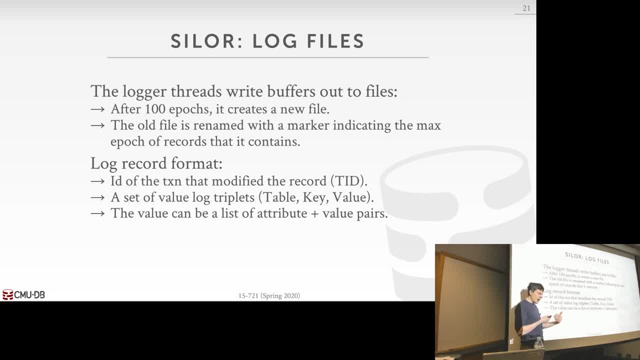 At lower isolation levels. you can't do this because I may update something and you may read something and update something else, and unless we have a log sequence number to order those things, we may come back and replay things in a different order. 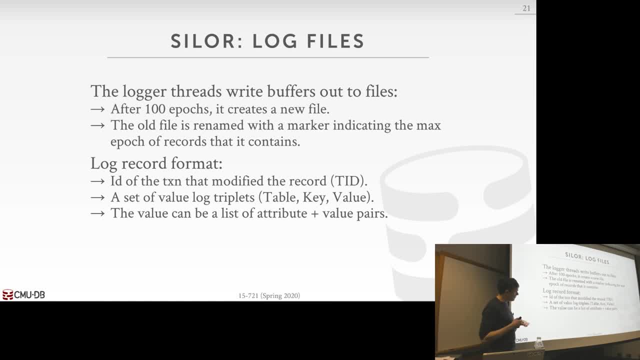 So by being serializable, we can guarantee that this will put it back to the correct state. Yes, Isn't that snapshot isolation if you assign the transaction ID at the start of your transaction? So isn't the snapshot isolation if you guarantee that the 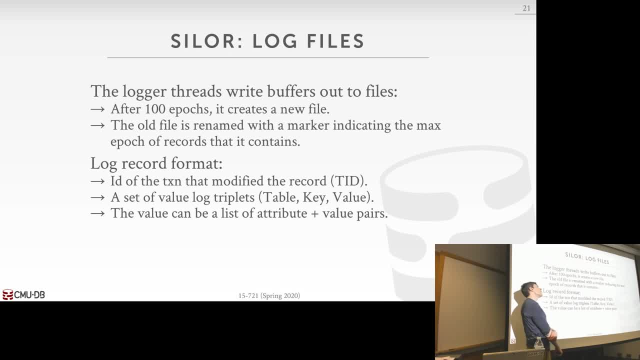 It's not necessarily serializable. Yeah, If the first writer wins, then that also solves that too. The main takeaway is that the transaction ID is enough to guarantee the ordering, to put you back in the correct state, and you don't need a separate log sequence number. 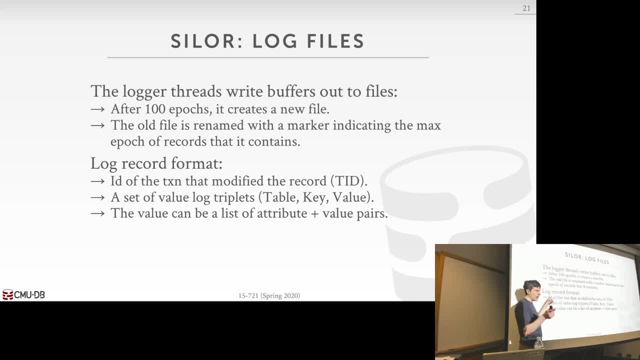 Because with a log sequence number, if an ID coordinated that across multiple sockets then that's a bottleneck. So the log file is going to be a triplet: just the table, the key and the value that gets modified and the value can just be the delta. 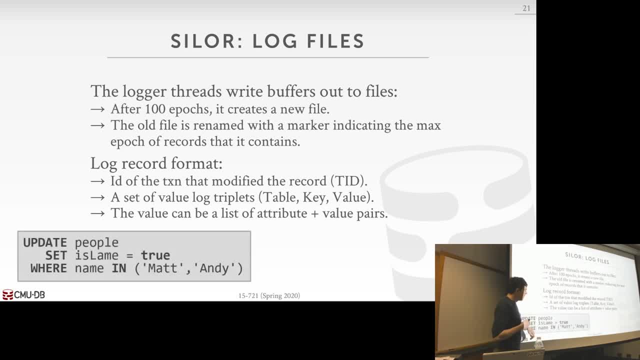 record of what the change actually was. So again, if I'm doing a simple query to update all the people that are lame with Matt and myself, then the log record will have a separate log record for every single tuple that this thing modified. 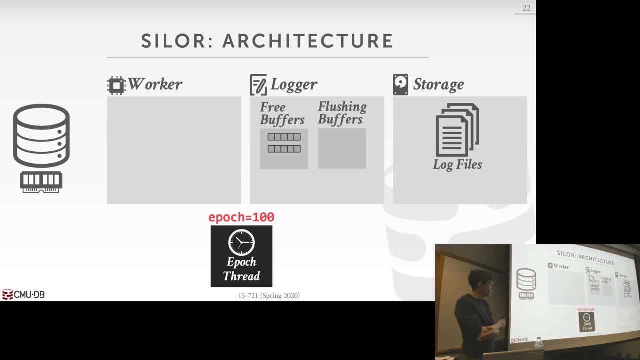 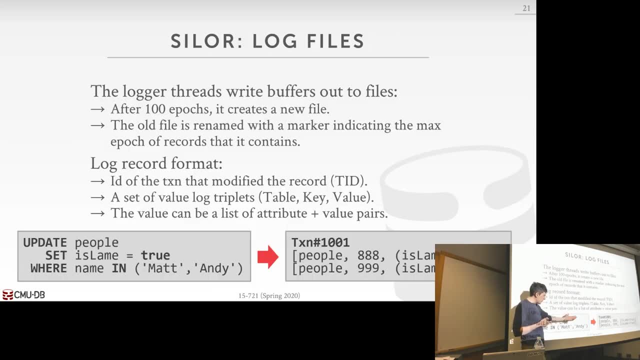 All right, All right. so here's the high-level architecture of the system, And again, the idea here is that I'm going to expose to you or show you that this is just physical logging, so there's nothing really novel being done here. 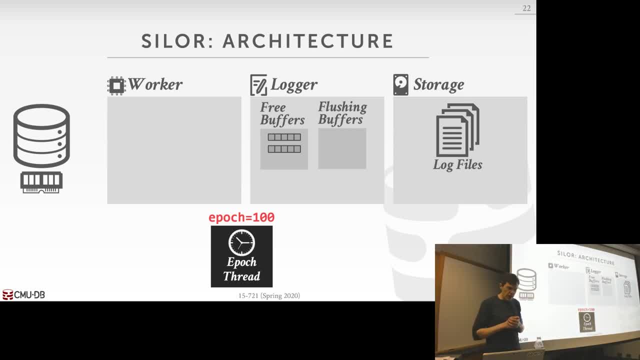 It's how they organize the system. that I think is actually quite interesting, and I haven't seen this in any other system. So again, the The transactions are going to update or the worker threads are going to execute transactions, So they're only going to execute these things as stored procedures. 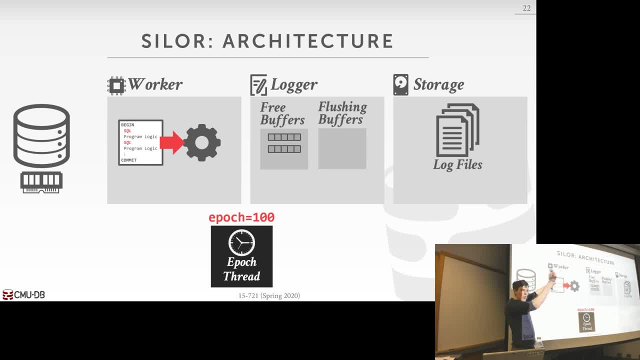 They call them one-stop transactions. But the basic idea is that we do a request like an RPC say, execute this transaction, and all the program logic of what that transaction is going to do is embed inside the system. So we never go back to the client. 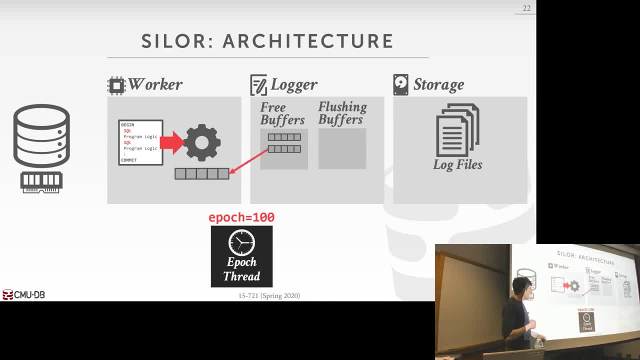 So everything is done in one invocation. So when a transaction starts running, the worker thread has to go to the logger and get a log buffer And once it has that it can start filling up the changes that it starts making to the database. 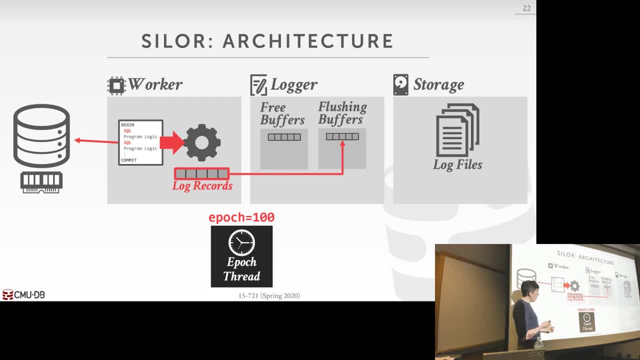 And at some point this log buffer will get full. so we hand it back to the logger thread and say: this thing's full, please flush it for us and we'll go ahead and get another log buffer. So then now at this point here, say that transaction's still running. 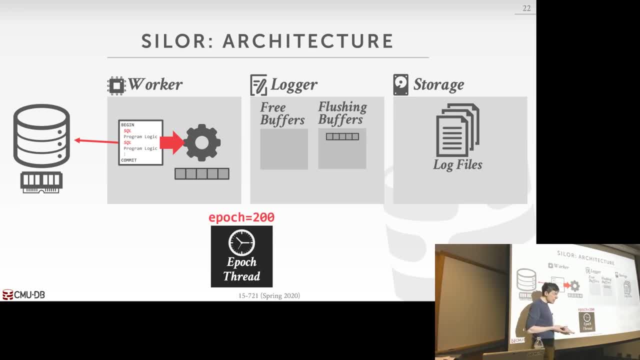 this other epoch thread waits up and says, all right, now, the new epoch is 200. So that's going to force all the logger threads in the system to now flush whatever buffers that they have, including any ones that were handed off before. 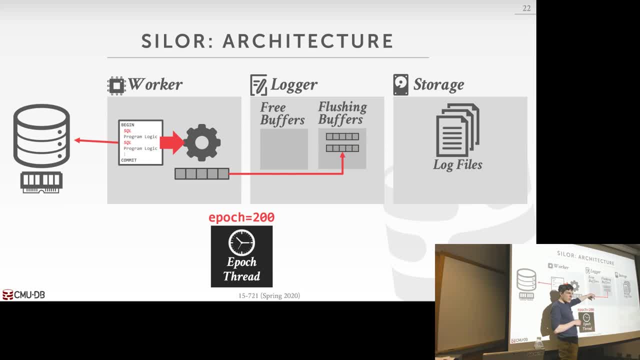 So now the worker thread has to go back to the system, It has to hand back the log buffer to the logging thread, and then it could keep on running. It could say: now give me another log buffer to start filling up, But in this case here there aren't any more, so it's going to have to stall and wait. 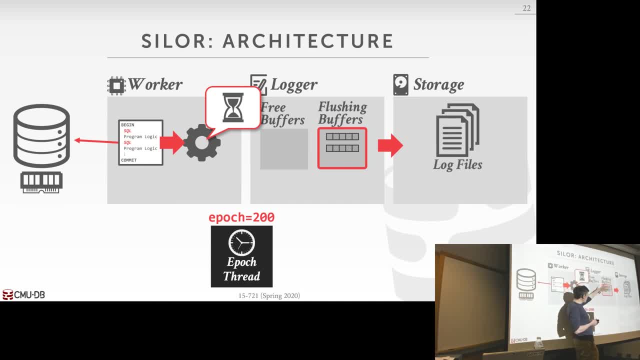 So now the logger thread can start flushing things out the disk right, And as it flushes them it frees up log space and then we can hand back the log buffers and let this guy keep on running. So in the most simplest world, assume every transaction will be finished within an epoch. 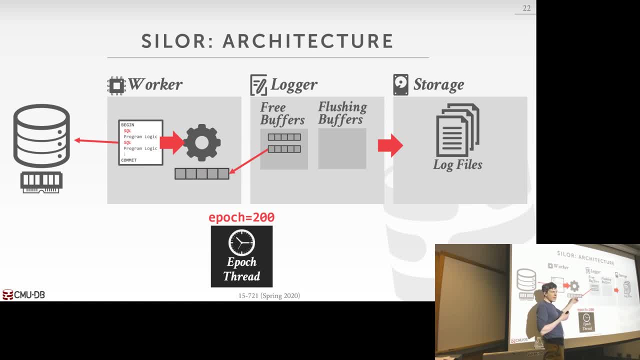 If it's spent, then it's going to have to wait. If it spans multiple epochs, then you basically have to keep track of. like this transaction was a round. It spans multiple epochs, so you have to go back further in the log to try to figure out what actually happened to it. 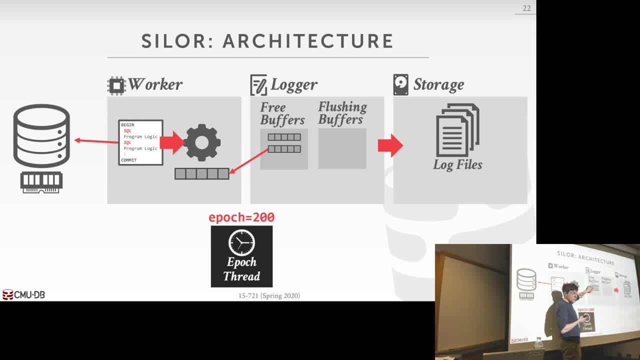 But the main idea here is that by having this back pressure mechanism where if we run out of log buffers we don't allocate more memory, we make this guy stall. that prevents us from generating log records faster than we can actually write them out the disk. 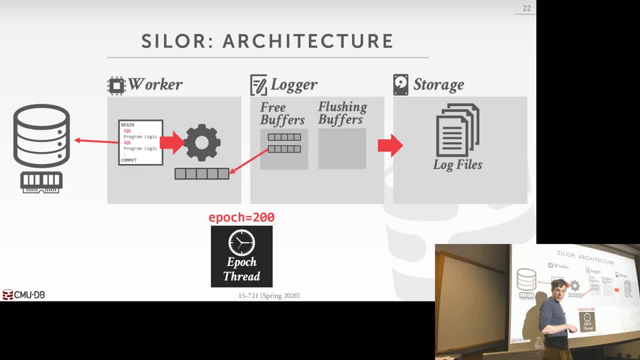 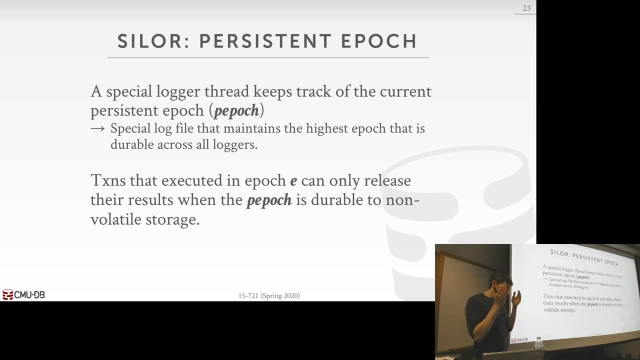 Because otherwise the log buffers will just grow infinitely and we'll run out of space. So let's talk about what this persistent epoch thing actually does. So every logger thread is going to have its own file where it records all the delta records that transactions are generating when they run. 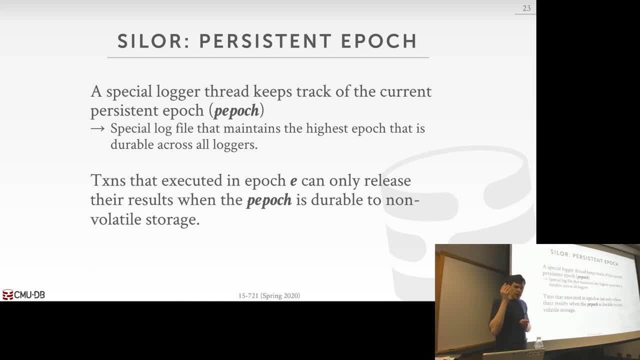 But then there's going to be a special log file where we keep track of the highest epoch that all logger threads have flushed out successfully to disk. Now everyone is flushing at the same time. when the epoch increments, you tell everyone to flush, Right. 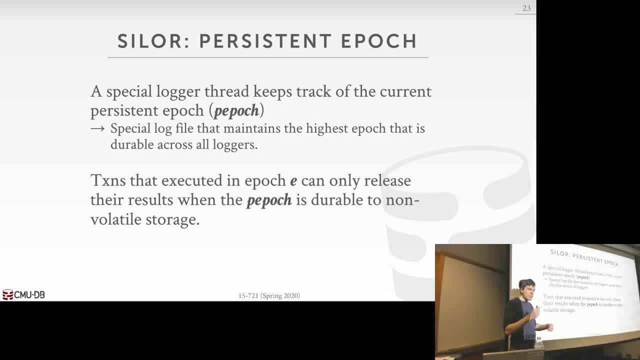 But then it may not all happen exactly at the same speed And only when everyone says: all right, I flushed it. then you go update and update the persistent epoch. Now you don't need this for correctness. This is actually just an optimization so that when you crash and come back you can just look at this one file and say, all right, what's the epoch I need to start with. 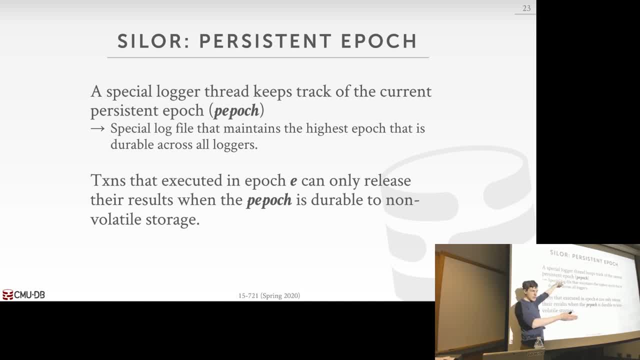 Otherwise you'd have to go look at every single file to figure out what's the intersection of the epoch across all of them. This is just an optimization. It's nice to have And the overhead of it is. It's somewhat small, other than an Fsync. 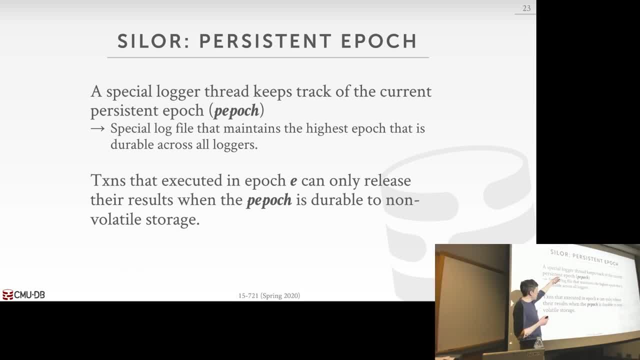 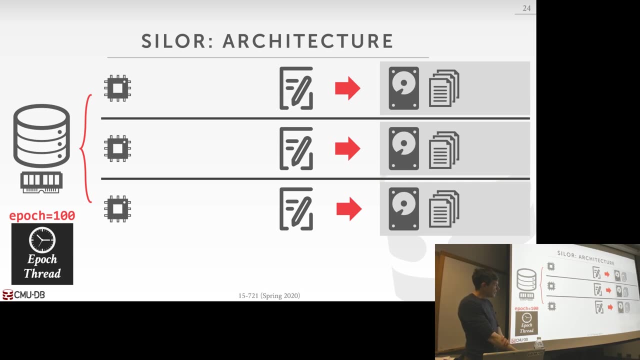 Okay. so we know that if this thing gets written out to disk, then we know that any transaction that executed in an epoch that's less than or equal to our persistent epoch we know is durable. So it looks like this: Say, we have now three logger threads and each have their own log file they're writing out to disk and each have a bunch of worker threads. 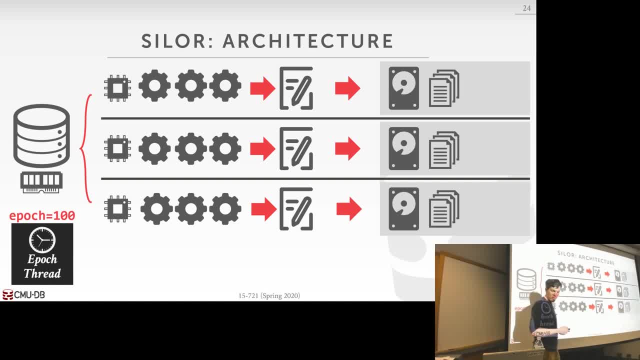 And again, these guys are just going and getting the log buffers from the logger threads And then you have this. now This is a special, persistent epoch thread that's going to update the file and disk Every so often. now the epoch changes. 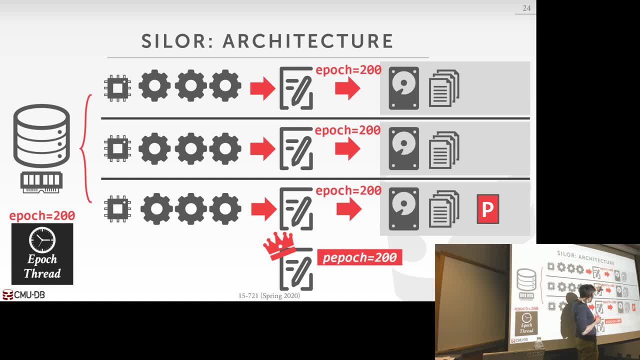 So everyone has to then flush out all the changes they have up to that epoch. Once they all then confirm with this epoch thread the persistent epoch thread that they've written out to disk, then we're allowed to go ahead and write out the persistent epoch file. 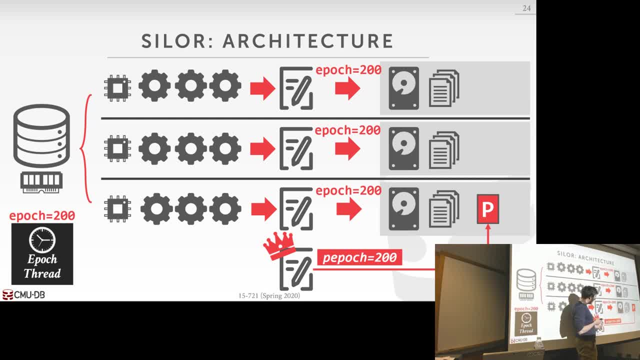 So for this one, like I said, you don't need this for correctness. This is just an optimization, So I don't think you actually need this to be Another fsync Like these. you want to fsync to know that you actually made the disk. 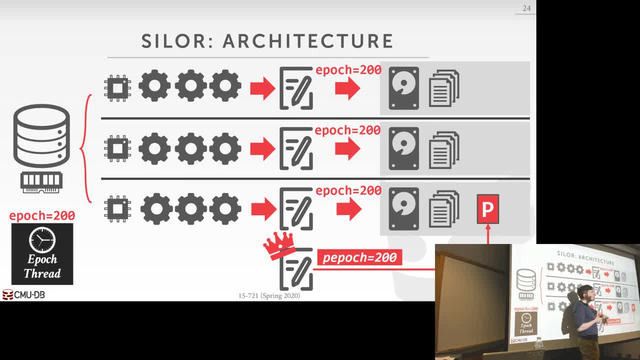 I think for this one, if you crash into the fsync now, you have to fsync. If you're going to rely on this to figure out what the intersection is of the epoch across all of them, then you have to fsync, right. 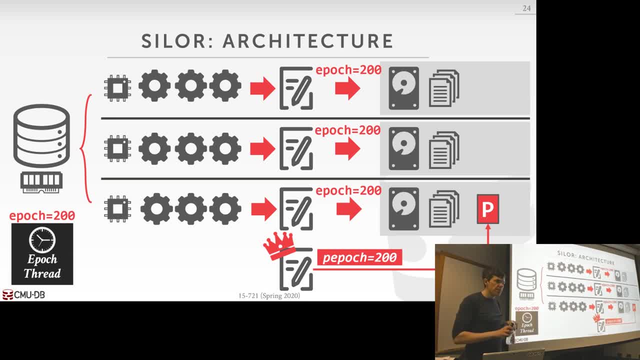 But that could be just another five milliseconds. Yes, So like at every 200, 300, are we also writing the pages out to this? Otherwise we'll have to start What pages? The in-memory pages? right, We are writing them and these are not checkpoints. 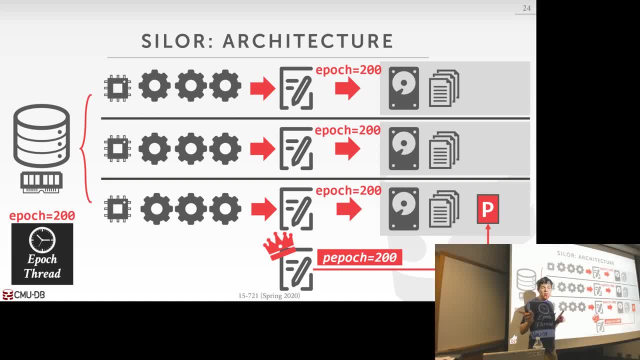 They're not checkpoints, These are just log records. Then we have to start from, like the starting thing again. Three more slides, We'll get the checkpoints. yes, But yes, this is what checkpoint solves. Yes, This is just again the architecture. here is how to do disk-aggregated log files across multiple disks. 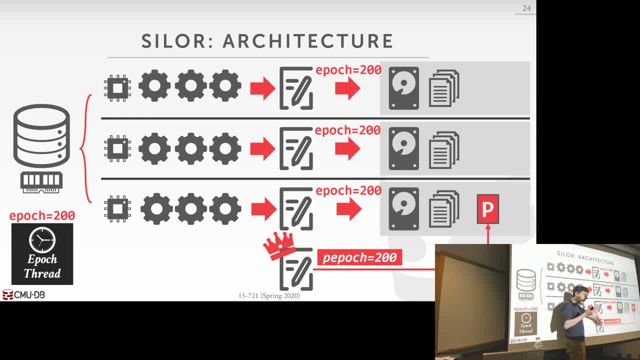 And you just have some sort of centralized location that you only update whenever this thing gets changed. In the silo paper they do this every 40 milliseconds. So in a real system this is problematic Because if you need sub-millisecond latency of your transactions, you're not going to be able to get that with this. 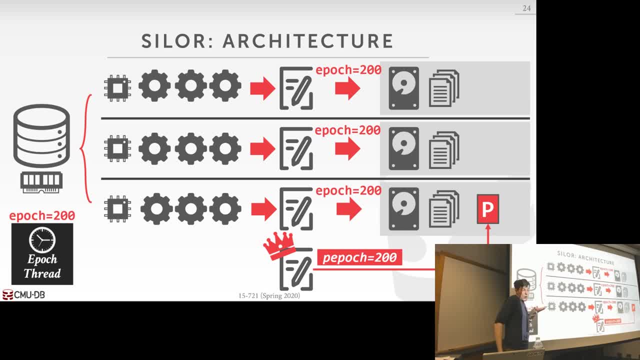 You have to crank this thing down. When I asked them why they picked 40 milliseconds, they just said this seemed like a decent number, right, So you could ratchet it down. so this thing gets updated every 10 milliseconds or 5 milliseconds. 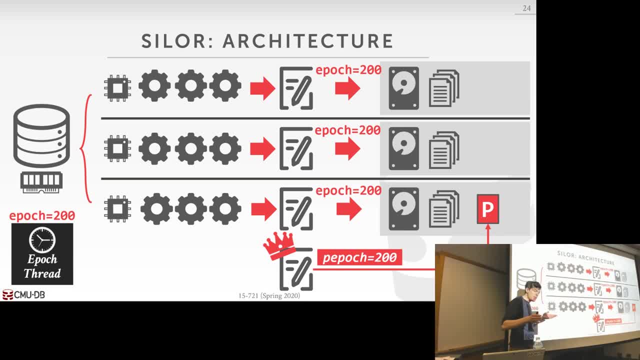 But now you're flushing a lot and this thing is getting written out a lot And you now could potentially have transactions that span multiple epochs And you have to do more stuff on recovery to handle this. All right, So now next slide, we get to your question. 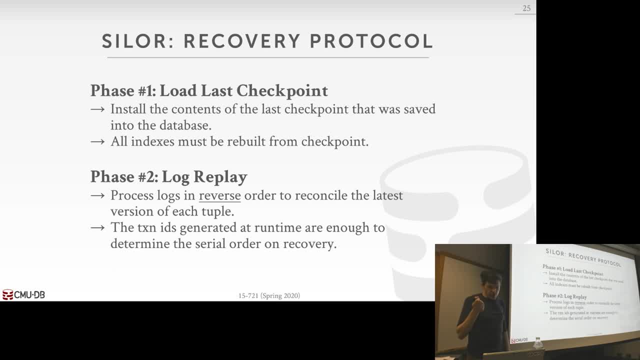 So we'll talk about checkpoints in a few more slides in more detail. But, as he said, if you don't have checkpoints then these log files grow forever And when I crash and restart I got to go back and potentially look at the entire log file. So every so often they're going to take a checkpoint And then when you, after a recovery, you load the last checkpoint in And that sort of bounds how much log file you have to look at And they're going to rebuild the indexes based on the checkpoint. 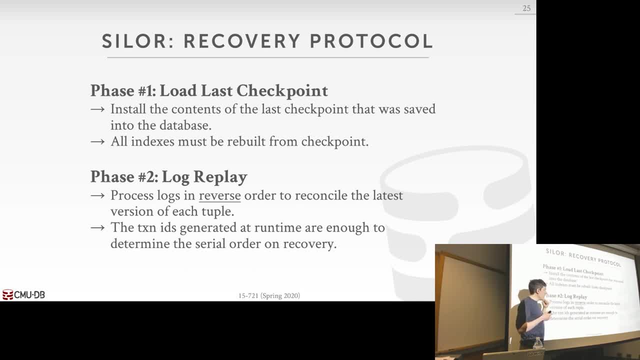 as I already said, because we're not going to make any log records for the indexes. Now, what is going to be different, though, than a disk-based system- which is super interesting- is that when they do recovery instead of doing in the redo phase, we saw with SQL Server. 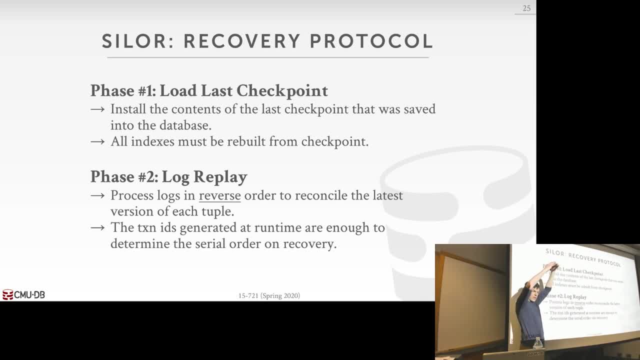 where they start at some point in the past and they process log records going forward in time. silos actually can start at the end of the log file and go in reverse order and start playing log records from newest to oldest, And again we can do this. That's because we're in memory, because we know that there's no dirty pages sitting around that got loaded in from the last checkpoint. So as we replay the log, we just need to know that what should be the final state of the database? 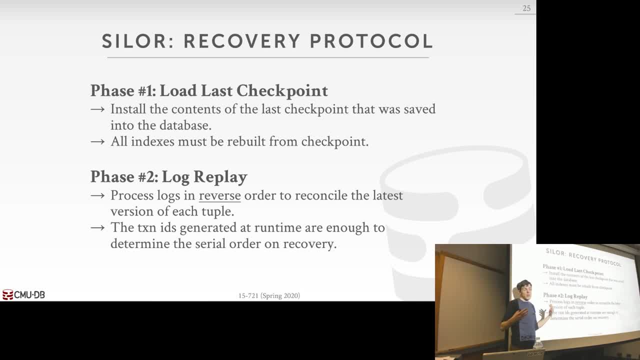 of a tuple in order for me to say the database has been restored. So if I have a tuple that's been updated 20 times, if I'm going in reverse order, I don't need to replay that log record for all those 20 updates. 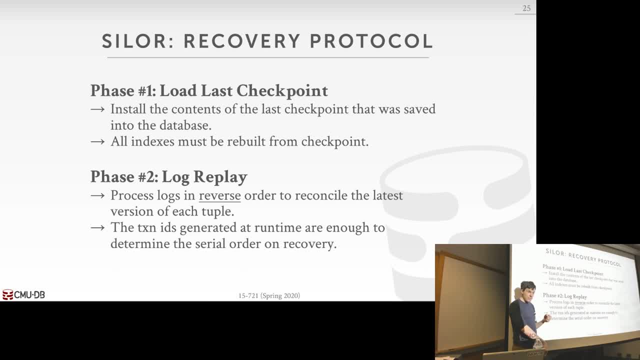 I just need to find the last update and apply that. That's totally different than as you would do this in a disk-oriented system because, again, dirty pages may have written a disk, so at some point I have to replay everything and then undo everything that shouldn't be around. 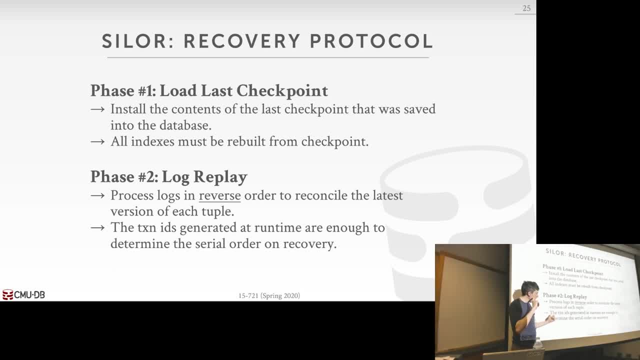 So what they're going to do again, they're going to keep track of the transaction IDs in every tuple to keep track of what was the timestamp of when this tuple got updated. So, as I'm replaying the log in reverse order, if I find a log record that has a timestamp that's smaller, 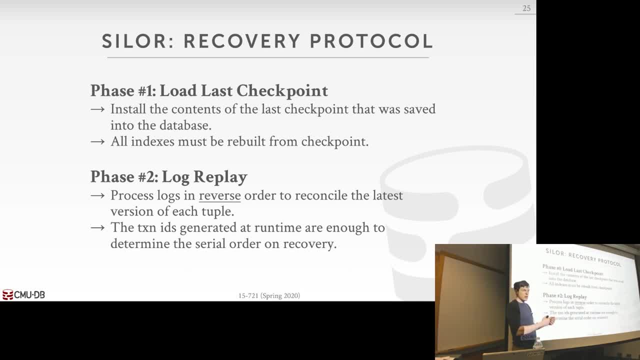 than the current time stamp, tuple's timestamp, meaning it was updated by a transaction in the future that I replayed earlier in the log. then I can just ignore that log record and I don't have to apply it. So it may be the case if I'm only updating a small number of tuples over and over again in my log. 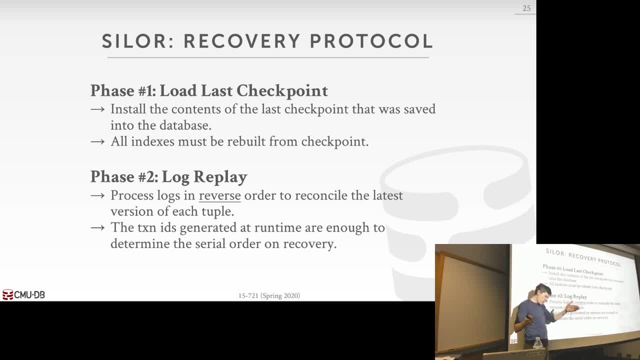 I may be able to realize that within maybe the first megabyte of log record data, I can ignore everything else after that. I still want to look at it, but I still don't have to replay it. Yes, This form work over here is not a simple version, right? 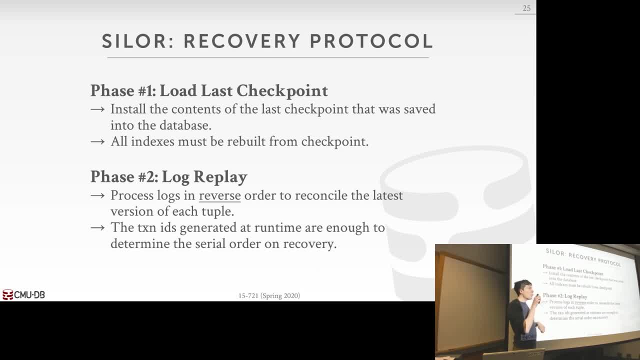 This question is: this won't work if it's not single versioned. If you don't need the old versions, then I think this is okay And so you could say: all right, well, if I don't need the old versions. 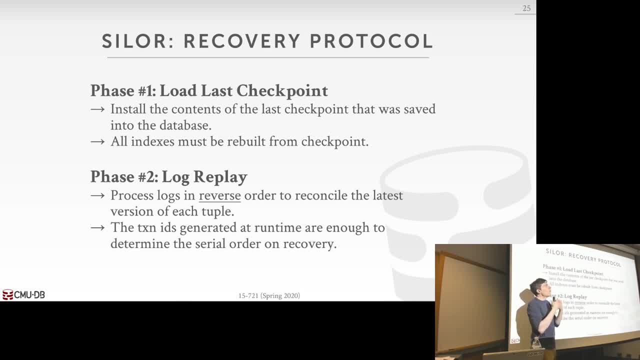 how do I say this? Well, one is no transaction. it's not like after a restart, any transaction that was running prior to the restart. it's not magically reappear when you come back. So there's no active transactions with timestamps that could possibly even read those things. So I could just ignore them. Now, if I'm trying to do audit logs or retain things to do time travel queries, then yes, I got to replay everything. then, yes, this won't work- I still need to redo everything. But if I don't care about it- I just care about what is the latest version- then this works. 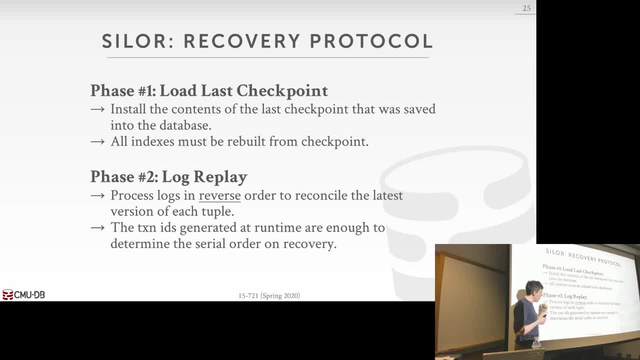 The reason why most systems don't do this is that when you do replication- which we'll talk about next class um- the replicas are essentially like in recovery mode and they're just replaying the log. So if you do it from oldest to newest, then the same mechanism you would do to do log replay is the same thing you can do for on the replicas. 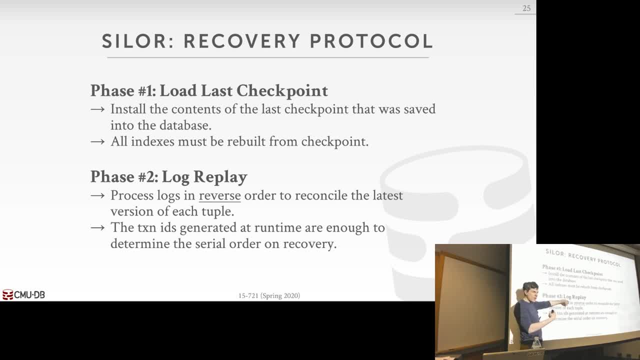 If, now, I have a specialized recovery mode where I can go reverse order, but only on the single node, then I have to have basically re-implement this twice. So Silo is the only system I know that does this. It's just. it's an interesting way to think about it, though, which I like. 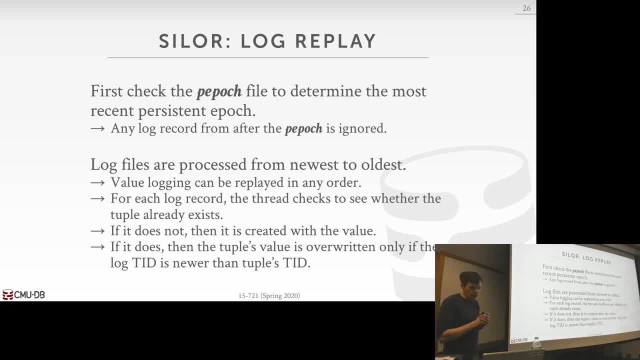 Okay, Okay, Uh, this one I think we've already talked about, right, So we go, uh, we go, look in the persistent epoch file, figure out what the most, uh, the most recent persistent epoch that was flushed to disk. 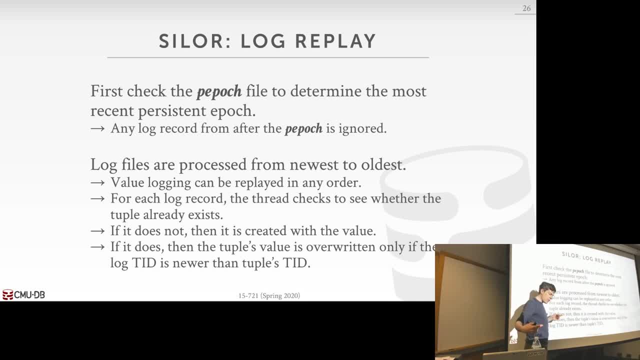 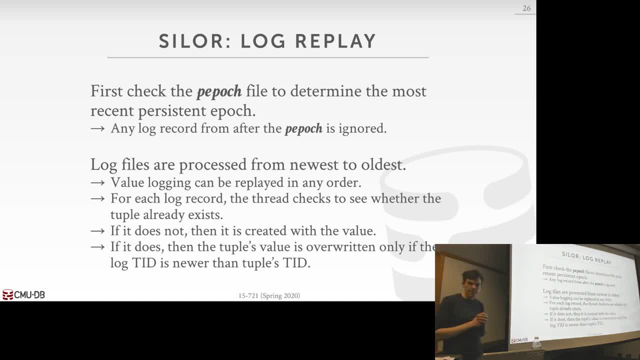 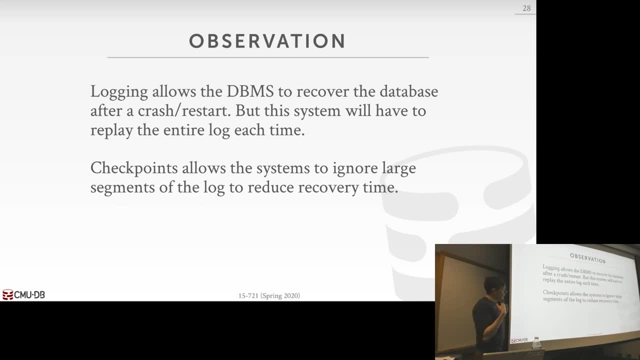 then I don't need to replay that log record. Okay, So now we also get to checkpoints in more detail. As we already said, the log file can grow forever, So that means that I potentially have to replay the entire log every single time I have to restart. 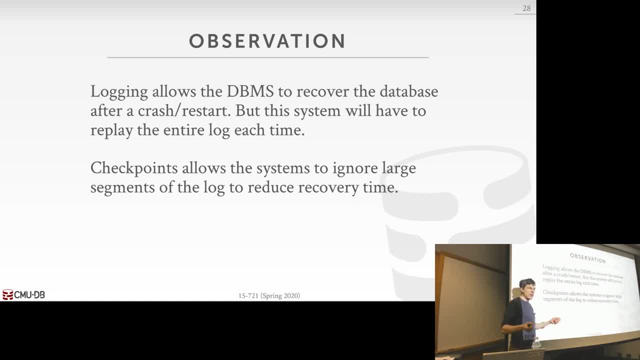 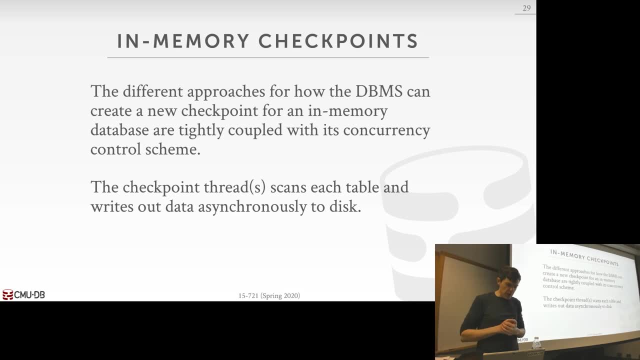 If I have a one year's worth of log without a checkpoint, then it potentially take me one year to restore the database, which is nonsense, like nobody could do this. So for an in-memory checkpoint, the different approaches we're going to choose are going to: 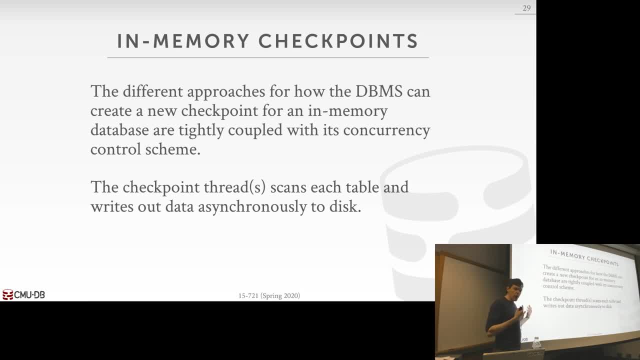 be tightly coupled with our concurrential scheme In some ways. if we're focusing on a multi-version systems, MVCC, then checkpoints essentially can become easy, depending on what we want the consistency level to be in our checkpoint, Because we just have a started transaction that takes a snapshot. 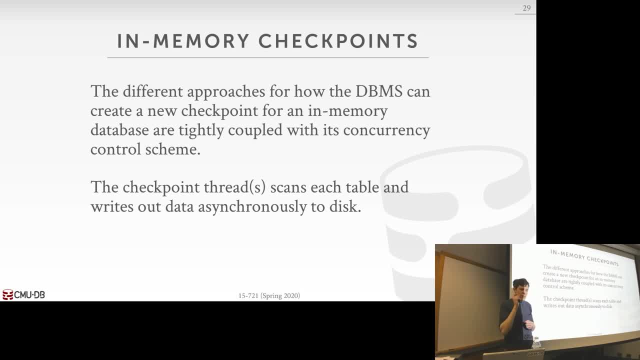 scans through a table and we just write out all the versions of the tuple that were visible to our snapshot and anything that is not visible to us meaning it came in the future we'll have the log records and we just replay those. all right, 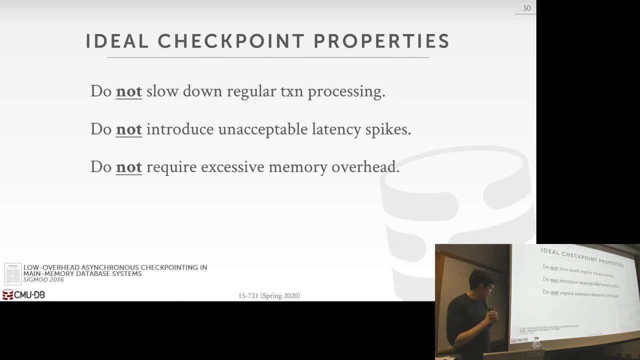 So there's a paper written by Dana Boddy, who did some early work on CommSource a few years ago in SIGBOD. He basically lays out what are the ideal properties you'd want for a checkpointing scheme in memory database. These seem obvious, but it's. 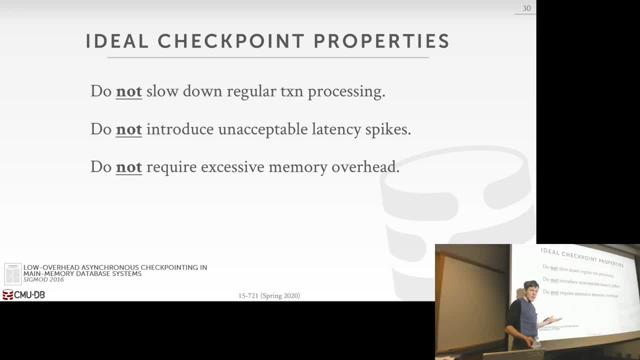 important to just keep these back of our mind. So obviously we don't want to slow down the regular transaction processing because it's not good if we can run really fast and also we take a checkpoint and now the speed of our system is cut in by half. 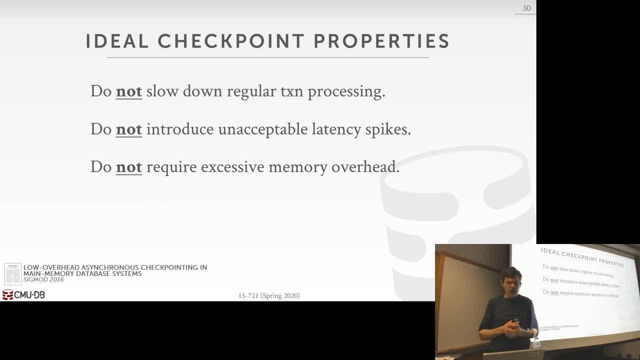 So the conventional wisdom for checkpointing schemes is that about a 10 to 15 percent overhead is considered acceptable. So every so often if I'm taking a checkpoint, if I get 10 percent slower, then people are okay with that. Likewise, you don't want any sort of huge latency spikes. 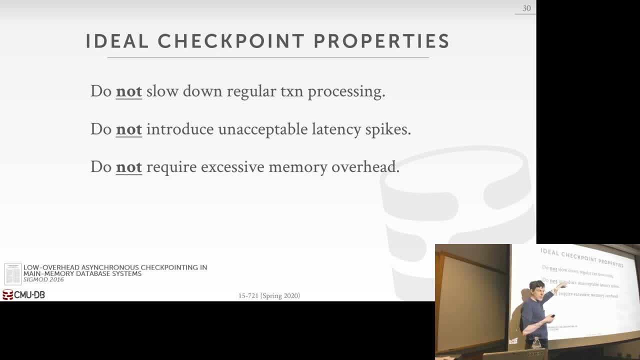 meaning I don't want a blocking checking scheme. I don't want to block the system or lock a table while I take the checkpoint and have all these transactions queue up behind this and then finally I release the lock and then they're allowed to run, because that's. 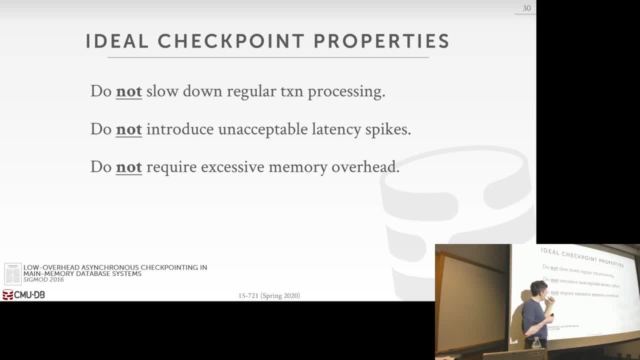 going to be a huge spike in our latency and people would pay attention to this. The last one, also too, is that we don't want to require any excessive memory overhead, meaning ideally we don't have to take a complete copy of the database in memory as we write down a checkpoint. 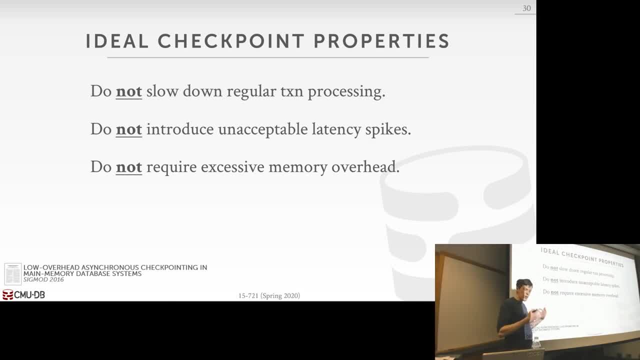 We want to be able to minimize that overhead because that puts pressure on our DIMMs and our memory bandwidth and our caches, So we reduce this as much as possible. So let's talk about the different properties you can have for a checkpoint, for an in-memory database. 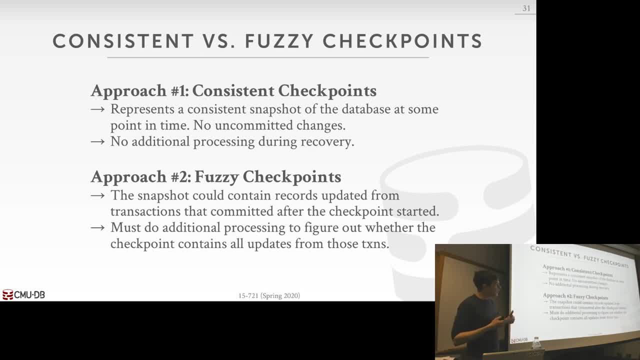 So this one here is. this idea here is very similar to what we talked about for disk-based systems last semester. So you have this notion of fuzzy versus consistent checkpoints. So a consistent checkpoint is when the snapshot of the database that's written to disk only. 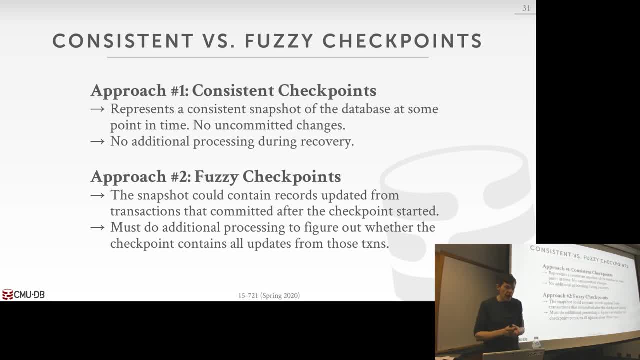 contains updates from transactions that committed. Again, think of just like under MVCC with snapshot isolation, the file I write to disk only contains the updates from transactions that committed before the transaction started. So now when I crash and restart, when I load the checkpoint in, 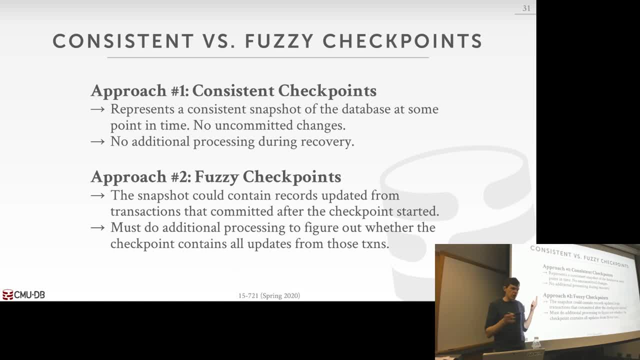 I don't have to worry about. does my checkpoint contain changes from uncommitted transactions? It only contains changes for committed transactions. So again, this is easy to do with MVCC. I run my query that scans the entire table and write it out. 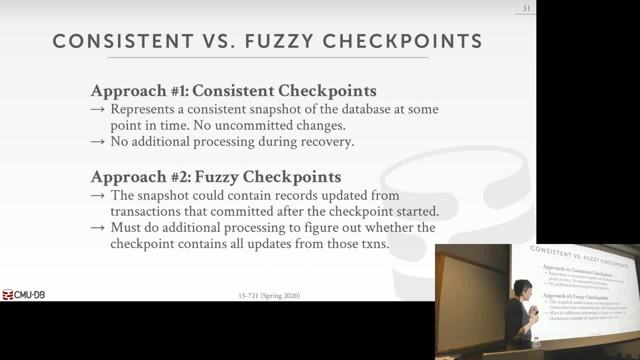 The other approach to do fuzzy checkpoints. well, this is where the snapshot could contain updates from transactions that committed after my checkpoint started. So my checkpoint starts running and I have a transaction that updates two tuples and say I scan through half the table. 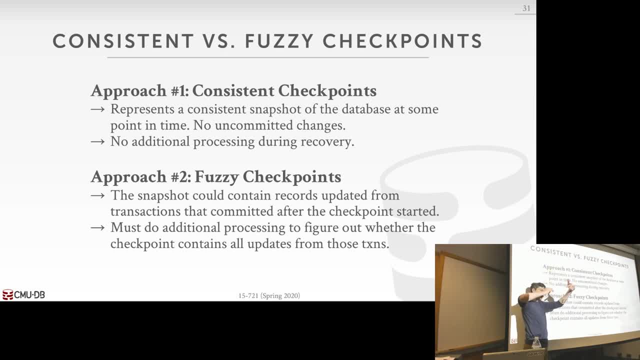 then the transaction updates a tuple I've already passed through, but a tuple I haven't passed through yet. My checkpoint now contains half the updates of that transaction. So now I have to do some extra stuff when I come back and recognize that. 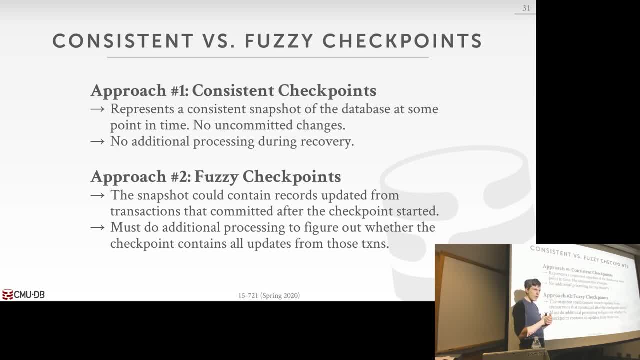 oh, there's an update that I may have missed, because this guy was running when I was running and I make sure I find the log records to reapply things correctly. So this is the easiest to do with MVCC. This one could potentially be faster and have less memory overhead. 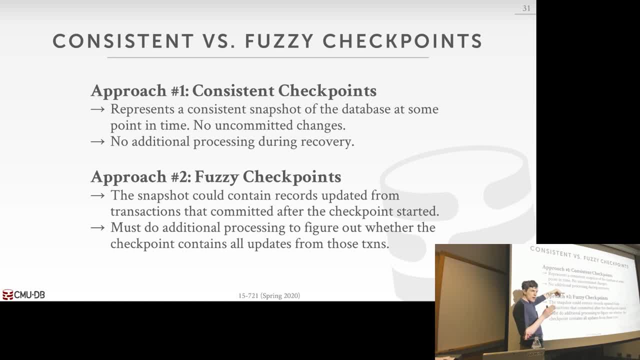 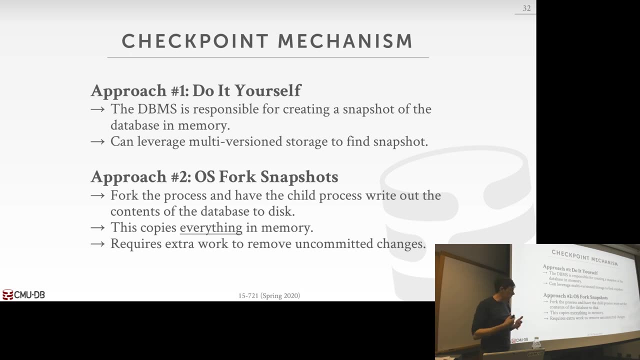 because now I don't have to worry about maintaining old versions and pausing the garbage collector. Most systems choose this. This one has advantages for storage overhead. The next is how we're actually going to do the checkpoint. So, as I already said, 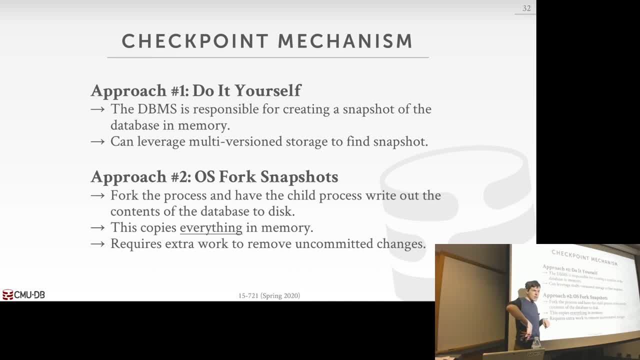 a do-it-yourself implementation of this would be just a sequential scan on the table and write out every single tuple that I find that's visible to me. Another approach is to do an OS fork, So this idea is interesting Because of an in-memory database. 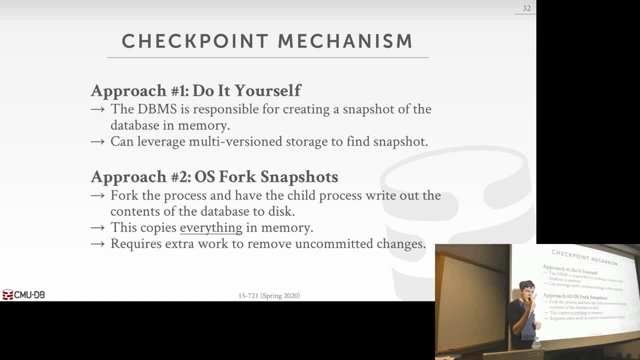 when we call fork in the operating system, what happens? We have a child process. What's in that child process memory? It's the exact same thing as the parent process. Yes question, Not like on-demand, right? It's on-demand, like you don't copy the entire thing. 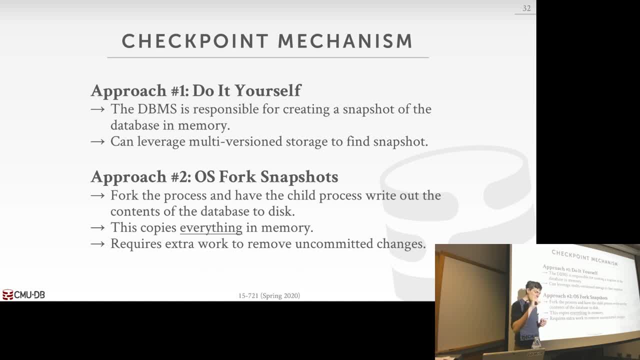 Correct. Yes, So the way it works is there's copy and write, So I call fork. The child process now has mapped in its virtual memory table all the same pages as the parent process. But if the parent process updates any of those pages, 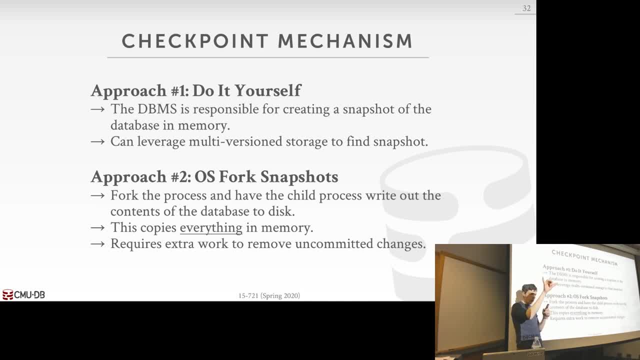 or if my child process updates any of those pages, then the OS will make a copy of it and remap it for your process. So as the parent process starts modifying in memory the database, the child process won't see this. So the only sort of well-known database system. 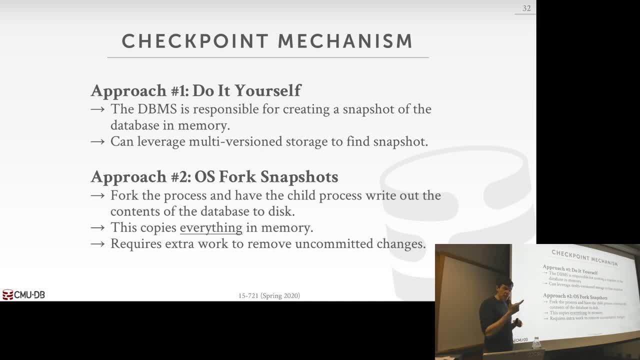 that actually does this approach is Redis. So this is how Redis takes checkpoints, And they can do this because they're single-threaded engine. So it is: pause transactions, do the fork and then now the child process has a consistent snapshot that it can start writing out the disk right. 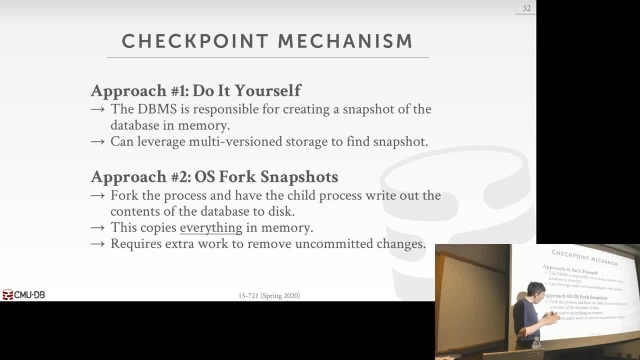 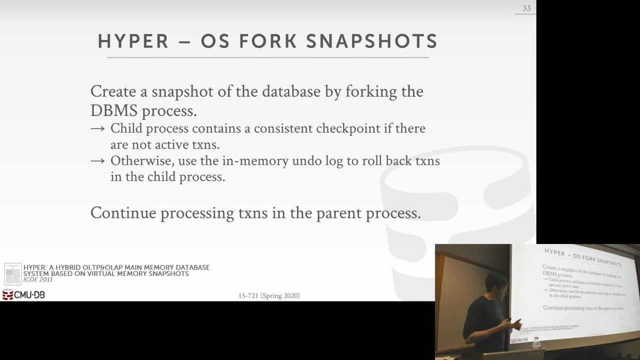 If you're not going to pause all transactions or updates while you do this, then in the child process you now need to reconcile the database to remove any uncommitted changes from transactions that were running at the time you forked. So Hyper actually did this back in the day. 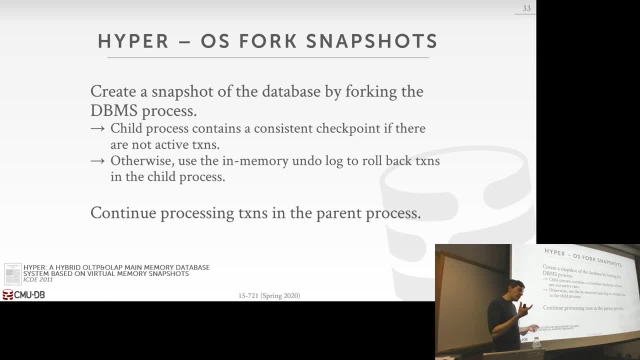 So this is a paper from 2011.. This is the first version of Hyper. It was actually influenced by a system that I was working on, or helped build HStore, which then became VaultDB, So they basically built their own version of VaultDB. 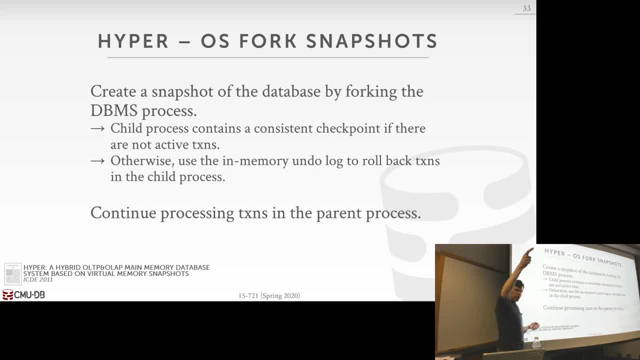 but they also wanted to do analytical queries. So they would do OS fork and then on the child process they could run analytical queries without slowing down the parent process that was running transactions Then they also could then take the child process and write out that checkpoint to disk. 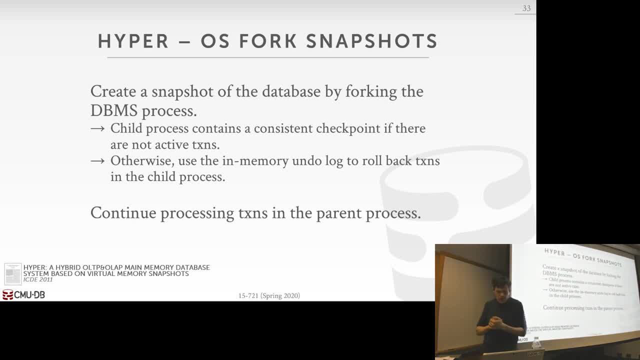 but again without slowing down the parent process execution, But because now, when they took the checkpoint or did the fork, there might have been some in-flight transactions that were running at the same time. they then in the child process. you need to look at the undo logs for those transactions which are in memory. 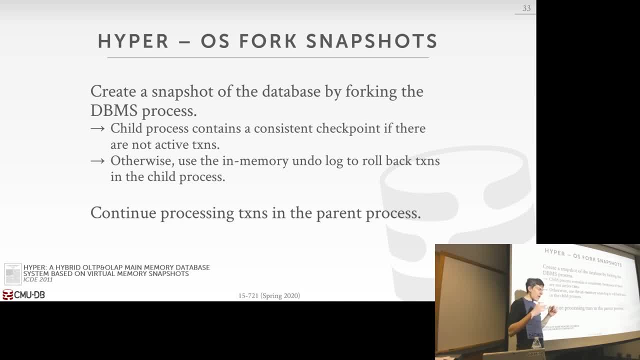 and make sure you reverse the database or reverse those changes so that again you have a consistent snapshot And then, after some period of time, either when the checkpoint was written to disk or when you're finished processing your analytical queries- they would kill the child process. 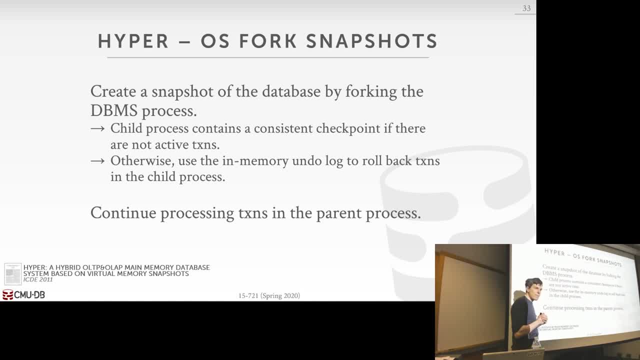 all the memory gets cleaned up, and then the parent would fork it again. So again, Redis is the only one that does this. It's easy to do because they're single-threaded. I don't know of any other system other than Hyper that has attempted this. 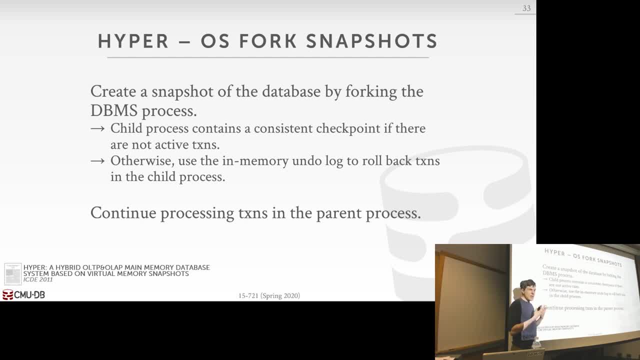 When we tried to do this in HStore, but we were based on the JVM. If you read the manual for the JVM it says don't fork it. We said, screw that and we forked it anyway. But it has all sorts of problems because you have a bunch of 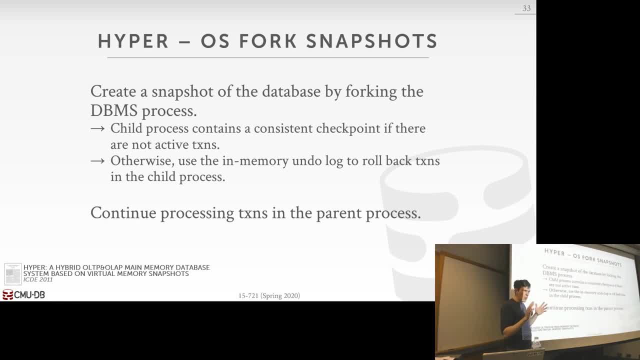 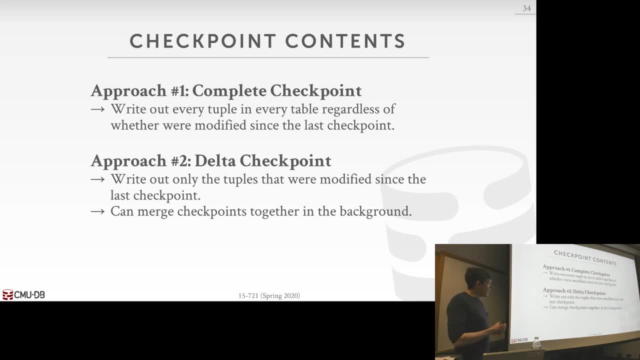 zombie threads because the garbage collector doesn't keep running again. Other background things don't run, So it would work, but it was a bad idea, Okay, The next issue is that: what are we actually going to store in our checkpoint? 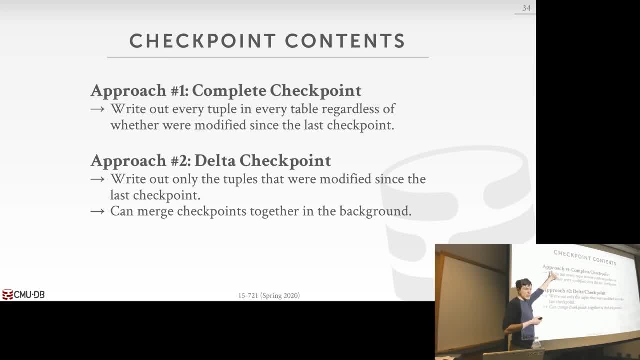 The two approaches are to complete checkpoints, the Delta checkpoints. Complete checkpoints is taking whatever is in my snapshot in my table or my tables in my database and just write that amount entirely out to disk. The Delta checkpoint is where you try to recognize what has changed since the last time I took 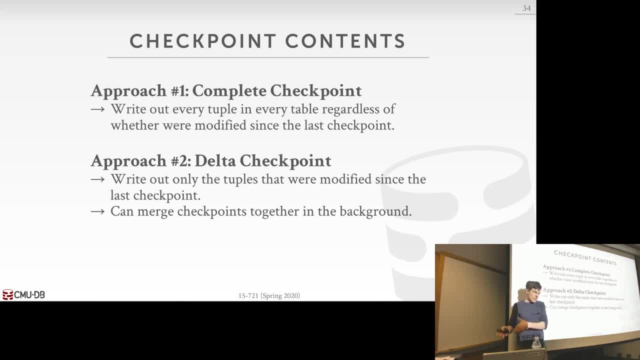 a checkpoint and only write out those updates. So most systems do this. The only system that I know that does Delta checkpoints is Hecatom, Because the issue is that with a complete checkpoint from a administrative management standpoint, I have this file now on disk that I can say. 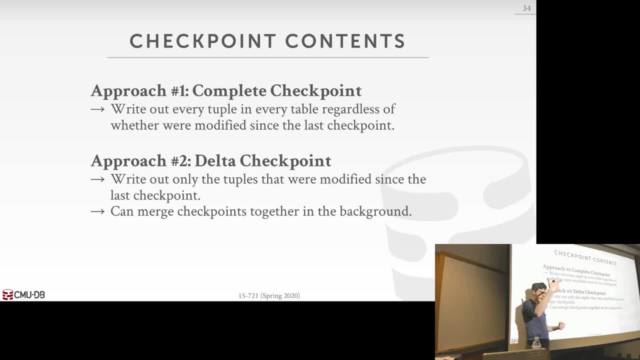 oh, this is my checkpoint. This is the exact snapshot of the database at this given time. With the Delta checkpoint, I need to retain a bunch of Deltas because there may be some updates that were in this snapshot but not the next snapshot. 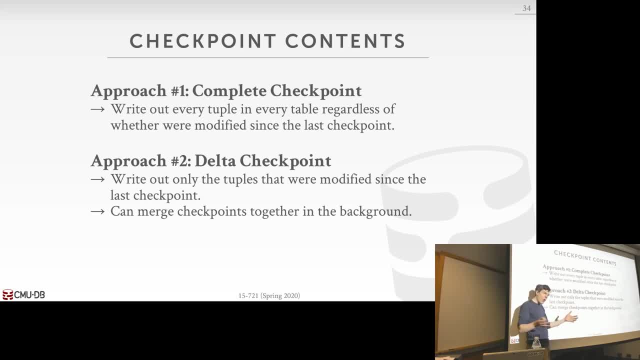 And in order for me to make sure I put the database back into the correct state, I need to have all of them. So when Hecatom does this, they have a background thread that will start coalescing, combining these Delta checkpoints to make it basically one giant complete checkpoint. 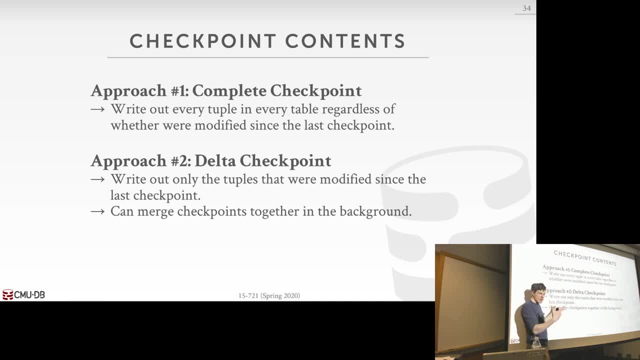 But you need to be mindful of this, of what the file contains that you're looking at. So this is easier to implement. It wastes more space, but from an engineering and management point, this one's better. One way to also to make this- not have a huge storage overhead. like if my database is one terabyte and then since the last checkpoint I only update one megabyte, this thing stores one megabyte. this stores one terabyte over and over again. If I store the data uncompressed on a file system that supports deduplication. 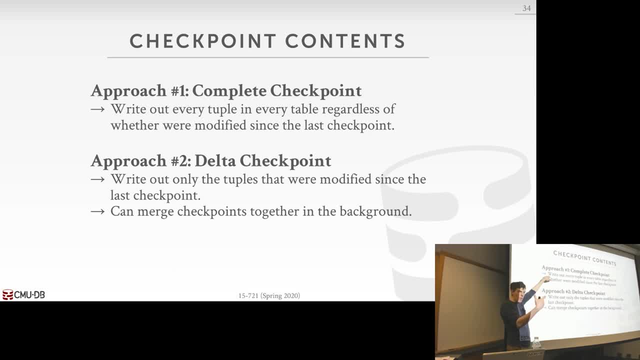 then the pages of memory that I write out are going to be duplicated over and over again and the file system could compress them down for me, So you can rely on things outside the database to make this thing actually tenable. All right, 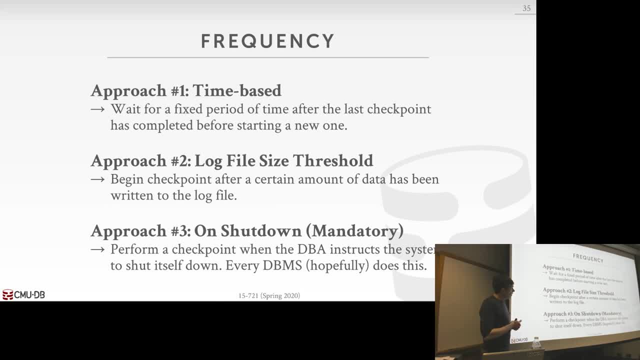 The last one is going to be the frequency of how often we're going to take a checkpoint. Again, we could just take a checkpoint all the time, but that could slow down the regular transaction workload. So typically what you do is either say: 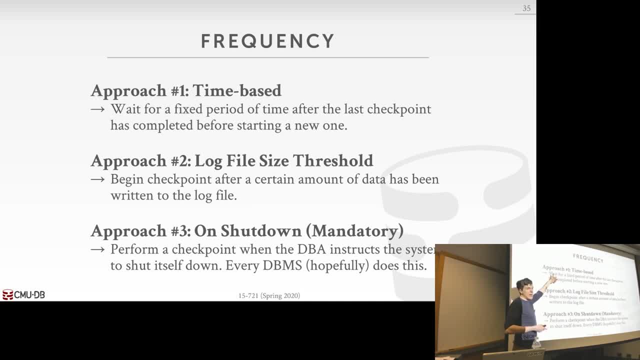 I'm going to fire off the checkpoint at a fixed interval, like every five minutes, or I fire off a checkpoint after I've written a certain amount of data to my log file, All right, So in this case here- this one- you can bound how much time it's going to take for you to recover. 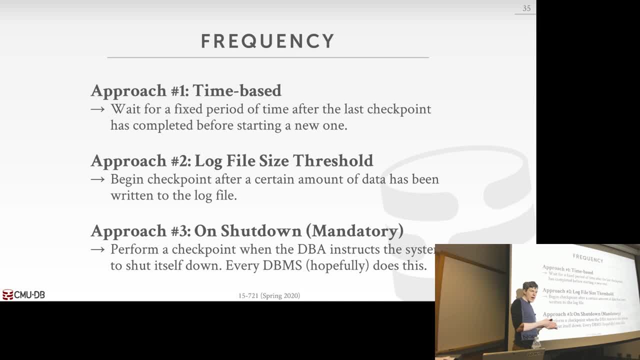 Say, if I crash I want my database to come back within five minutes so I can take a checkpoint every four minutes. So I know that when I crash I only have at most four minutes of log. I need to replay to put me back in the correct state. 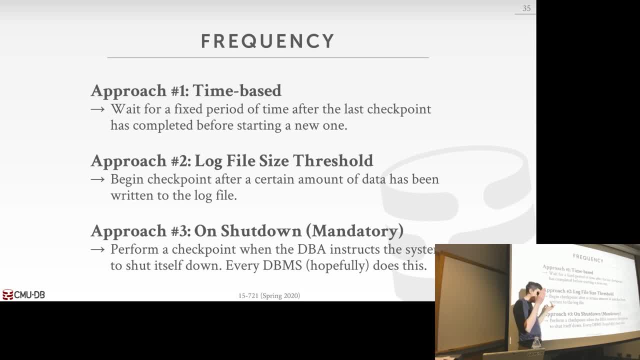 This one, you can do the math and figure out. oh, if I can replay the log at one megabyte per second, then if I set it so that I take a checkpoint after 100 megabytes, then I know I can recover in 100 seconds. 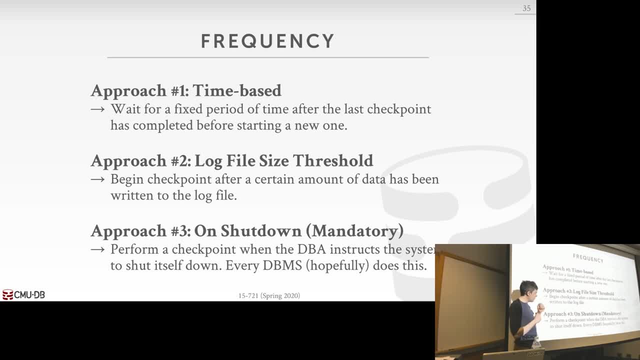 So they're essentially the same thing. It's just a different way to think about the problem. Again, some applications where you maybe don't care about things being super highly available within a single node- they can use replicas to hide all this. 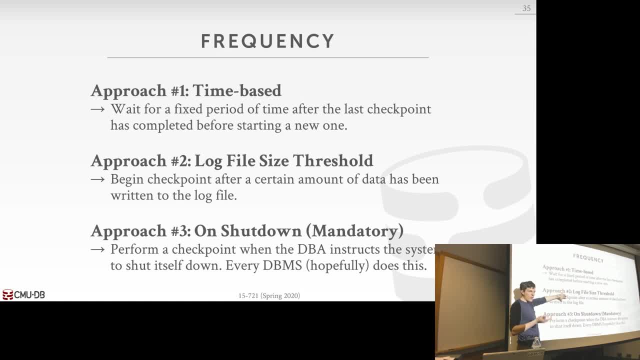 So maybe you take a checkpoint at longer intervals or longer follow-up sizes So that way if you have a replica, if the master crashes, the replica can come up without having to recover the log. We'll cover that on Wednesday. 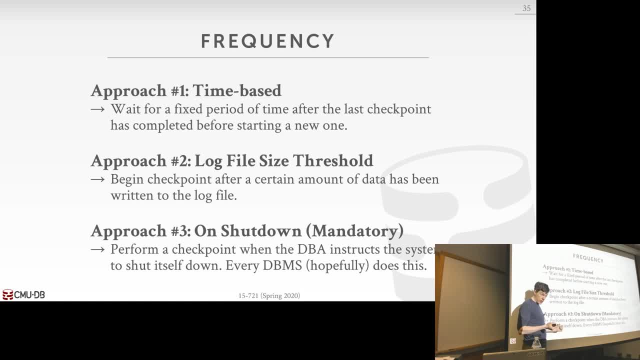 The other thing, though, that we need to do- which every system has to do- is that, if the data system is told, hey, we're going to shut down, then we want to take a checkpoint. at that moment in time, We acquiesce or stop all the worker threads. let them finish whatever transactions they're running and then take a complete snapshot, a complete checkpoint of the database. This is why you want to tell the database: hey, I want to shut down. just don't pass it kill-9 and do a hard sigterm. 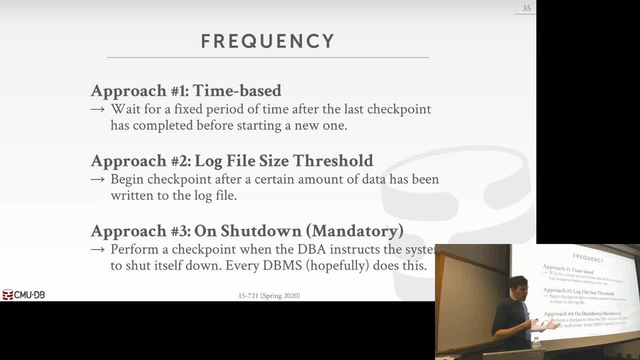 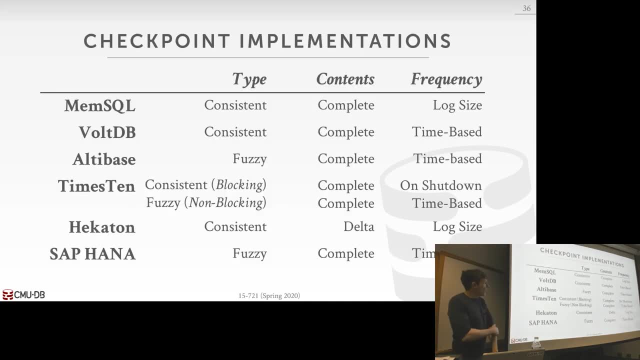 You want the database to be able to write things out gracefully, Because otherwise, if you do this, then you don't have to replay the log because you know the database is in the correct state. So this is just a quick summary of what some in-memory data systems actually do. 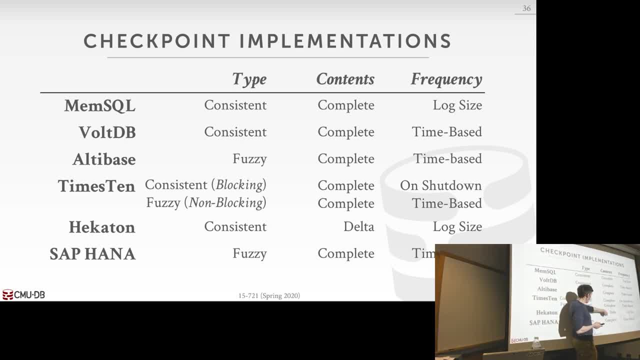 As I said, most systems, in terms of what they're actually going to store, are going to do complete checkpoints. Only Hecaton is doing the Delta one. Then what's interesting too is that some of the MVCC systems like Hecaton and MemSQL, 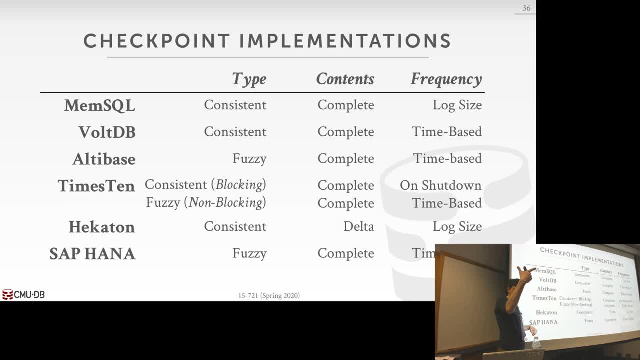 are doing consistent checkpoints again, which is just like snapshot isolation, just doing a scan, writing everything out. BoltDB is not an MVCC system, but they still can do consistent checkpoints, Because what happens is when you say I want to take a checkpoint, 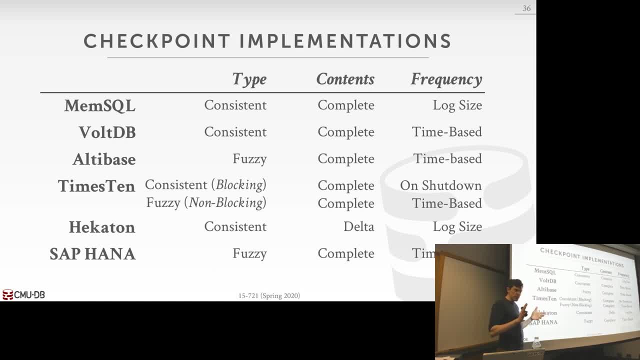 they switch into this sort of specialized two-version or multi-version system right, Where you just have the version of a tuple that existed at the checkpoint and then you just have another version. that's always the latest version. You don't really have version change. 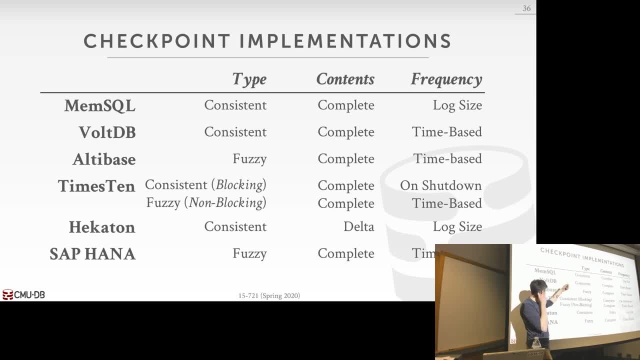 other than you only have two versions. So that's how they're able to do consistent checkpoints. AltaBase can actually do fuzzy N consistent checkpoints. I think they do the same thing on the x10, where, like if I'm shutting down. 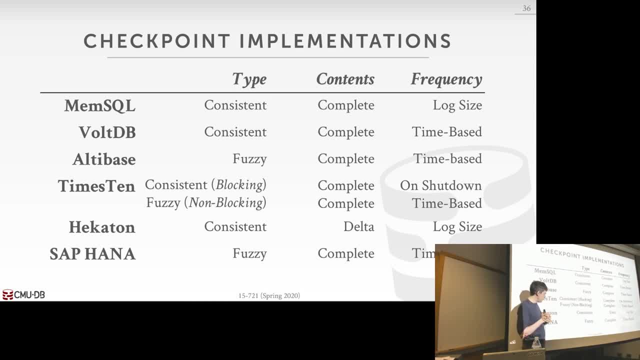 I'll do a consistent blocking checkpoint, but otherwise I'd normally take a fuzzy checkpoint Right And HANA does fuzzy with time-based. So again, different database systems do different things. If you're doing MVCC, then my opinion. 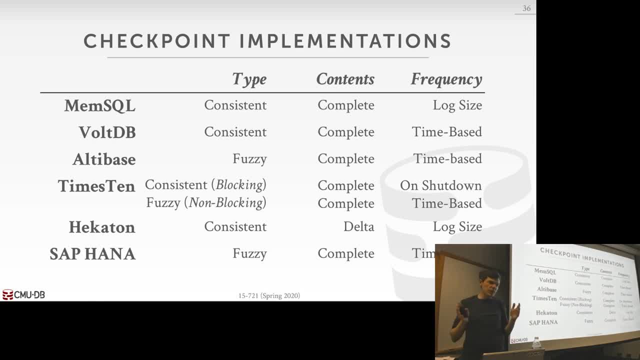 doing the consistent checkpoint and taking a complete snapshot is the way to go, Because there's less engineering overhead of figuring out what to actually write out. You just scan through and write everything. So any questions about checkpoints? Again, after restart I load the checkpoint in. 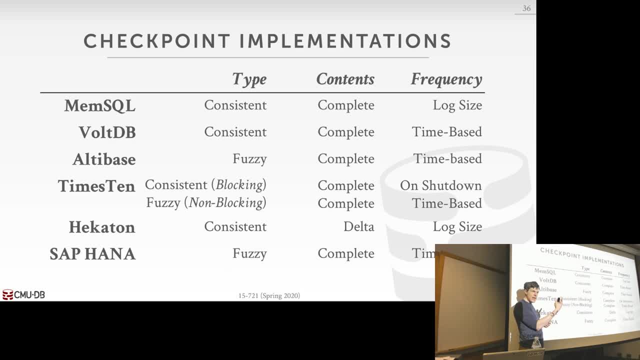 And as I scan the checkpoint, I'm copying data into my tables And as I do that- it's essentially like an insert- I update any indexes that are on that table so that they get populated correctly, And then, once all that's done, 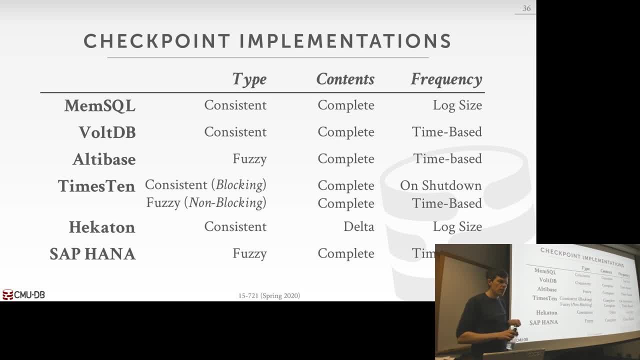 now the database is back online. Yes, The fourth thing: indexes also get copyrighted. So the question is: with the fourth thing, the indexes already get copyrighted. It depends on implementation. You don't have to, Why a fourth will copy something. 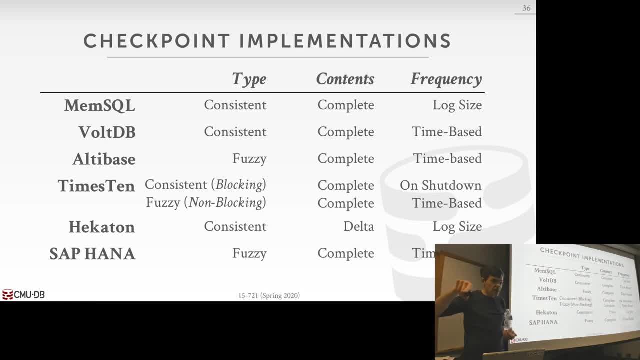 What do you want to write? Yeah, so fourth: yes, All the indexes get copied. What do you want to write? But you don't have to write it? All right, It's probably again. it's a waste of space. 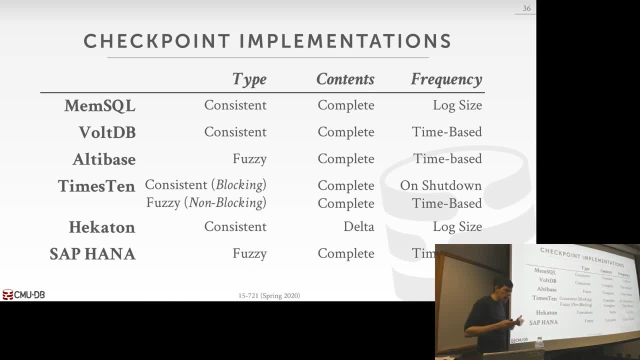 My indexes are huge. It's not worth it that this guy ought to write that out if I'm gonna repopulate it anyway. on recovery, Right, It's a trade-off between computation and storage, All right. so the last thing I wanna talk about very quickly. 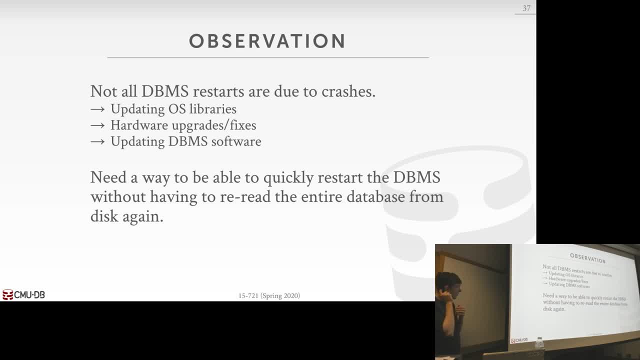 is how to do fast restarts. So everything I've talked about so far, the crash recovery for Silo and SQL Server and all the checkpoint stuff- this is assumed that, oh well, our system was operating, our system was running, something happened. 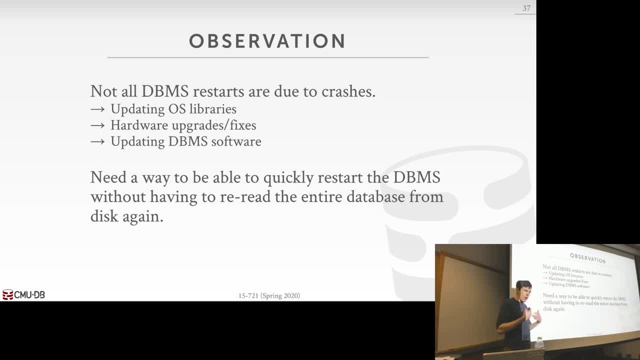 somebody tripped over the power cord, lightning struck the data center and we did a hard crash. It was unexpected, right, But there's other times we actually may need to restart the database system where it's not gonna be from a crash. All right. Very commonly maybe, we have to update our OS libraries. There's a technique in Linux called ksplice that allows you to update kernels without having to restart the system. But let's say you can't always do that. Sometimes you have to restart the whole OS. 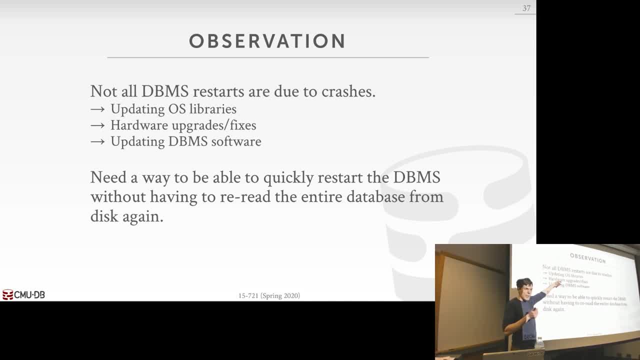 Certainly if you're gonna upgrade the hardware. some disks are swappable, but DIMMs I don't think are Like you have to turn the system off, put the new DIMMs in, or certainly if you're moving to another AWS instance. 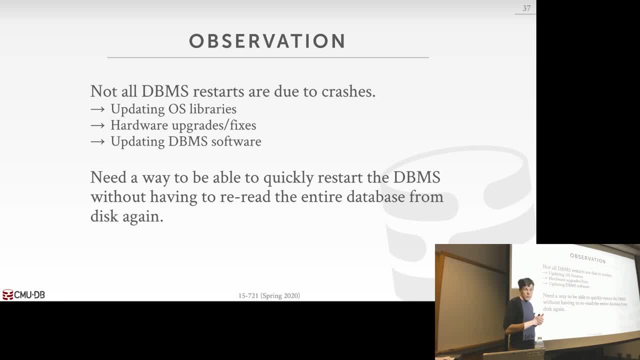 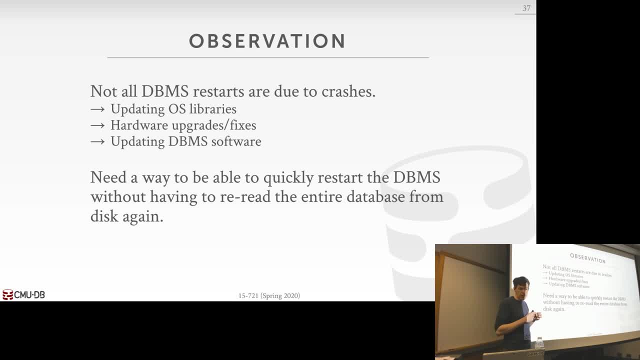 Again, Oracle has a lot of software. Again, Oracle has techniques that allow you to do patching without taking everything offline. but most systems don't have that. So let's say we wanna do this one here, Assume these ones here, we have to restart. 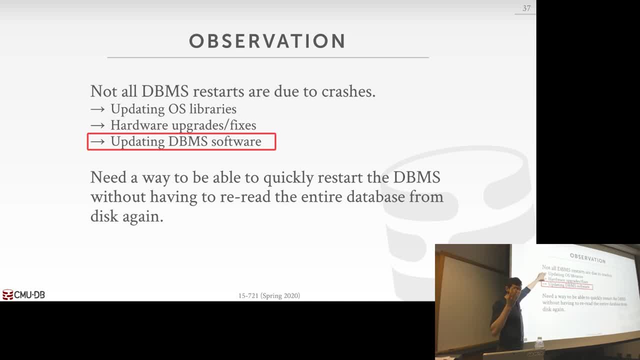 There's no way to get around this Right and restart the entire box For this one. here, though, we don't have to restart the OS, We don't have to restart the hardware, So it'd be interesting to see a way. 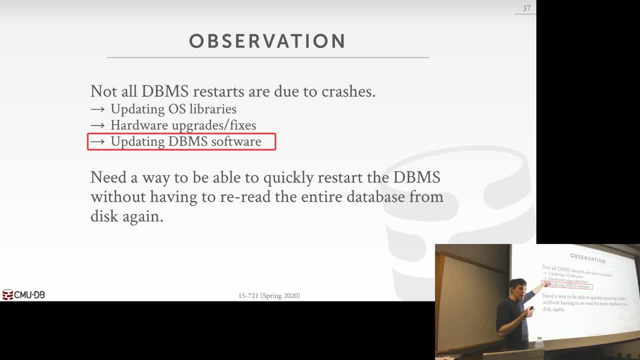 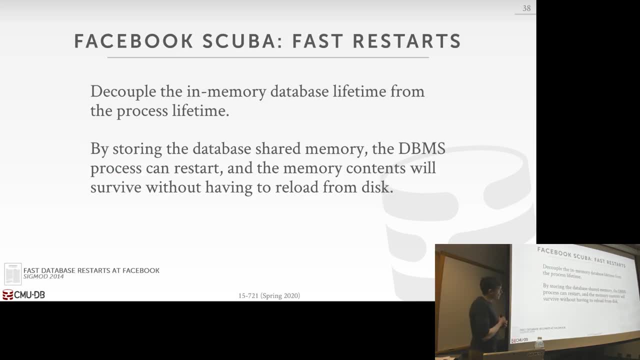 if we can restart the system for our in-memory database and not have to flush a checkpoint out the disk and then load it all back in over and over again. So this is what Facebook can do in their Scuba system. So I'll briefly talk about what Scuba is in a second. 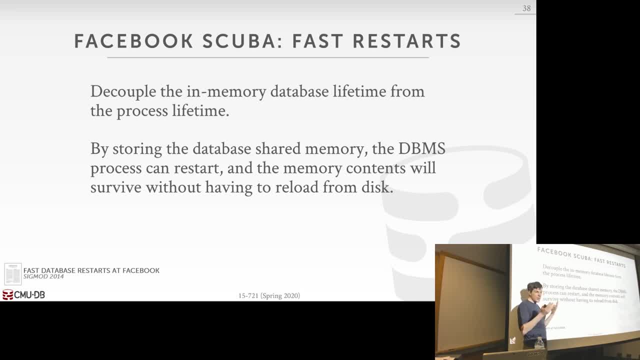 but if you remember from the introduction class, we spent a whole. this is what the students voted for. the most interesting system that they wanted me to talk about, So Scuba, is a. it's a distributed in-memory OLAP system developed at Facebook to do event log processing. 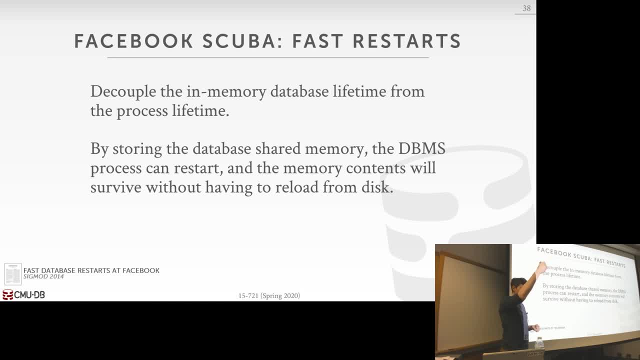 So whenever you load a page in Facebook, they're gonna- they're gonna keep track of what every single stage, every single service it touches for that request, record all that information and then dump it off to Scuba so you can do analytics. 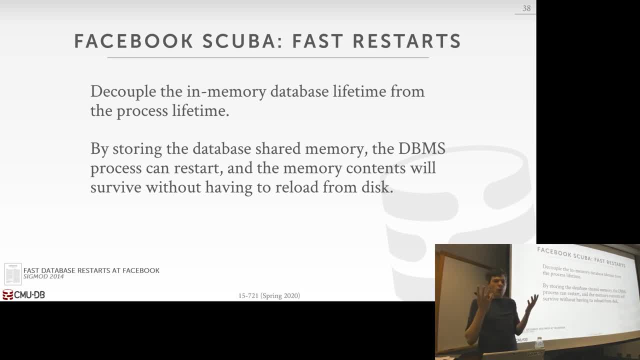 and say: find me the you know, explain to me why my page requests went 20% slower than yesterday. right? And because they're pushing out updates all the time for their web apps, they wanna know whether things are regressing. 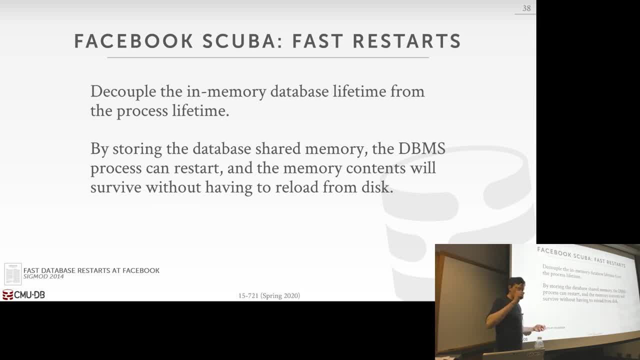 So what they're gonna do, though, is that, when they wanna update the database system software, that instead of. So what they're gonna do, though, is that, when they wanna update the database system software that, instead of shutting it down and taking Checkpoint. 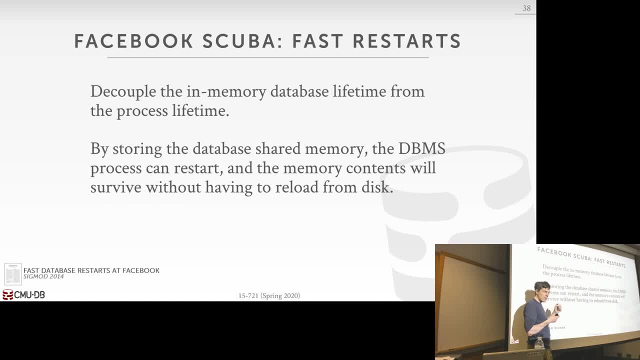 and loading it all back in. they're gonna write out the contents of the database, essentially the Checkpoint to shared memory, restart the process, come back up, see that my database state is now in shared memory and suck it all back in. 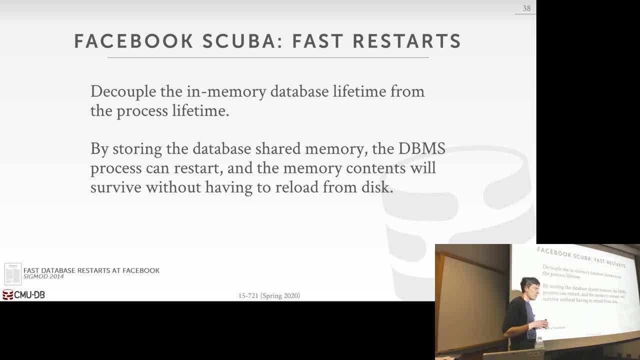 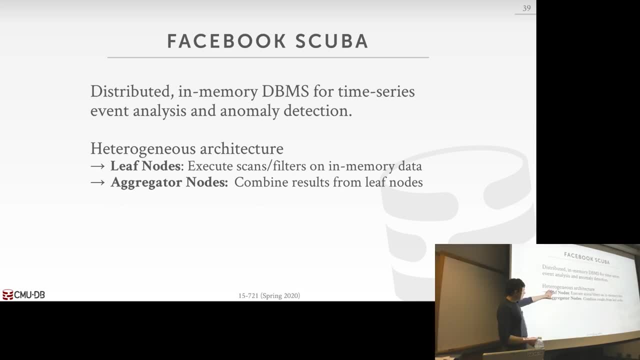 They're essentially using shared memory as like a RAM disk, which is kind of interesting. So again, I've already said this, it's a distributed in-memory system. It has a heterogeneous architecture with leaf nodes and aggregator nodes. This is not too interesting for us. 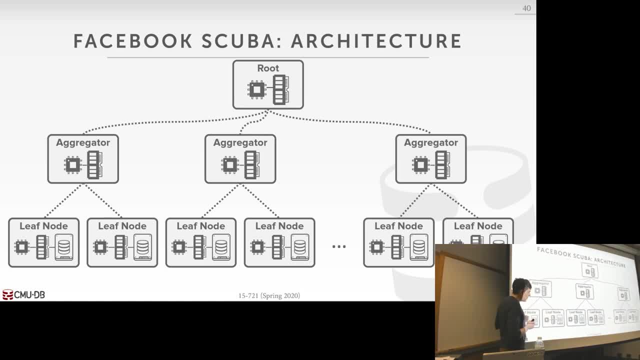 but just the thing to be mindful of is the state of the database is only at these leaf nodes here right, The aggregator nodes and the root node up above these are stateless and there's combining results of queries that these guys are they generate. 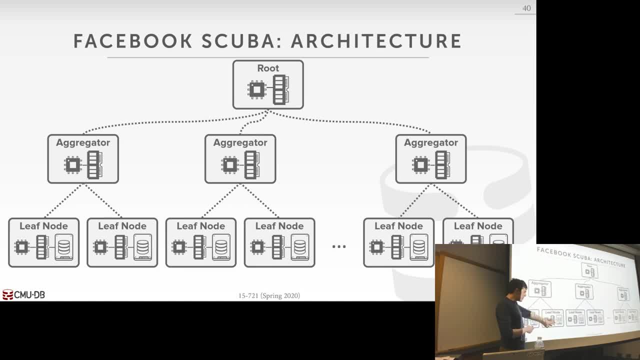 So all the updates of inserting new data goes to these leaf nodes, so this is the primary storage location. So if we wanna restart these guys, we need a way to again try to use up the shared memory so we don't have to load the Checkpoint from disk. 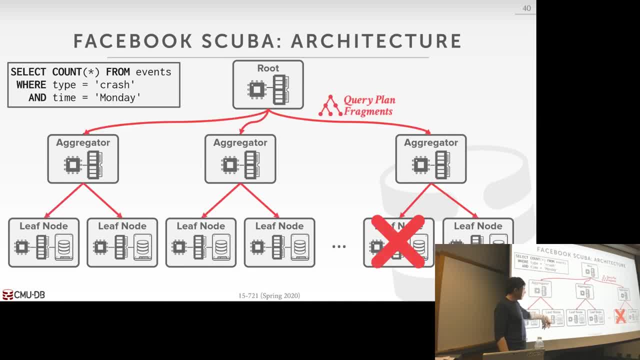 As a high level. the way it works is that if I have a query like this, they're gonna break up into plan fragments and say: this guy goes down, these guys are all gonna send their updates up and then we just combine it together. 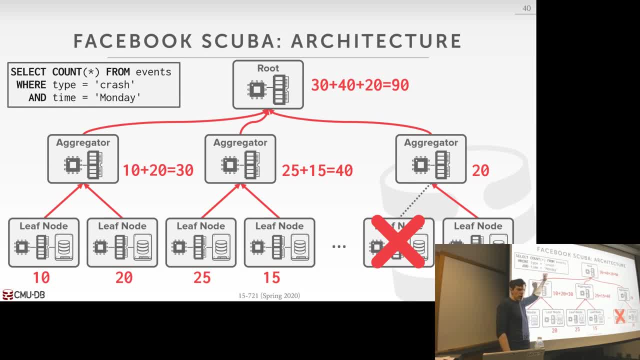 to produce the final answer. This is actually basically how MemSQL works out. well, right, Because the story goes. the guy that founded MemSQL- he was at Microsoft- saw the Hecaton project borrowed some of their. I was inspired by their ideas. 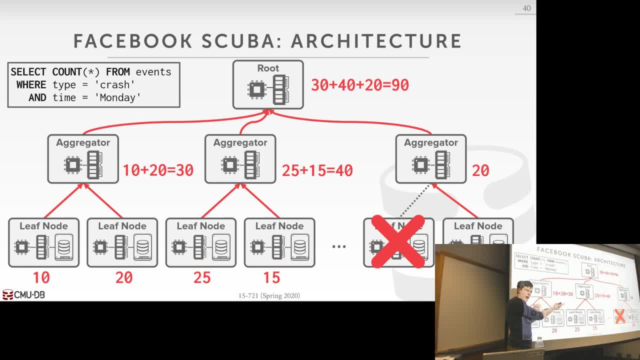 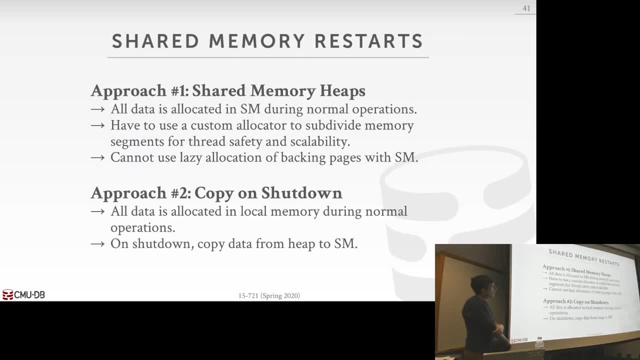 went to Facebook- I don't think he saw Scuba, but he saw this pattern used in other systems at Facebook- saw this idea and then combined it together to make MemSQL All right. So there's two approaches to do this. 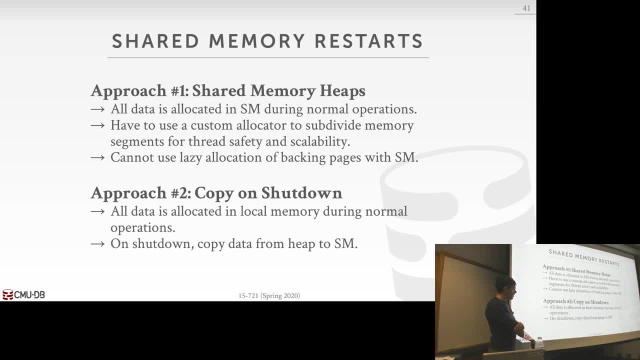 So the we've already said this- we could just do the shared memory heaps so that we could just, in our system, we modify the memory allocator so that whenever we call malloc for the data we're storing in the table instead of being local to my process. 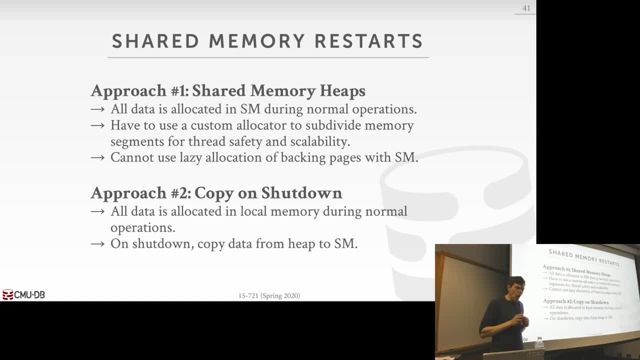 now it's sitting in shared memory. As far as I know, there's no overhead in the OS of saying something's in shared memory, because it's just getting back a memory address and the OS knows that it should. that memory should last beyond the process- lifetime. 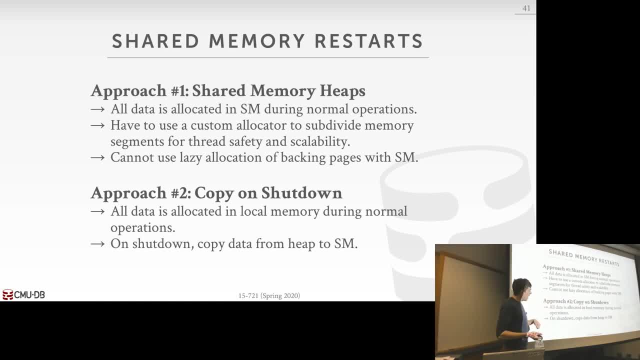 So to do this, though, again, you have to modify jmalloc or tcmalloc or whatever malloc implementation you're using to be able to write things out to shared memory and be able to divide things up efficiently so that multiple threads can be writing. 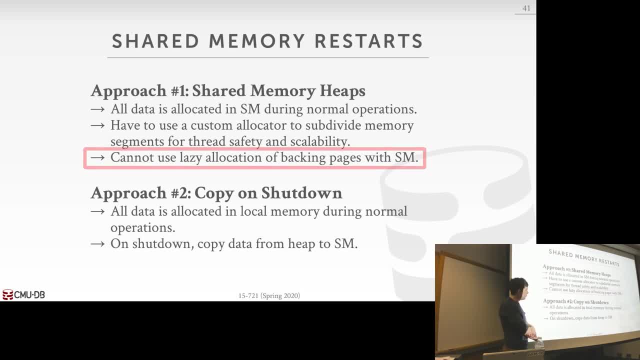 to the same location. So in the paper they talk about how they can't do lazy allocation of backing pages and shared memory, meaning if I call malloc on something in shared memory, the OS is actually going to need to have that backed by physical memory. 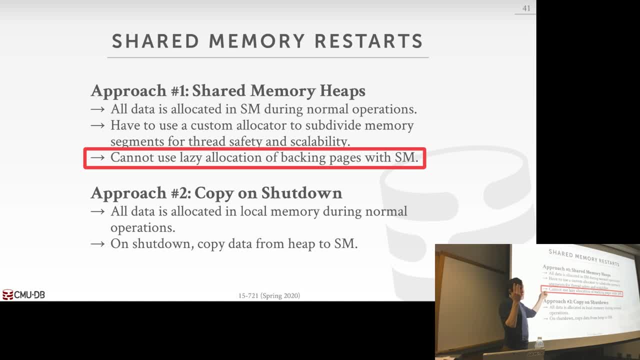 So they claim this is in the paper. They Facebook bought the guy or they hired the guy that created jmalloc. So in the paper they talk about how they talked to the jmalloc guy and he says: you can't do this. 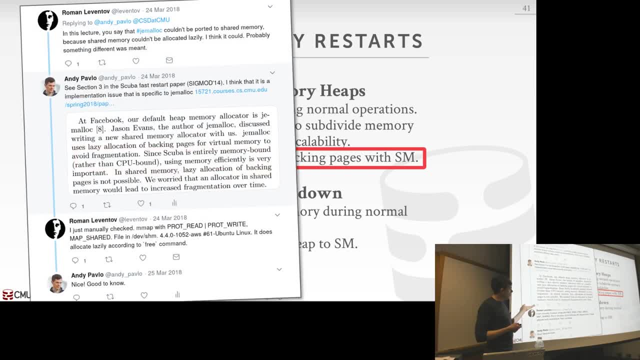 I posted this on Twitter, or at least the slides for this- on Twitter, and then some dude reached out to me and said: you actually could do this, like he actually tried it, and at least in the newer versions of Linux, that you could allocate memory in shared memory. 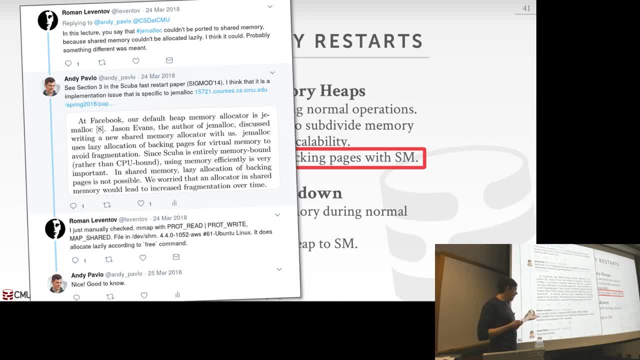 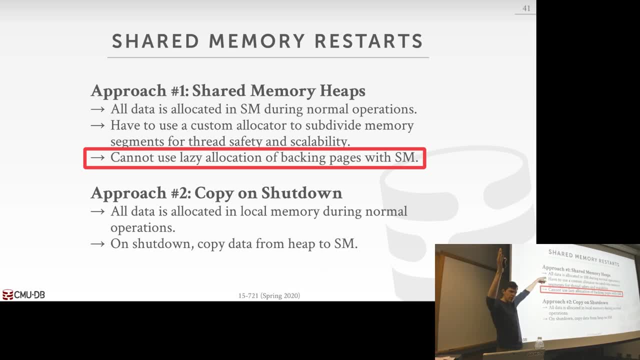 and not have it backed by physical memory right away. This part is actually not true anymore, So you actually could still do it this way, So you could have your memory allocator allocate pages on the heap in shared memory and not worry about any thread safety issues or backing it right away. 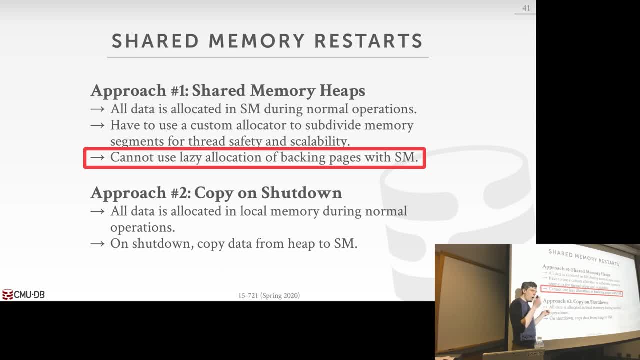 But instead, what they're gonna do in this version of Scuba is that when I'm told my process is going to shut down, I stop all updates from any transactions, any queries, write everything out to shared memory and then I can go ahead and restart. 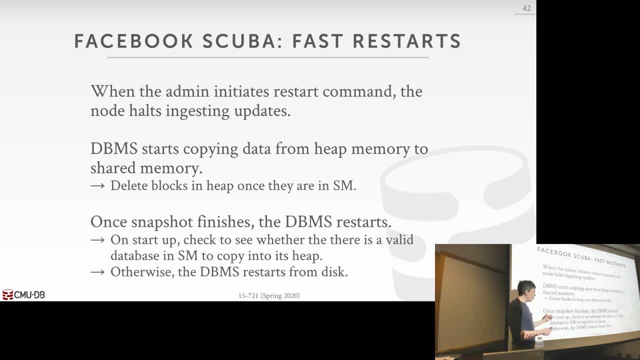 And so they do some extra stuff, that where they keep track of what's the layout of that memory that they're running out to shared memory, like what's the version of the database, and they wrote it out so that if you restart and come back and you recognize. 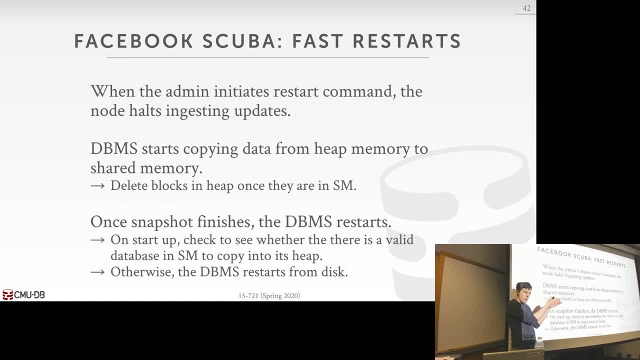 oh, I have some shared memory contents of the database from what it was before I've restarted. then you make sure that the layout is still correct. So they basically maintain some extra metadata when they run out to shared memory to say: oh, by the way, my layout looks like this: 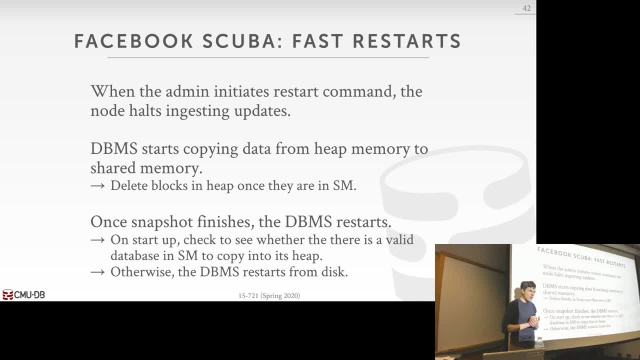 because I'm on this version, So if I come back and it's incompatible, then I just load it back up from disk. So Scuba's an interesting system, because in their world this is not high value data. right, It's not like your timeline or all your. 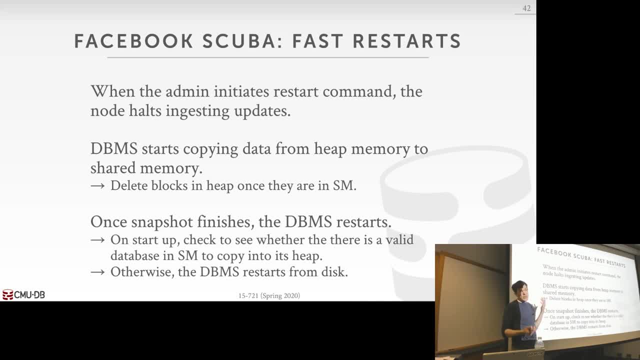 whatever your friend messaging crap Like it's data that they could potentially lose. They don't want to, but it's not like they lose money if this goes away. So ideally if they say a node comes back and there's nothing on disk, 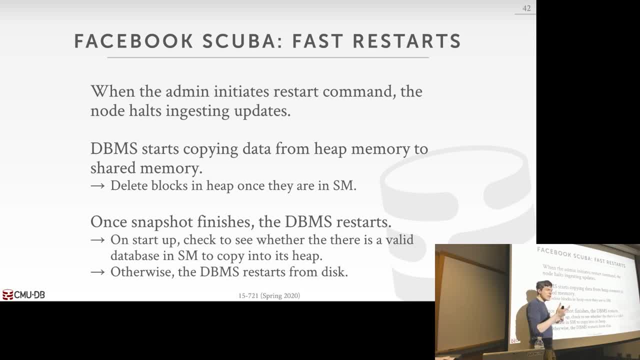 but the shared memory, sorry, the database system comes back. there's nothing on disk, everything's in shared memory. but the shared memory data is not compatible with our new version of our software. then they'll just backfill it from you know. 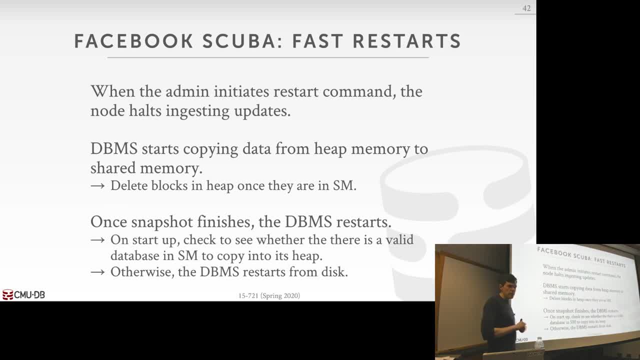 from another disk from somewhere else In their world. that's okay, So I like this idea. I don't know if anybody else does this with shared memory. The most famous shared memory system is Postgres, but they're obviously not in memory. 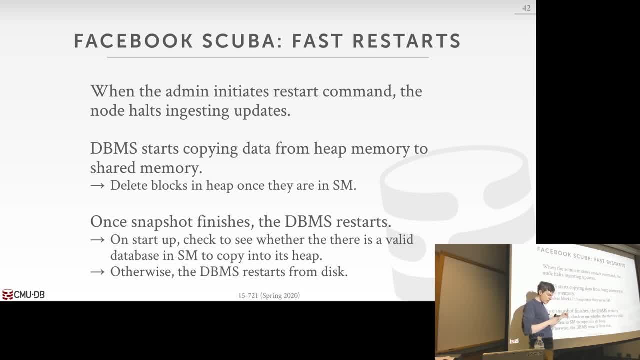 And they're doing this to coordinate across different processes. This is like this is now. this is an interesting idea to think about, because it's passing data from one instance of the process to the next, even though they don't actually overlap in time. 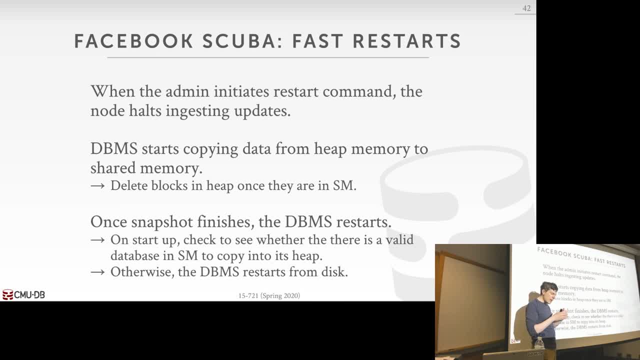 They're allowing the memory of the of the database go beyond the lifetime of the data system process itself, which I find super fascinating. Any questions about this? Again, if my database is one terabyte, if I don't have this technique and I restart the database, 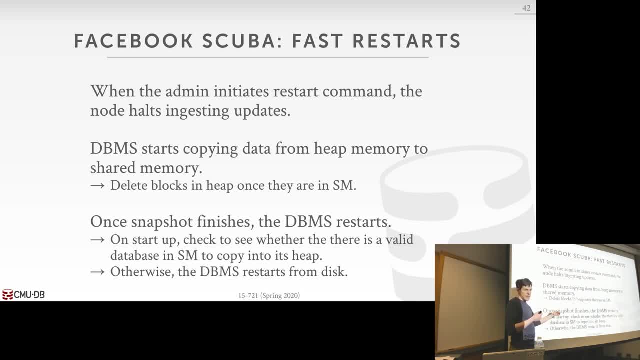 then I gotta suck in one terabyte off a disk, which could be slow, But in this case here I could come back and instantaneously have everything that I need. Okay, All right, so just to finish up, The main takeaways from this is that physical logging, 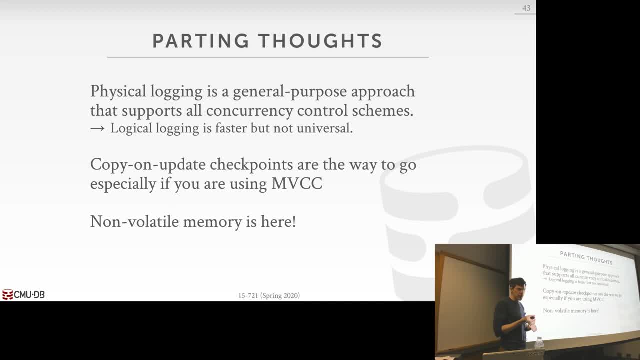 is probably the best approach you would wanna use for an in-memory database and it's gonna support all possible conceptual schemes. There are some advantages we can take, or things we can take advantage of if we're using MVCC, like doing the copy on updates to get consistent checkpoints. 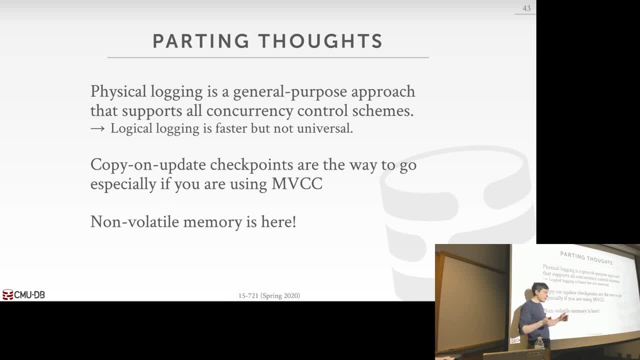 by just relying on the idea of snapshot isolation to only see changes from transactions that have already committed. And, as I'll talk about at the end of the semester, non-volatile memory is here. It is gonna change how we wanna do some of these logging, checkpoint protocols. 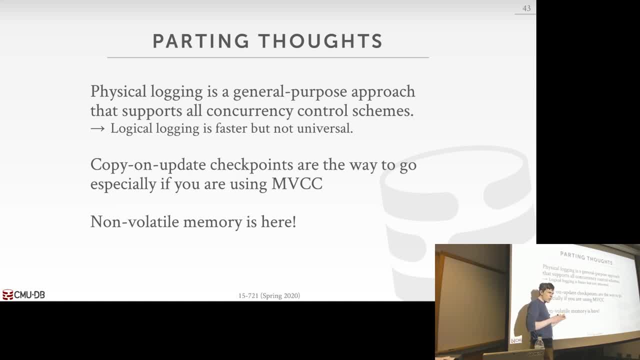 but the high-level idea will still roughly be the same: that we don't need to maybe restore or don't need to log any undue information. If we're careful about where we store our data, then we only need to keep track of redo information. 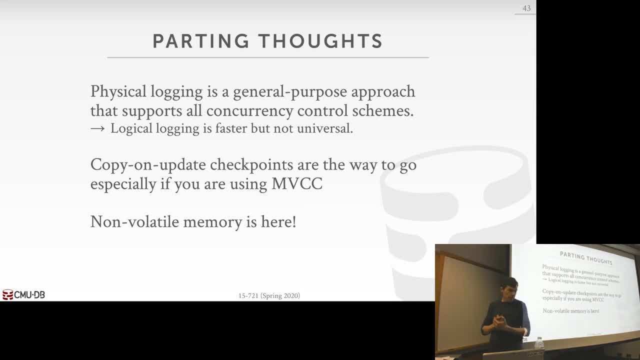 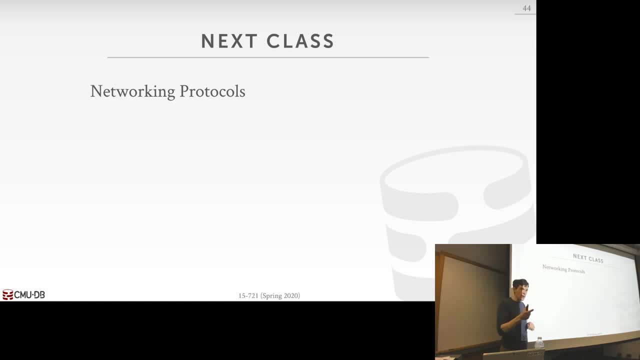 and that makes the log replay much faster. Okay, All right. so next class we'll talk about networking protocols and I don't have it listed here, but we'll also introduce project two. This is on Piazza You guys should start thinking about. 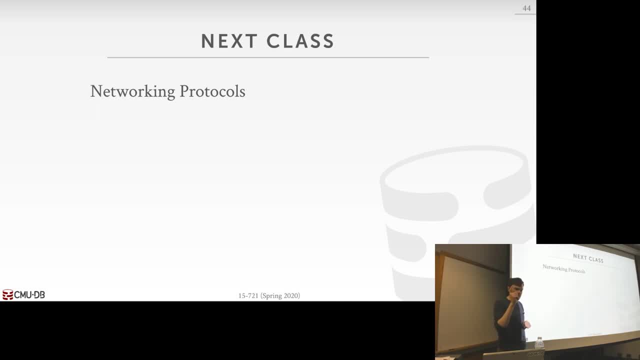 how to form groups of three, because project two will be a group project. okay, If you can't find a group to be in, send me an email and we'll figure out something for you. Okay, I forget how many students are in the class. 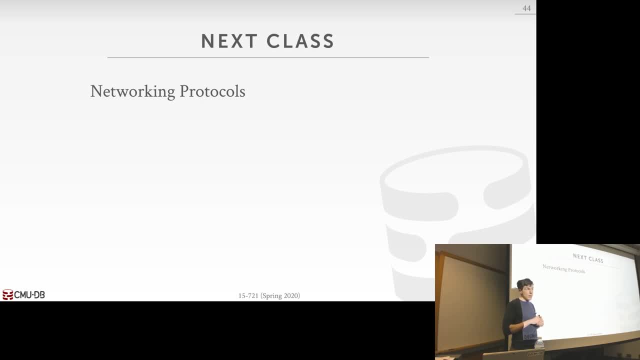 I don't think many people are dropped, so we should have enough to do exactly three, I think, 13 groups of three or something like that. Okay, Yes, So right now it is like this, that there are six, seven groups. 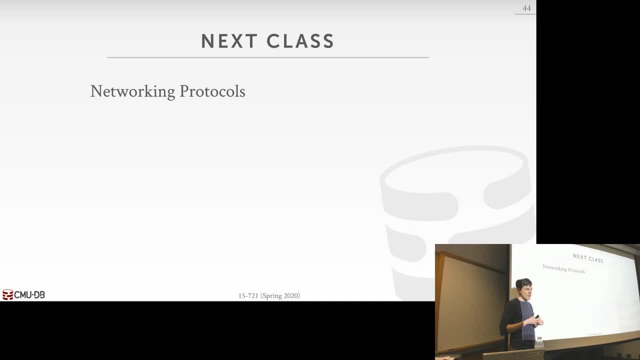 All of them are of two people. Has to be three, Okay, So make friends. And again, whoever's in your group for project three- sorry, project two- will also be in the same group for project three. So if someone is like an. 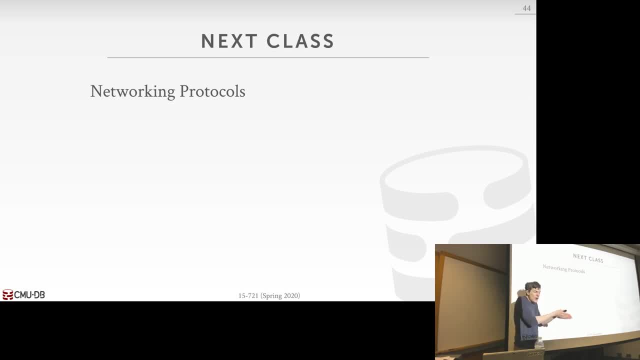 has hygiene problems. if you can't stand around project two, then you have to deal with them in project three and that's not gonna be good. Okay, And if I have to break up fights, I've done it before and I can do it again. 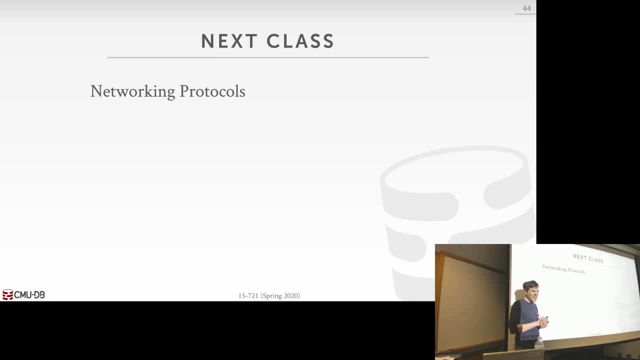 I really don't want to do this. Okay, Any questions. Bank it in the side pocket. What is this? Someone push. Hey, yo, it's me. I don't want to do this. I don't want to do this. 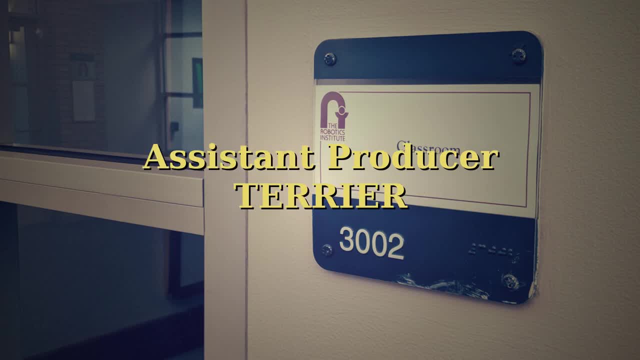 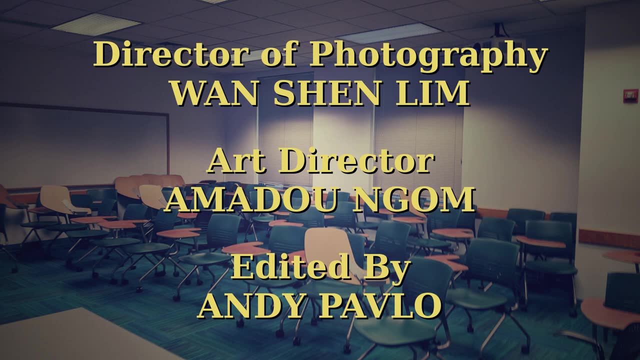 Okay What? Took a sip and had to spit, cause I ain't quit that beer called the OE, cause I'm OG. ice cube down with the STI. You look, then it was gone. Grab me a 40 just to get my buzz on. 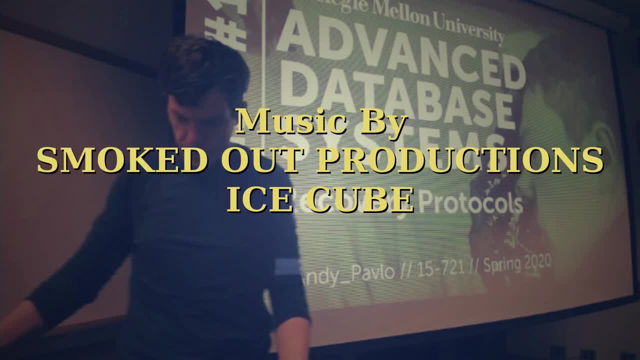 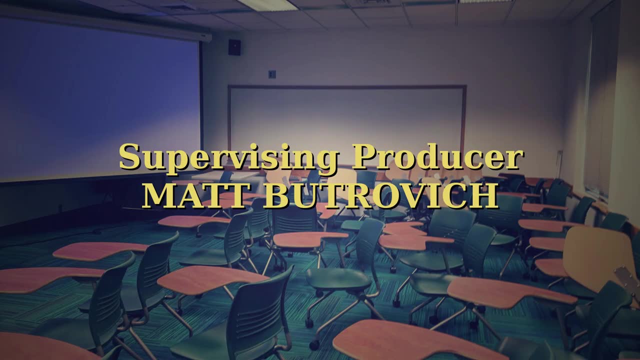 cause I needed just a little more kick. Look like a fish after just one sip, Put it to my lips and rip the top off. They just dropped off Cause St I's hopped off and my hood won't be the same after ice cube. take a St I to the brain. I don't want to do this. 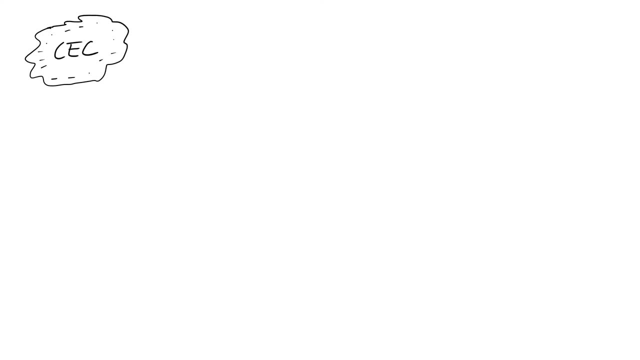 So today we have yet another video looking at the cation exchange capacity and we want to move towards looking at cation exchange capacity as it relates to changes in soil pH and therefore changes in soil acidity and alkalinity. So we know that the clay, mineral and organic matter components of soil tend to have negatively charged sites on their surfaces which adsorb and weakly hold positively charged cations. 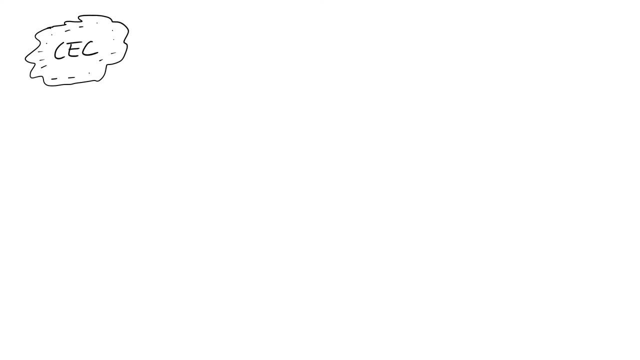 Now, the electrical charge is critical to the supply of nutrients, because it's one of the ways that nutrients are retained in soils. So we could say that, in general terms, soils with a large cation exchange capacity tend to be more fertile because they retain